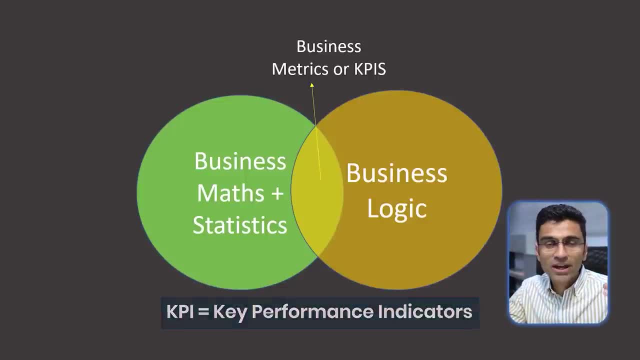 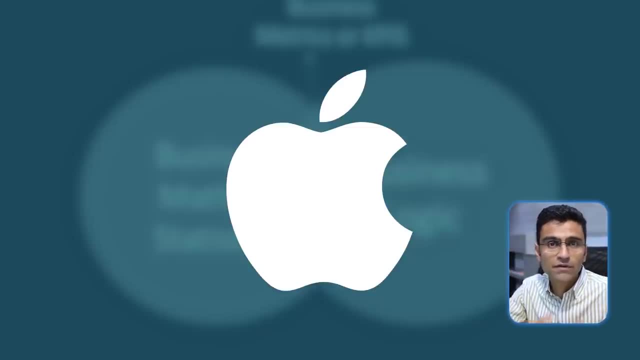 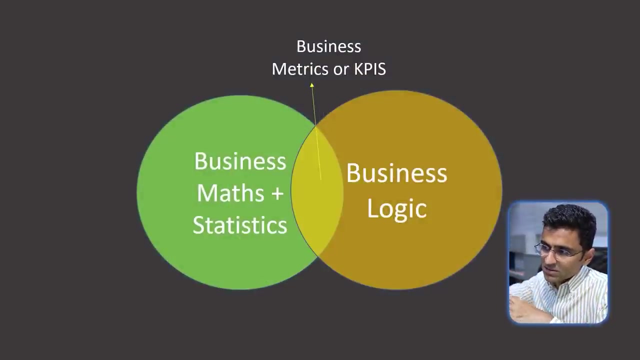 revenue, profit. you know if you're looking at apple, how many iphone they sold last year. what are my top five products? who are my top five customers if you are in a service industry? so these are all called kpis, or business metrics, and it is an intersection of business math. 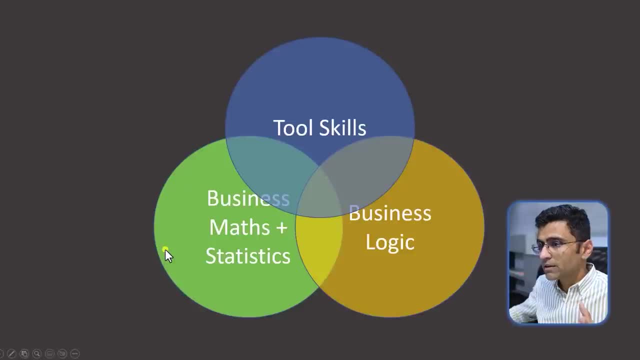 statistics and business logic. now, if you add a third dimension to it, which is a tool, skills, because, see, to do data analysis or business logic and business math is not enough. you need to know some tools such as excel, python, r, power, bi, and the intersection of this is basically your data. 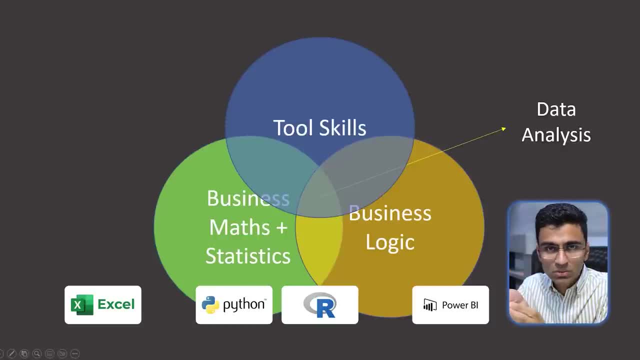 analysis. in order to do data analysis, you need some tool, which could be excel, python, etc. but just by learning tool skill, you're not going to do data analysis. this is the classical mistake that people do. when i'm talking to any data aspirant, i ask this question: in last one month, how much time you have? 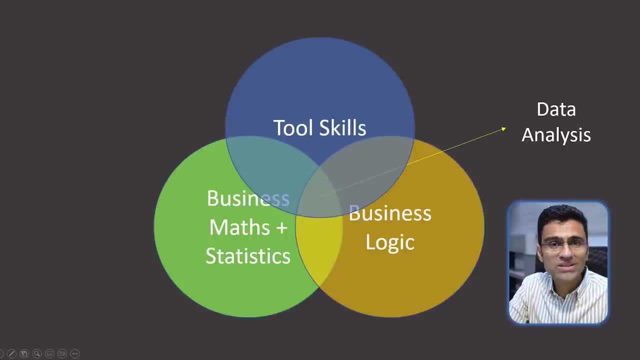 spent in business logic or core skills such as communication, presentation, and usually the answer is close to zero. people focus so much on tool, but this diagram will make you realize the real data analysis can happen if you have right combination of these three skills, and in this video series. 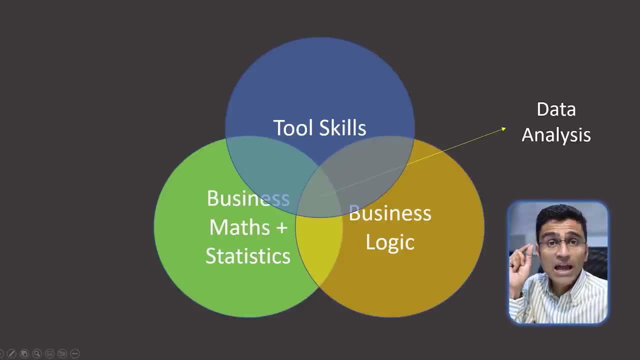 you will find a playlist link in the video description below. I am going to be teaching you all these three skills using very, very simple examples, so that even a dumb person should be able to understand these things easily. as far as the tool is concerned, we are going to use Microsoft. 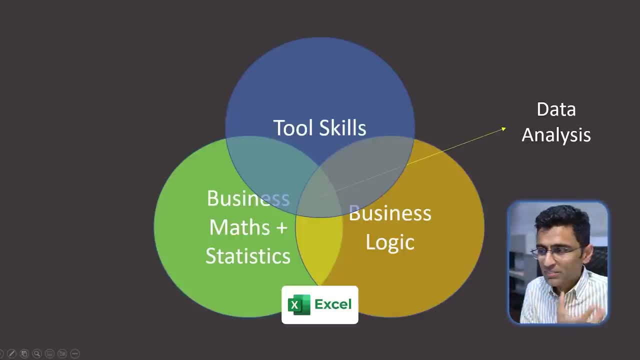 Excel because that is the number one tool that people use when they are performing data analysis, especially on smaller data set. so, believe it or not, Microsoft Excel is truly the strong cornerstone of this whole world, still very, very widely used, and that is the reason i have created microsoft excel course. 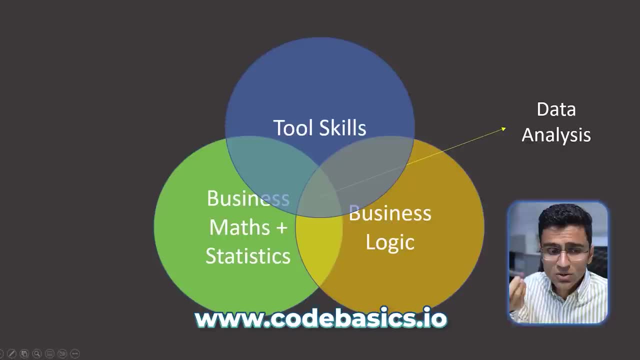 which will be available on my website, codebasicsio, in march 2023, so check the description below. you might find a course link there once it is launched and that course will contain a lot of premium material, but i have taken some of the material from that course and designed this. 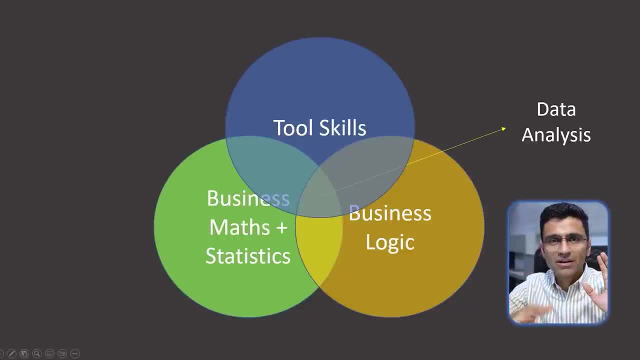 entire playlist. so this playlist will have, let's say, 10 percent or 5 percent of the content from my premium excel course. okay now, since we are using excel as a tool skill, in the next video we are going to look at some excel basics. you might know some excel already, but i'm just going to quickly. 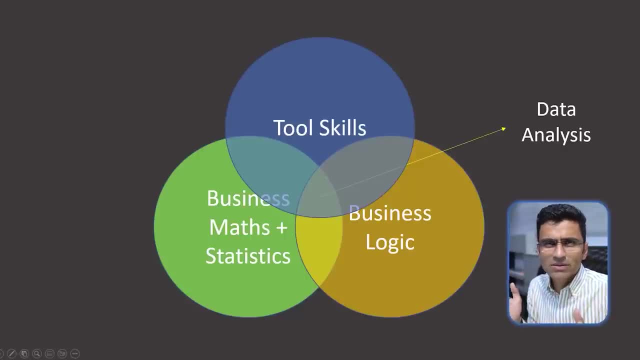 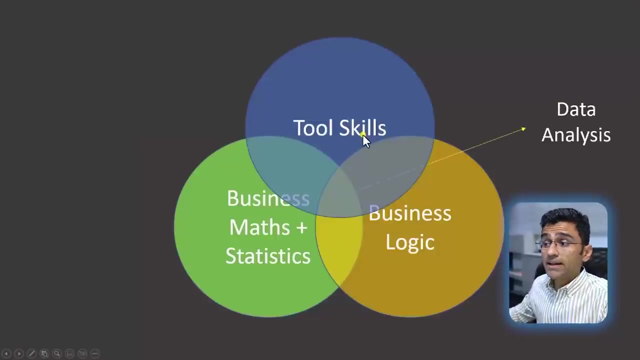 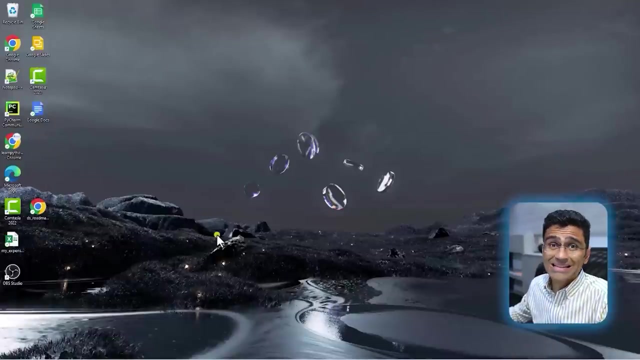 cover some of the very, very basic things in excel and few advanced things as well, and then we will start performing some business related data analysis. in the last video, we said that as a tool we will be using microsoft excel for this entire series. therefore, i am going to be covering some excel basics in this video. i have windows machine where. 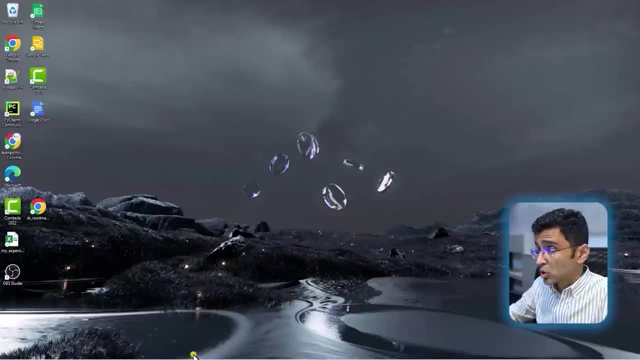 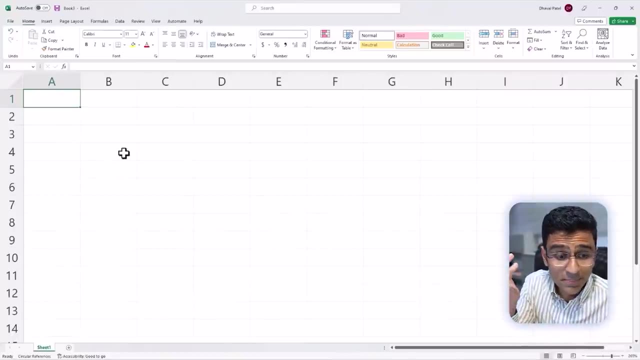 i have excel installed already, so i'm going to launch that application directly. if you don't have it, you can install it. it's a paid software. if you are a student, they give some discount. if your college has association with microsoft, you can also use the online version of microsoft excel. 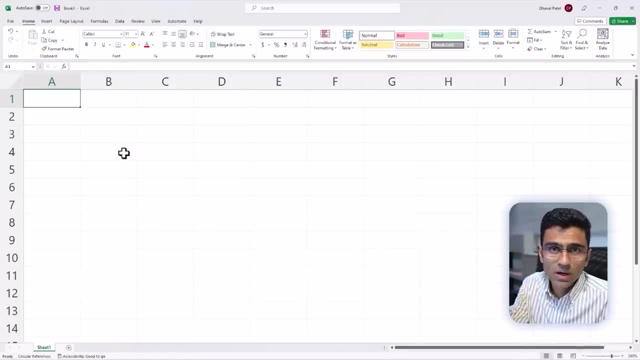 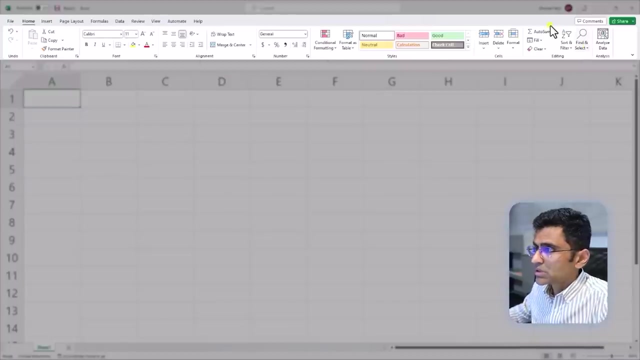 where the excel will run in the browser and that should work okay. but i will leave it up to you on how you want to install excel. let's say you have it installed when you launch it. let me go over this: the tool and the anatomy of the application. so at the top you see this manual. 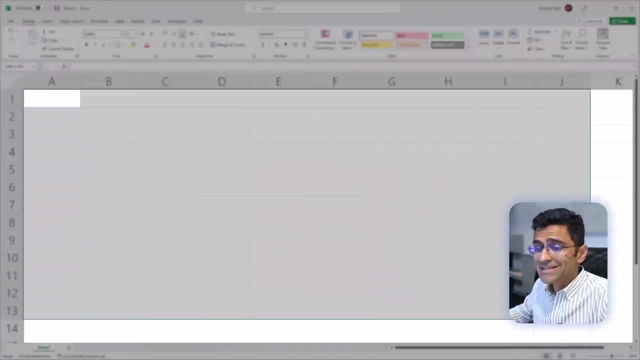 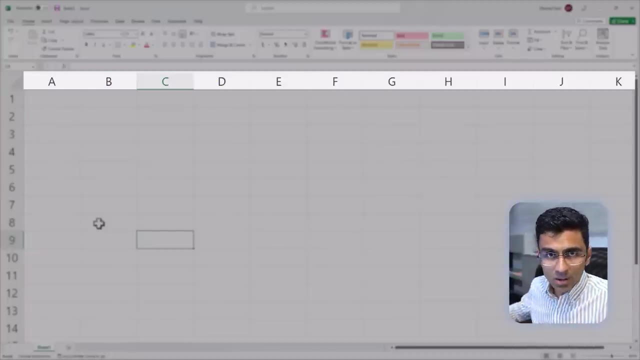 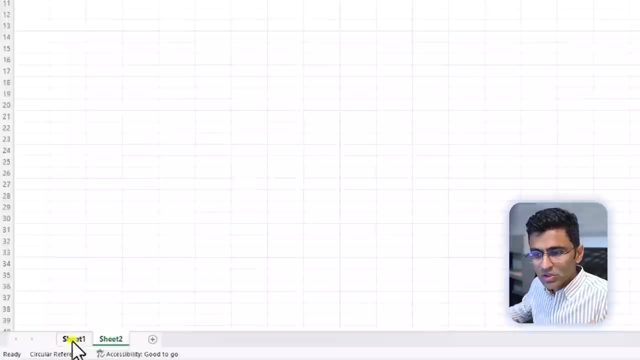 bar where you see variety of option here. what you are seeing is the spreadsheet, okay, and spreadsheet has rows and columns. so one, two, three, these are row numbers, ABC, these are columns, and at the bottom you have sheet, so you can have multiple sheets by the way. okay, so let's say you are trying to maintain your 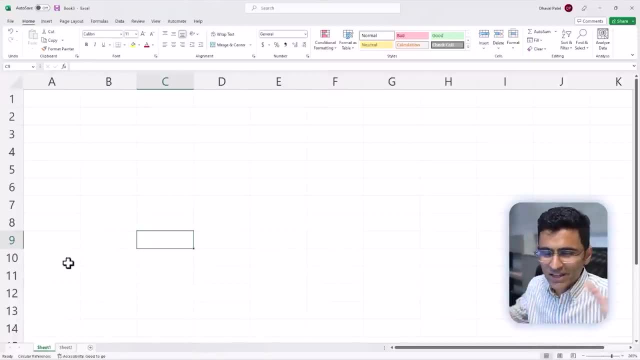 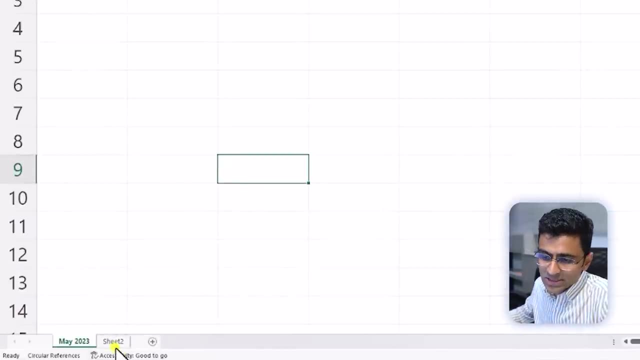 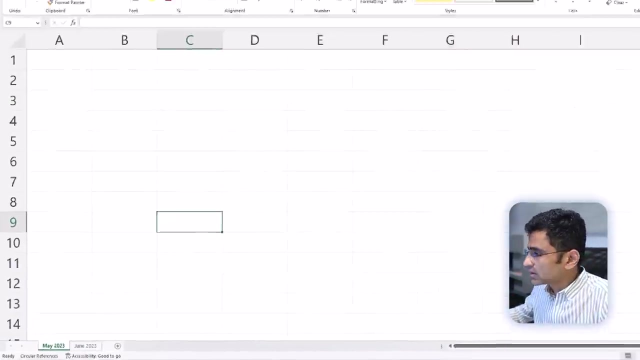 monthly home expenses in the excel file. that's a very, very first basic use case you should learn whenever you are learning Excel. and let's say I am maintaining those expenses month by month. so I will say May 2023, June 2023. for each month you can create a separate tab. when we started my company, atlick 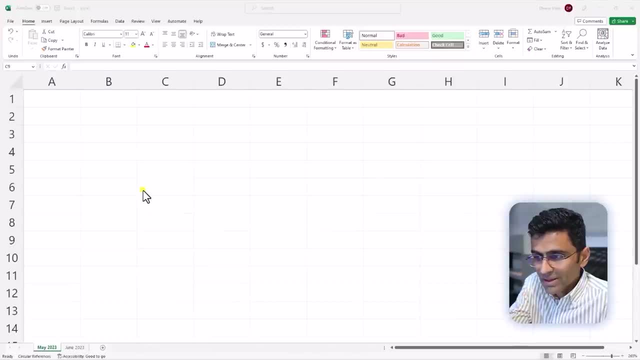 technologies, which is a software development company. we used to maintain all the expenses in this kind of sheet. you know month to month expenses for the company and here you can type in your expenses so you can see. here you can type in your expenses. so you can type in your expenses, so you can. 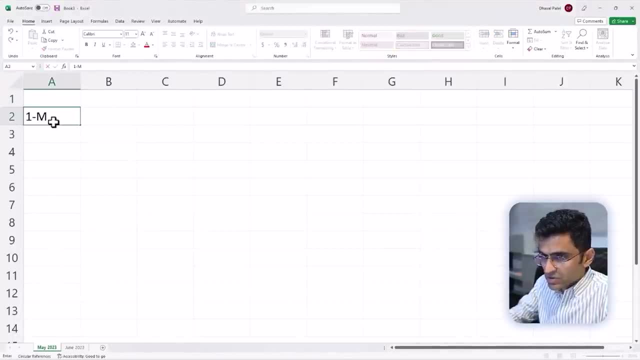 say: okay, first me on me, I spend on home rent. I spend, let's say, $500, okay. so this home rent is, let's say, an item and this is an amount. this is the category, because you're going to categorize your expenses, like rent and food and utilities. 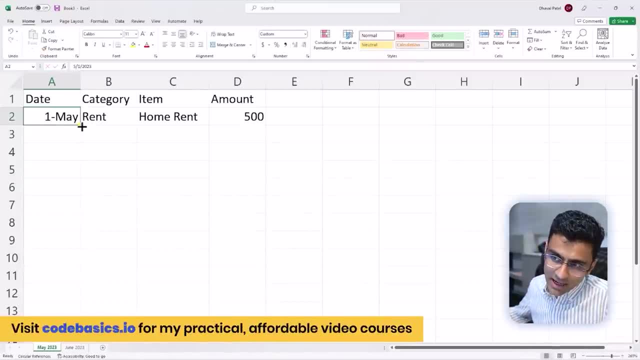 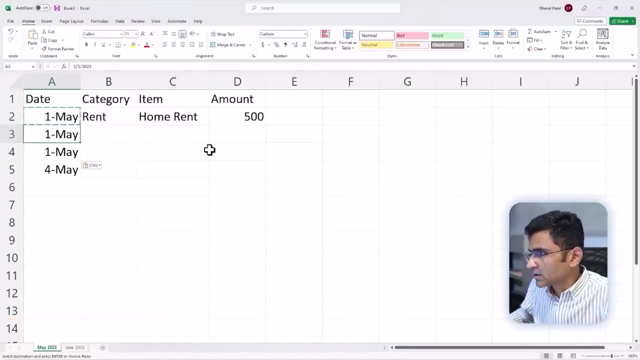 and so on, and in excel you can drag and drop it. when you drag and drop, excel is smarter and it will figure out that this is a date, so it will increase the date. okay, but let's say for first may itself i have a few expenses, so let's say i have. 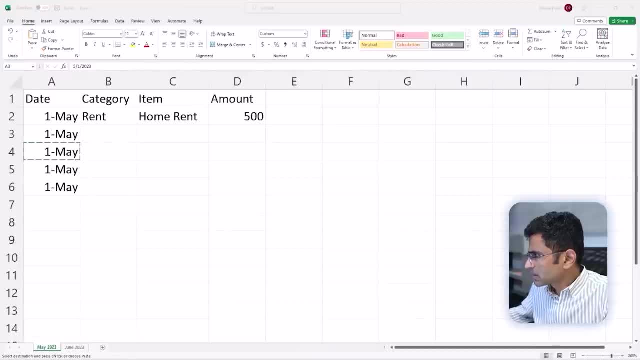 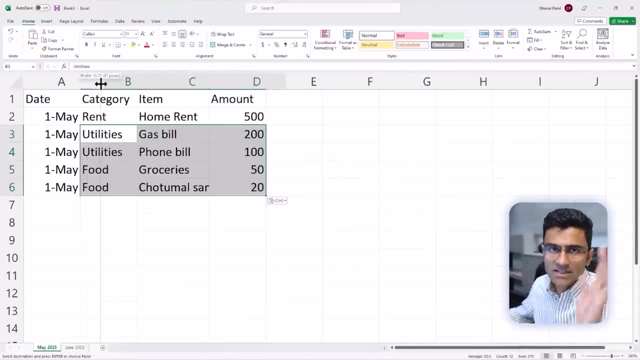 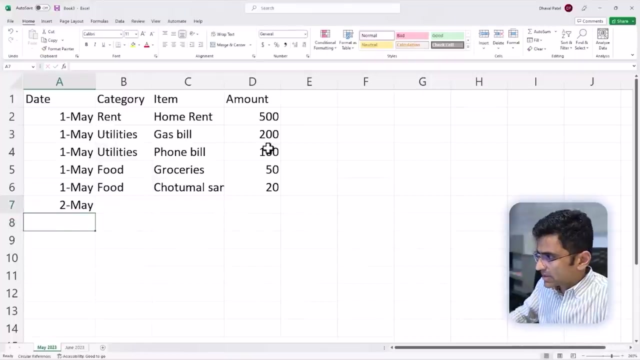 five expenses for first may, and those expenses i'm going to just copy paste to save my time. so for copy paste you can say ctrl c, ctrl v. i'm going to provide this excel file. check the video description down below, then you can have. okay, let's say this is my second may. for second may i: 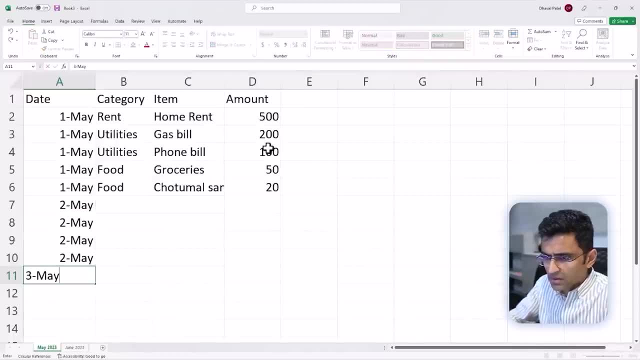 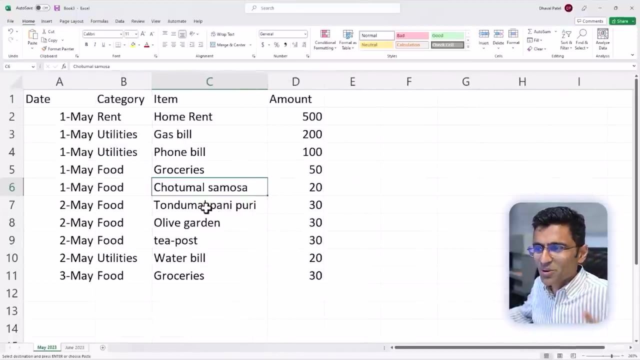 have once again four expenses. and third, may i have one expense? okay, so i have this other sheet and i'm just going to copy paste data so that it saves time on recording. okay, you love samosa, so there is a chotumal samosa shop nearby your home. there is a tondumal pani puri, so you are eating. 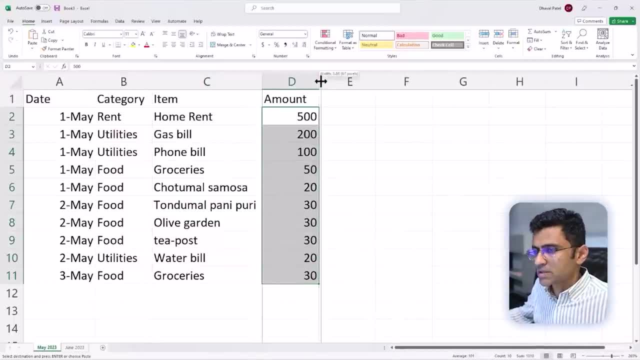 all of that and you're maintaining, you're maintaining, you're maintaining all your expenses here. okay, it is a common practice that the header you want to highlight in a special color so that you know it is a header, and then if you use b, it will make it bold. 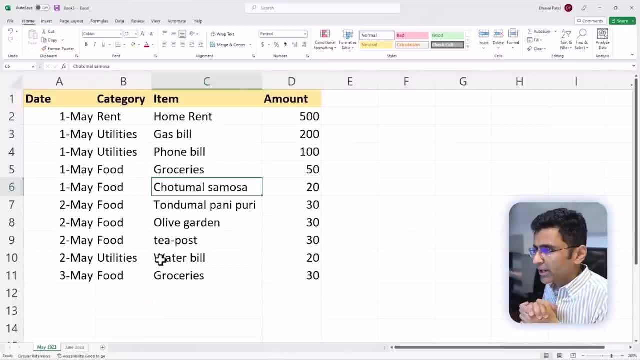 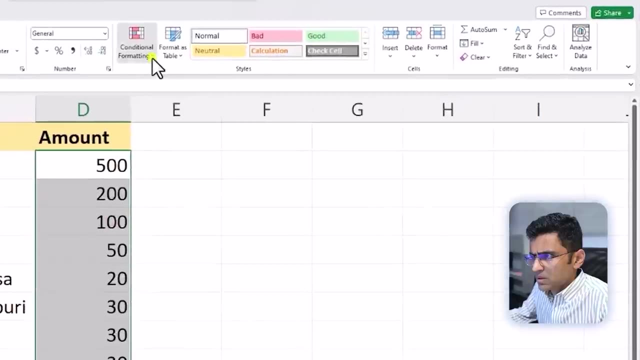 so now my expense sheet looks little prettier. all right, you can also use conditional formatting where, let's say, if the expense is more than 100, you want to highlight it. okay, so let's do this. you can select this column and you can say: highlight greater than so if this is greater than, let's say, a hundred dollar. 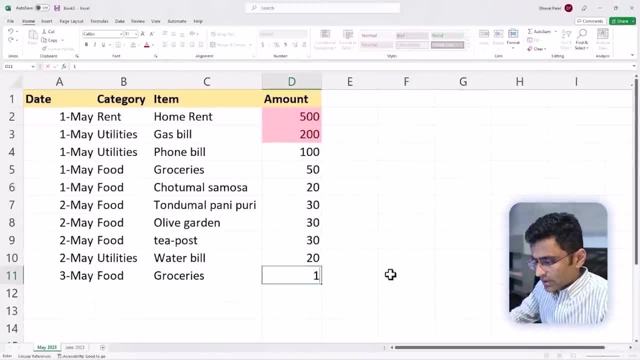 then i want to highlight it. so now what happens is, whenever your expense is more than some amount, it will highlight it. this kind of highlighting helps. as i said, i have worked in a industry for many years and when i used to deal with this big excel files, especially at my stay at bloomberg- 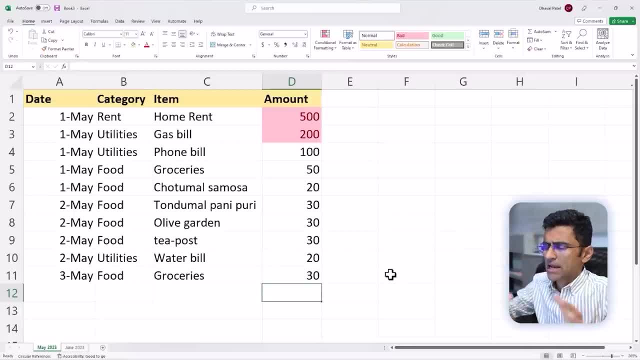 in new york office we used to get huge excel files and if you want to highlight this kind of highlighting, you have this kind of conditional formatting that will always help. you have some data point which are extreme or which are which are creating some kind of trigger. you can highlight those with certain. 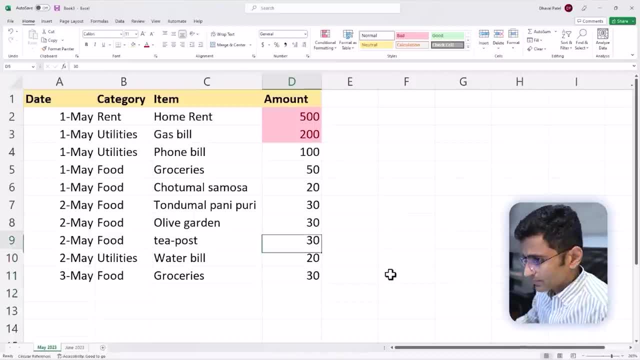 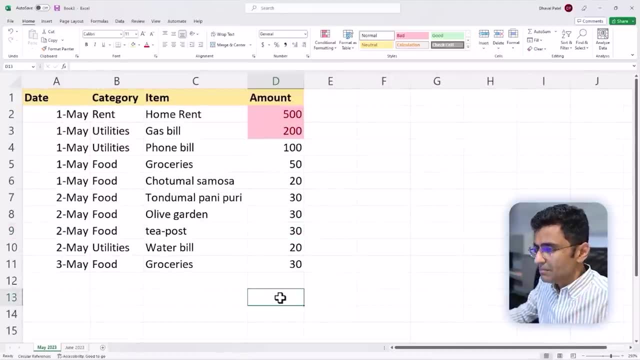 numbers so that you can quickly look at them and do your analysis. okay, now let me show you some basic formulas in excel. okay, so let's say you have all these expenses. naturally, the first operation you might want to do is you want to know your total expense. 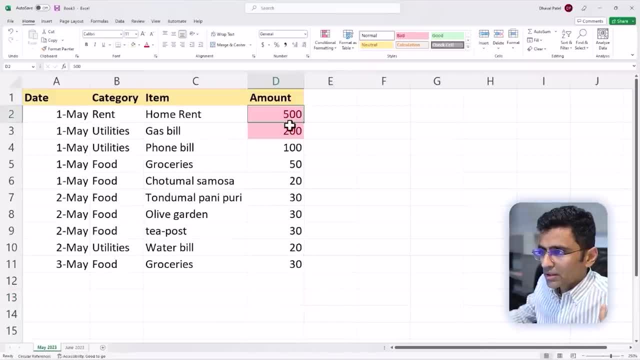 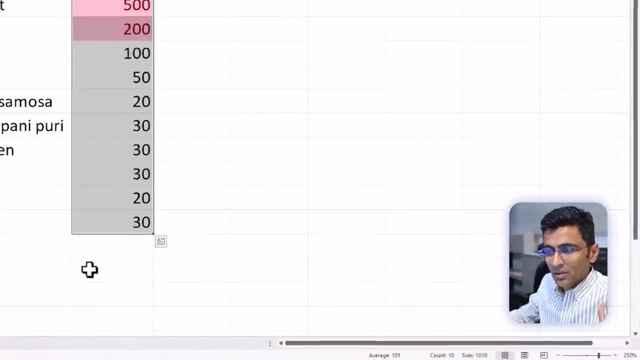 how much i spent in total in month of may. you can do that by just highlighting left mouse click, click here, and at the bottom it will show you the sum 10, 10. or you can type in a formula and for formula what you need to do is you you can just say: is equal to. 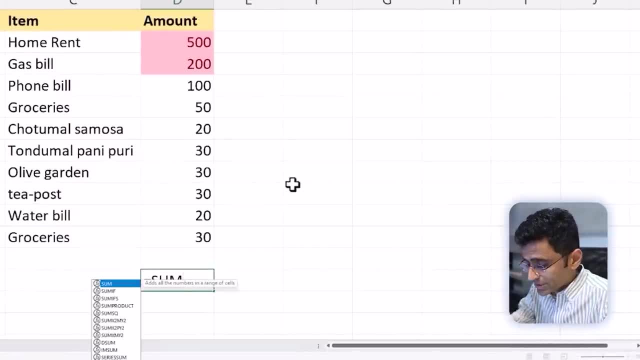 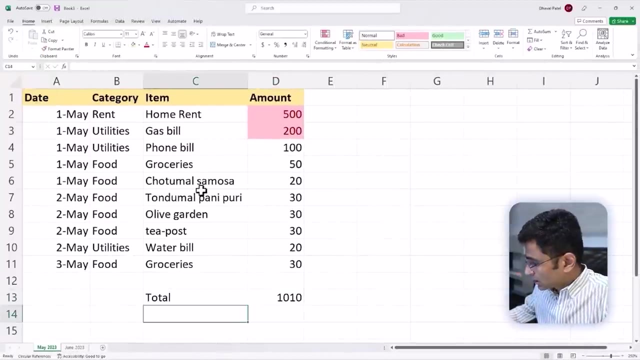 sum. so sum is the formula. so it is showing you in autocomplete. you open a bracket and then left mouse click you highlight all this cell. you can type this thing manually also: d2, colon, d11, bracket close and that shows you a sum. okay, so this is my total. you can control. scroll down to 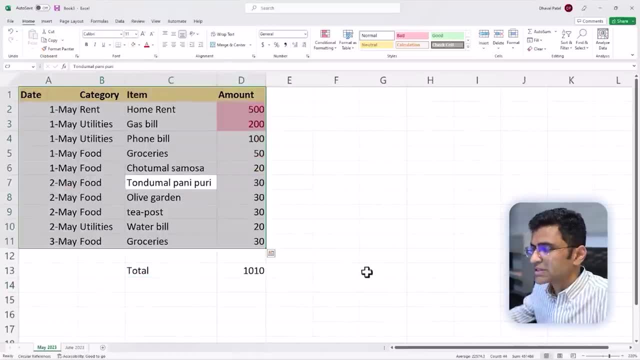 reduce the font size, or you can reduce the fonts. this is the, not the font size. this is really the view. okay, you can reduce font size from here. you can also do auto sum by using this particular, this particular option. okay, you can also sort the numbers by clicking any number here, and you can. 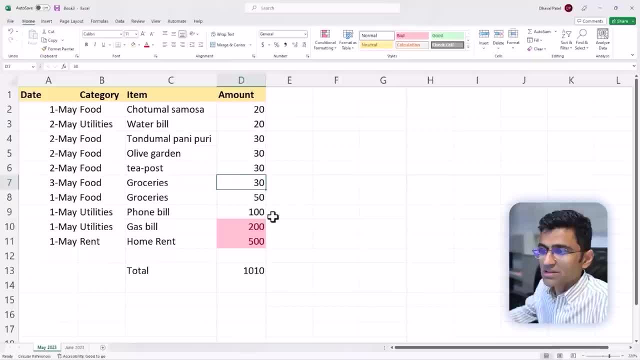 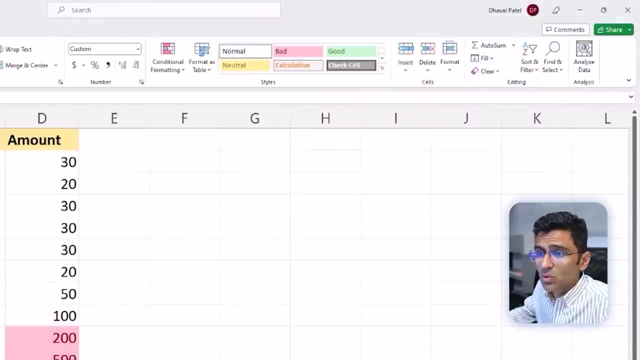 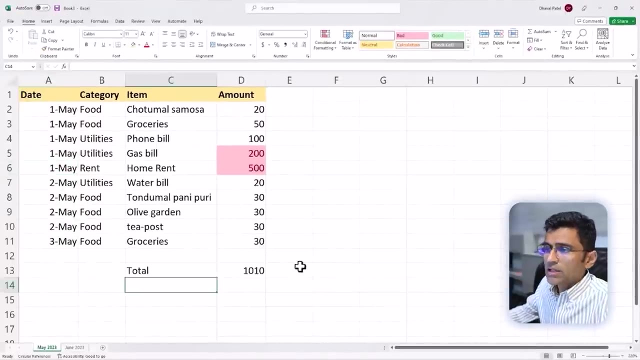 here, say, say smallest to largest, and see, it will sort it like that. but if you want to sort by dates, you click here and once again, you can say newest to oldest or oldest to newest, and it will sort things like that. all right. now each block, the square that you are seeing, is called. 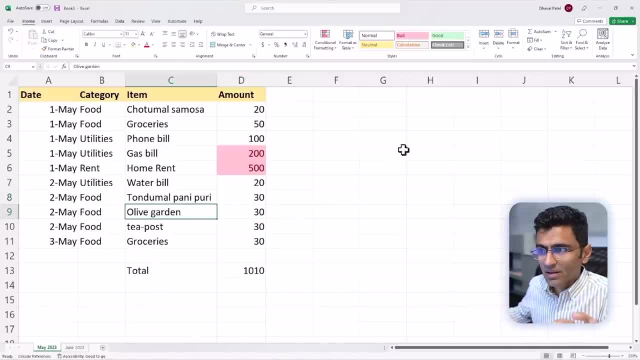 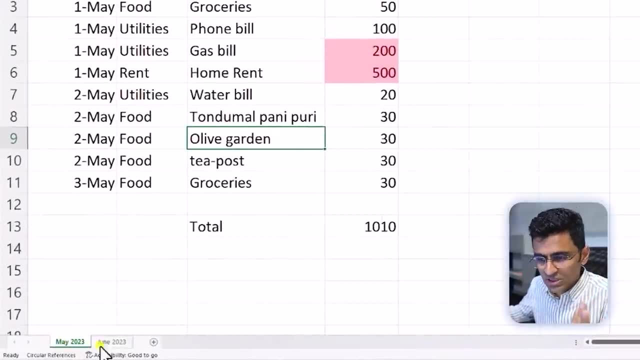 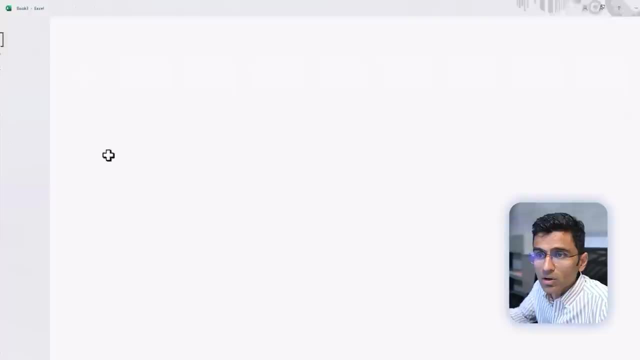 cell. so this thing is a cell, this thing is a cell, this whole thing is a spreadsheet and you can call it spreadsheet or sheet. so sheet one, sheet two, you can rename it, and this whole thing, the whole file that you're seeing, is called workbook. so the file you can save by 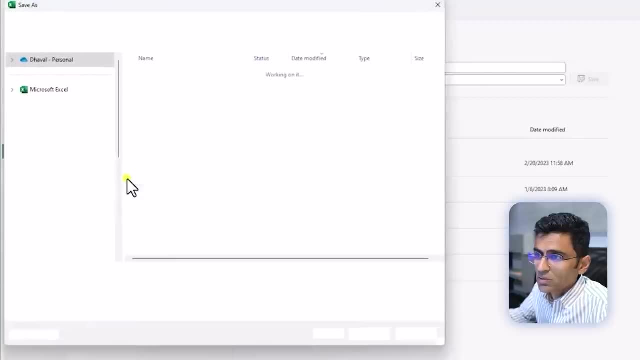 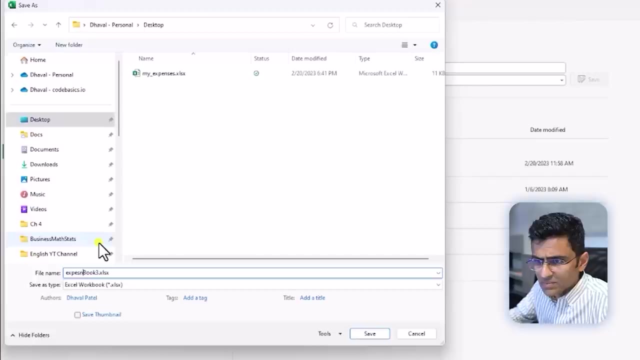 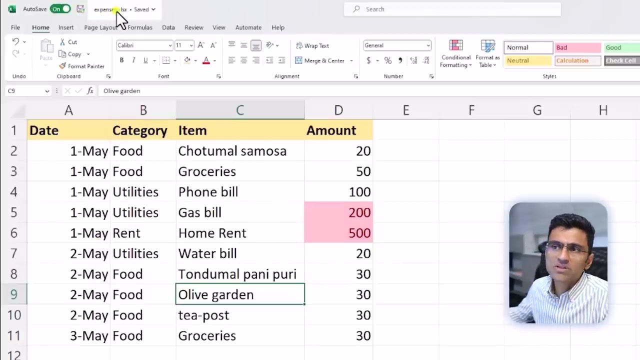 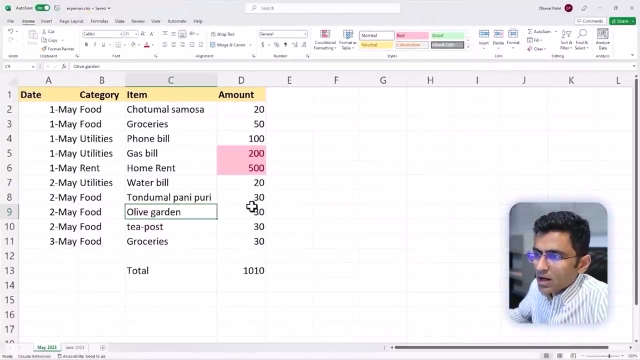 saying this: save, okay, so you can save to, let's say, this pc. i want to save it on desktop. i want to call it expenses, expenses, okay, so. So expensesxlsx is the extension for excel file. Now, when you have numbers, you can do formatting. let's say, this amount is in dollar, so if you 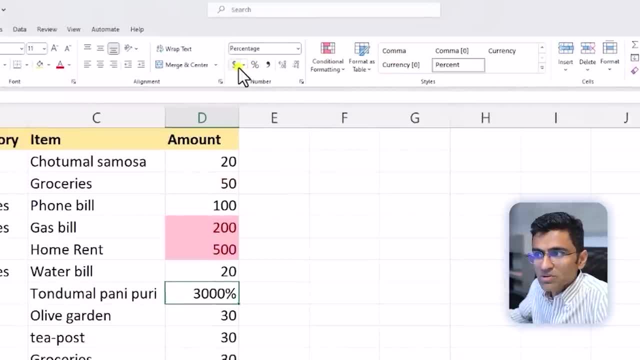 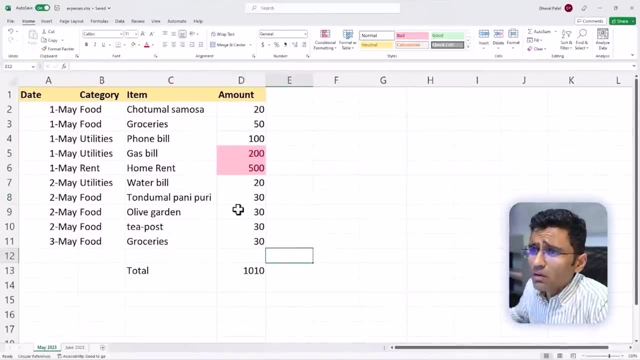 click on it, see, it will show it as a dollar Percentage also. you can do, but I don't want to have any formatting here, so I will just say general, which is no formatting. One other operation you might be interested in doing is you have this: categories. 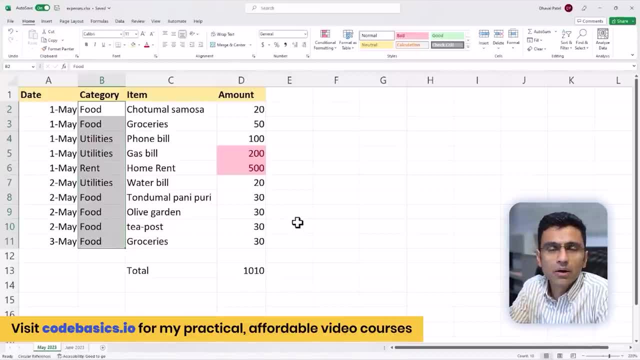 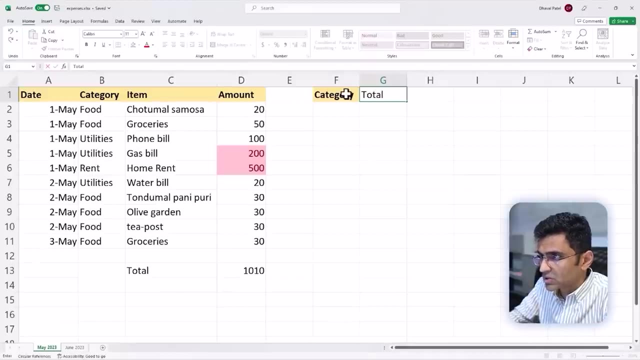 I want to know the total expense per category on food in the month of May, how much money I spent on utilities, how much money I spent. So you can here create another kind of a table where you will say category and total. in category you have food, utilities etc. 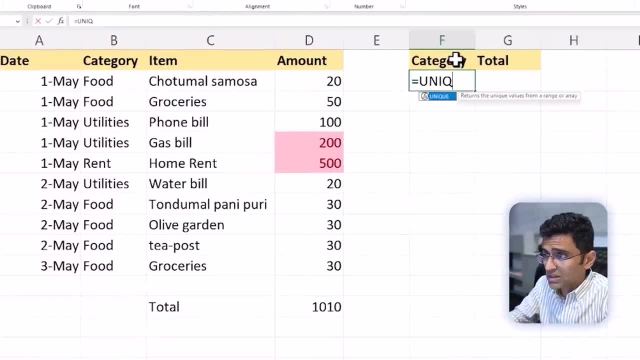 Now, if you don't want to write all of this, you can use unique formula so you can say equal to unique and in the unique, So see food utilities, rent. and if you want to sum them, see, I can use sum. I can use sum. correct, but that's a total sum. I want to sum only food items. for that there is a function. 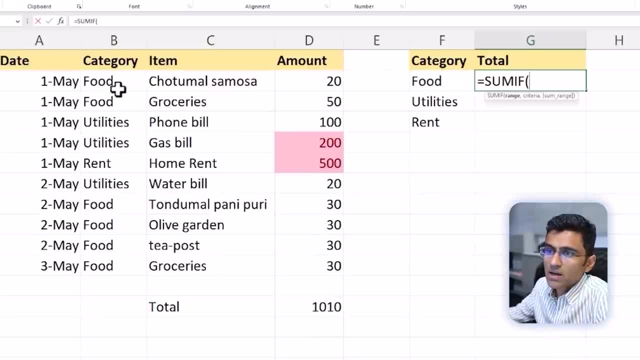 called sumif. so in sumif you will specify on which category you want to do that grouping. so you first specify the category column. then you want to say: I want to filter only food. okay, food comma. how do you want to sum? so this is my sum range. so in this range I want: 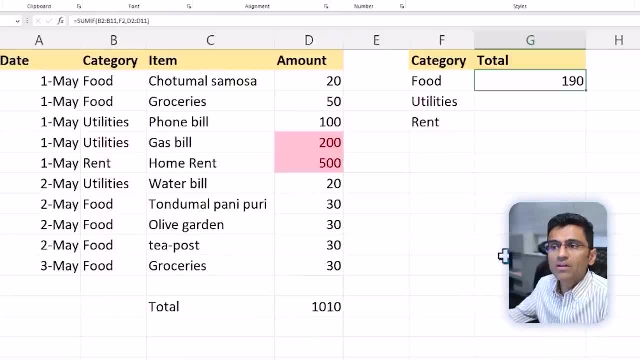 to sum them up. so when you do this you get 190. so that is your total food expense. you can control c, control v here. see, by default it will change this thing. so you can fix it: b2 to b12 or b11, rather okay, and d2 to d3. 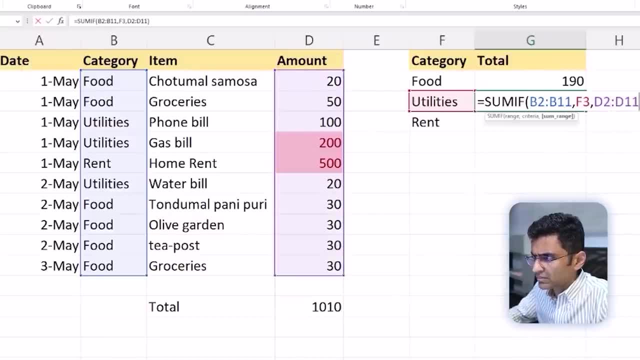 So that's the total food expense. So that's the total food expense. So that's the total food expense. So utility this much expense and sumif, once again, this, not this. actually this comma, this and this is the range. okay, if you want to verify that this total is correct or not, you 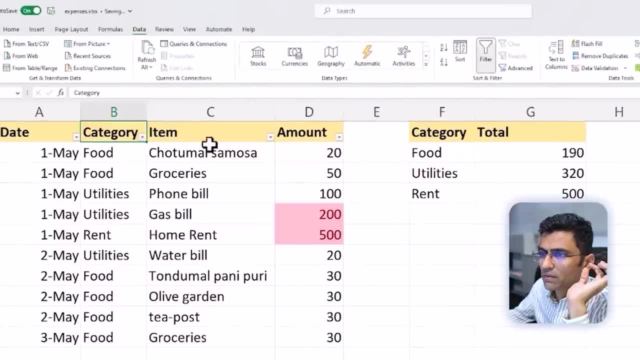 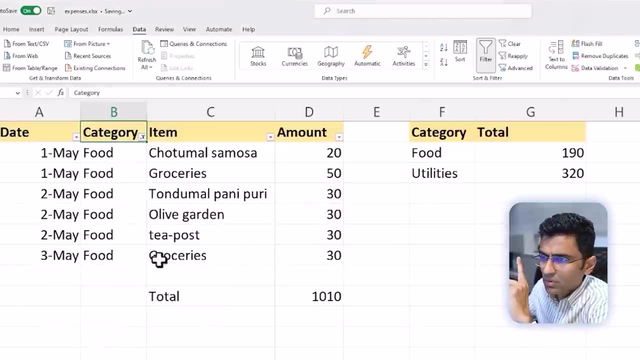 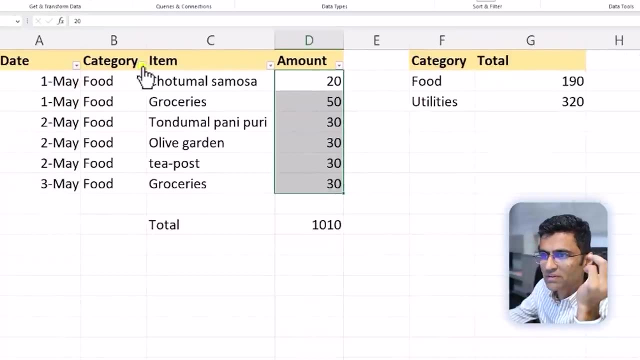 can do it using a filter so you can go to data. click on filter. now it's filtering per category. So you can see for food. on the right hand side you see 190. so I will say food- okay, food, I have this much. you click on it and at the bottom you see 190 so that 190 is verified. 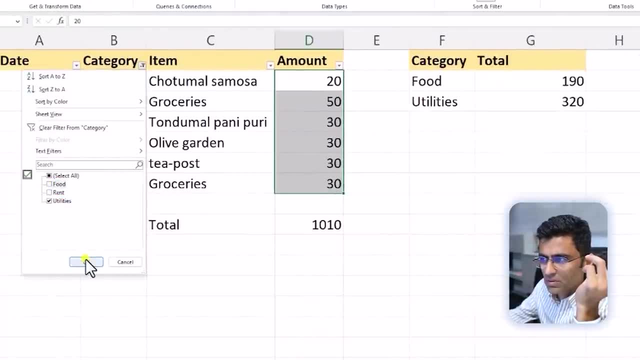 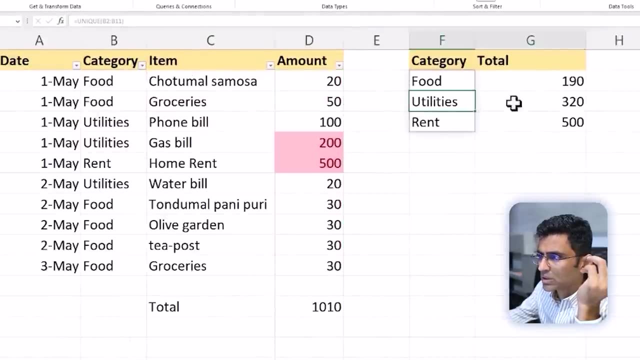 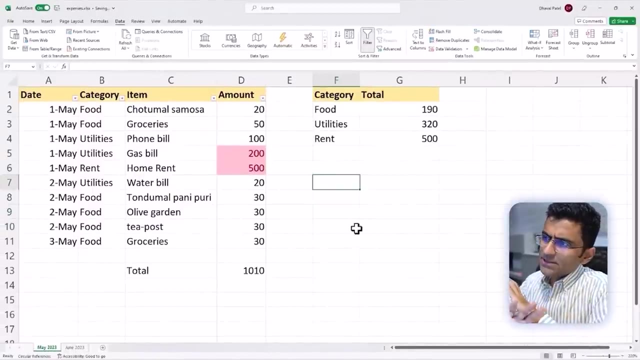 similarly, if you do utilities, for example, you see see here you see 320. so when you click and remove it utility, you see 320. so things are correct. Okay, Okay, Okay, Okay, Okay, Okay, Okay. So let's talk about some general cells in the excel file. 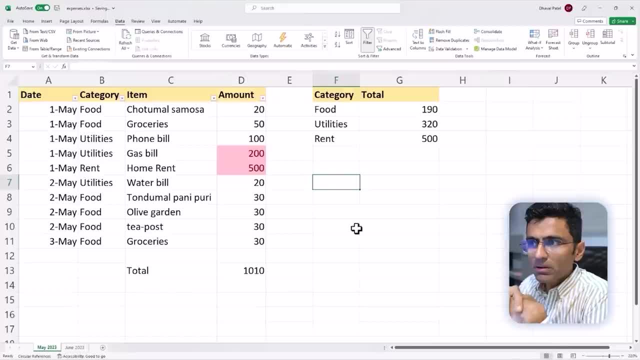 But there is something called table two, and table will allow you to do some advanced things. So here, whatever I have created, it looks like a table, but see, the table is pretty big. right, it's a whole sheet and in that you have bunch of numbers and text here. but if you want a, 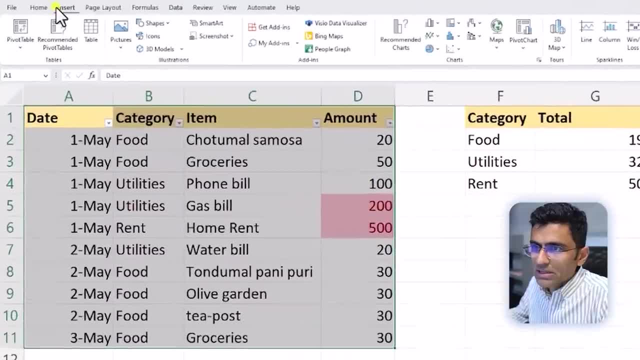 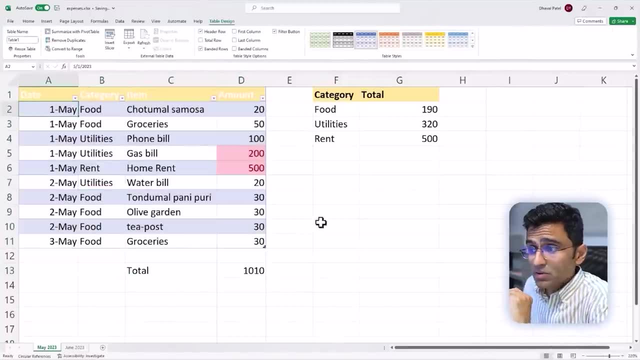 proper table. you can select this and you can say insert table and just say okay. Okay, now what happened is this thing become a table. so when you highlight your mouse cursor here, say at the top, you don't see table design option. but when you are, 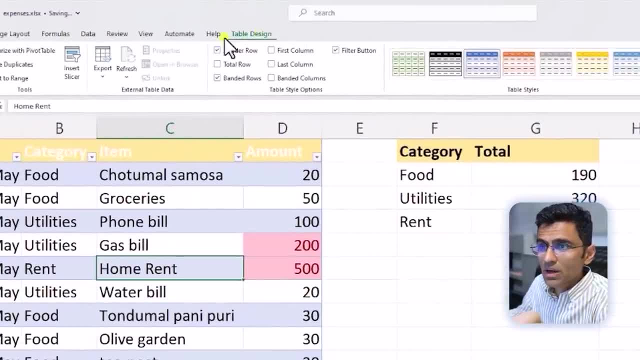 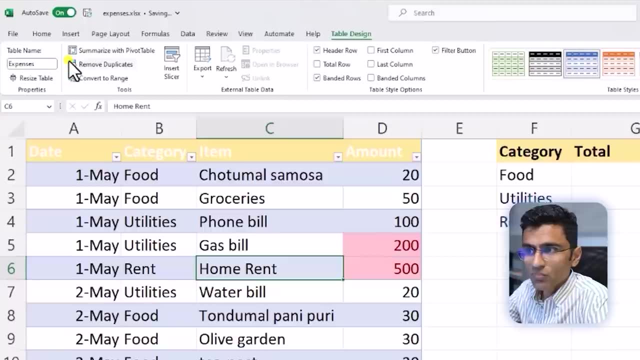 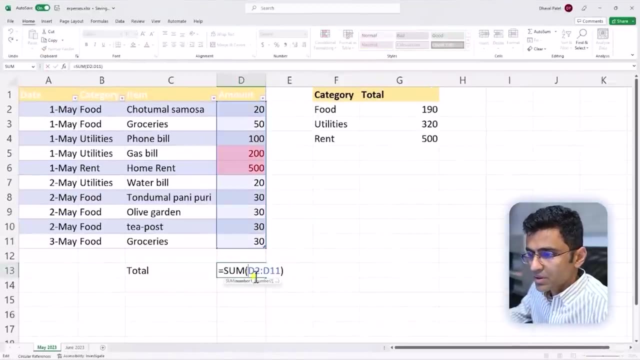 here you will see this extra option called table design, and when you click on it you can name the table. so I am going to say: name of this table is expenses, and how does naming the table helps? well, now, when you want to sum things up, you don't need to say sum d2 to d11, because that's cryptic and you. 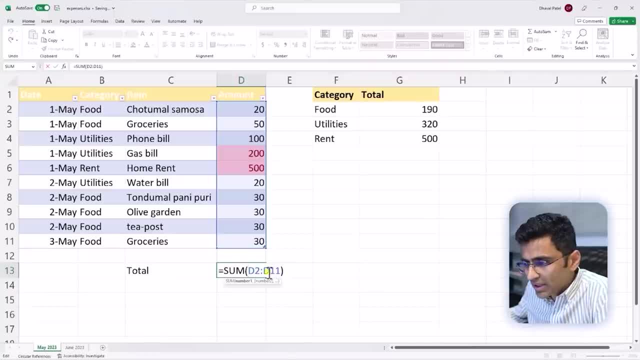 know, tomorrow I enter a new row, I have to modify the formula and all that. now I can do something like expenses say, because expenses is my table and when you put this bracket it will also show you the column name and you can hit tab bracket: close now, expenses. now see, this is. 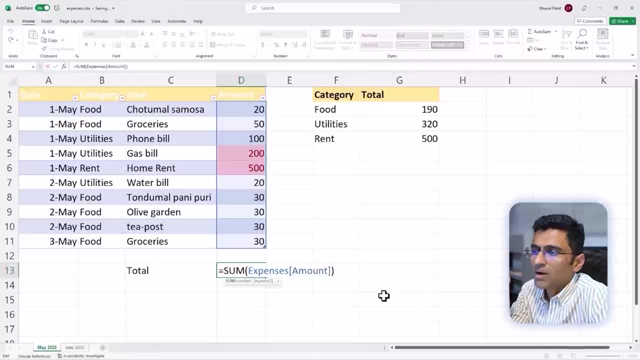 you can see that the table is now in the column name and you can hit tab bracket- close now expenses. now see, this is now expenses. now see, this is much more readable than just saying amount or just saying d2 to d12. what does it mean? d2 to d12? it's just random cells, but here there is a table. 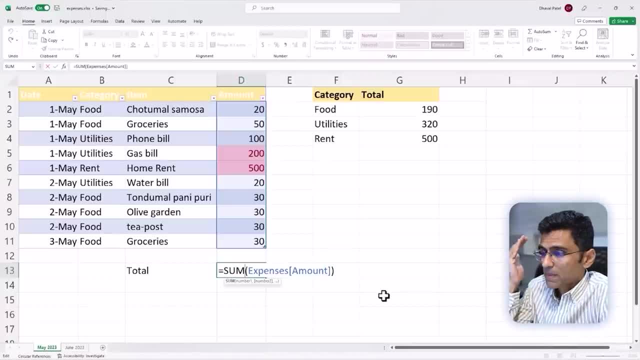 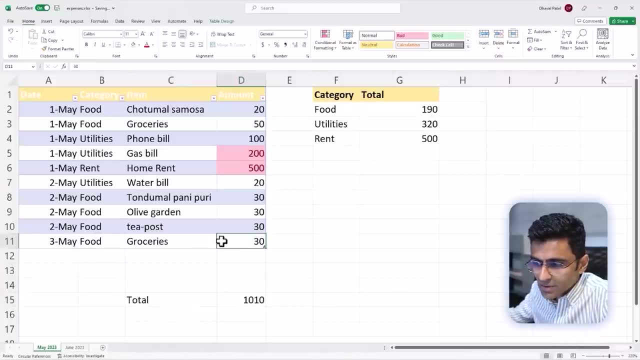 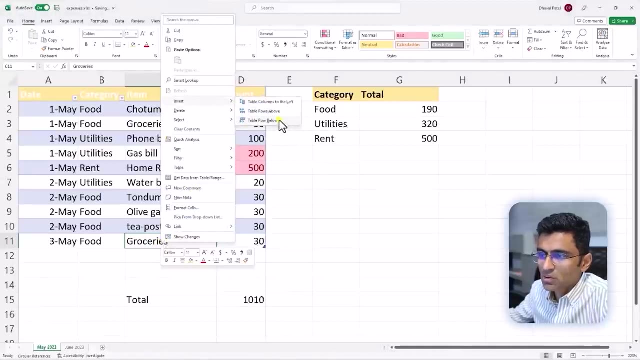 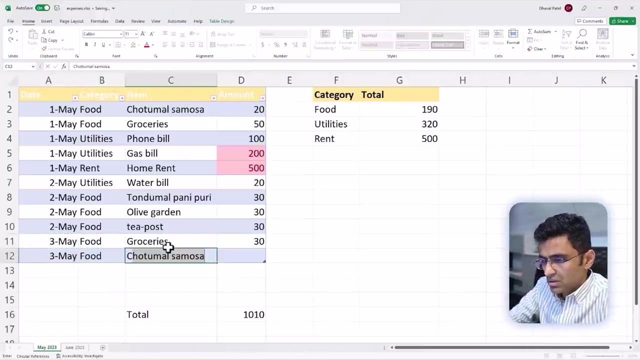 name expenses and there is a column name amount, so this looks much more readable also. the other benefit is- let me just put it here: ctrl X, ctrl V, whenever you are adding a new row, for example here, let's say, you right click and you see, insert rows below and let's say: on third, may you incur another food expense? 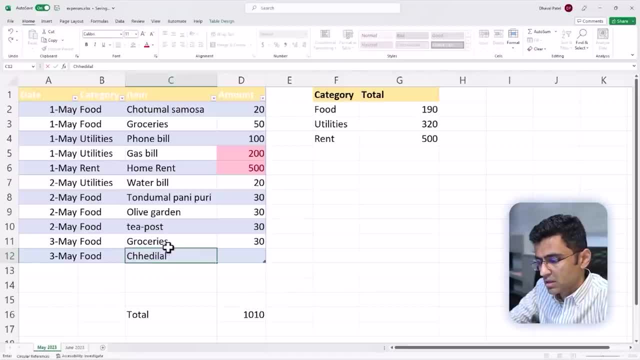 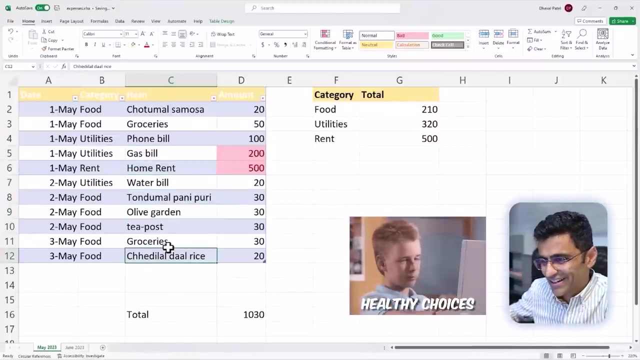 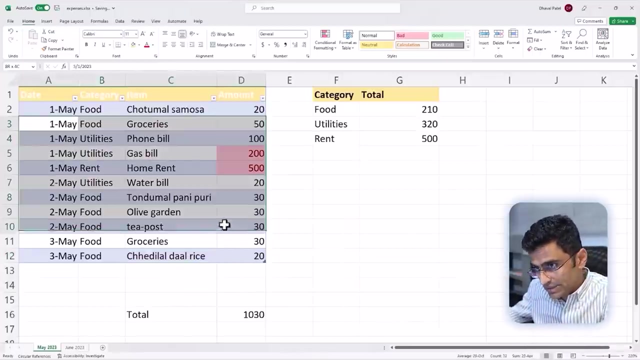 let's say chedi laal rajma rice or chedi laal dal rice. okay, dal rice is my favorite food, by the way, and I don't like all this pizza and bourgoneau- all that I like to eat- or Indian traditional food anyways. when I inserted this new row, it became part of the table. see that it is. 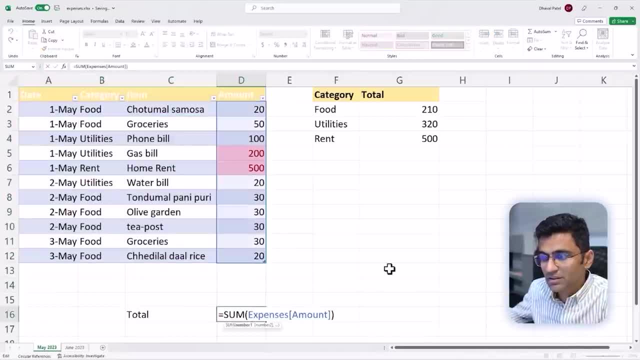 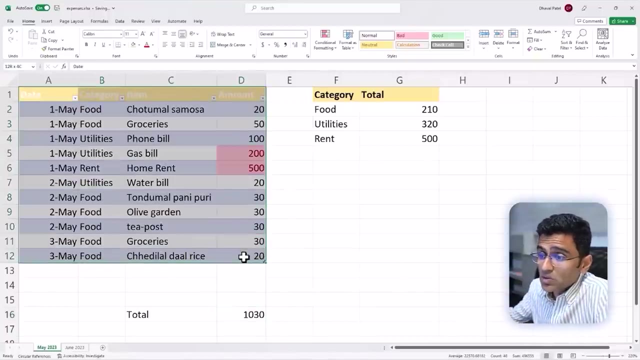 highlighted, so it become part of the table. not only that, the formula got modified. the formula is now taking that into account. formula is same, by the way, but since the new row is part of the table, it came here automatically, so that's another benefit. one more benefit is you select. 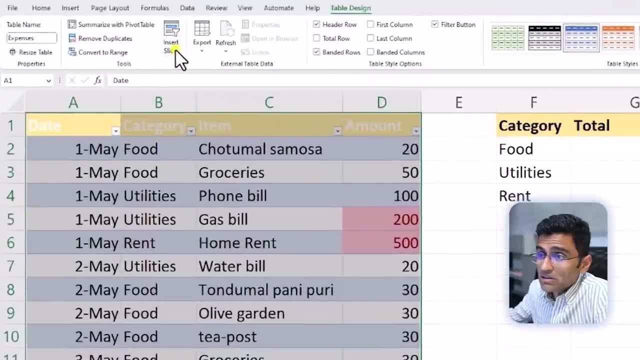 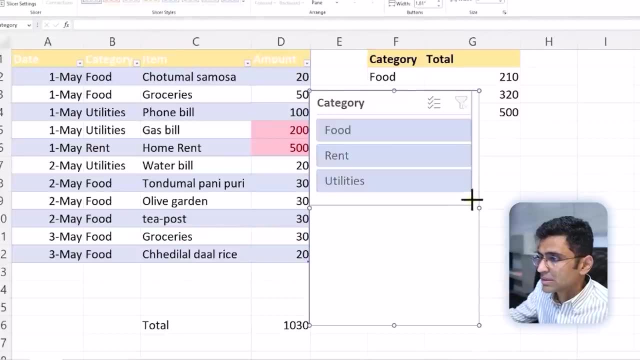 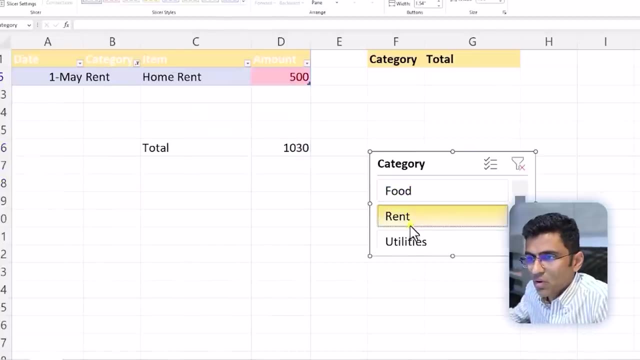 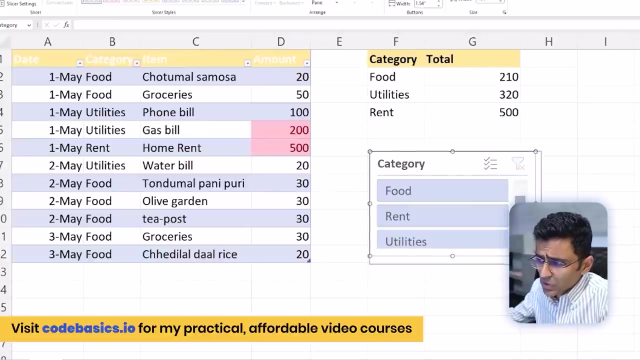 the table and you can just say insert slicer. and you can say: let's say you want to do category wise breakdown, so you can just say category here and this slicer will allow you to filter. so i want to now see only food items, only rent, only utilities, see, so you get all of these useful features. 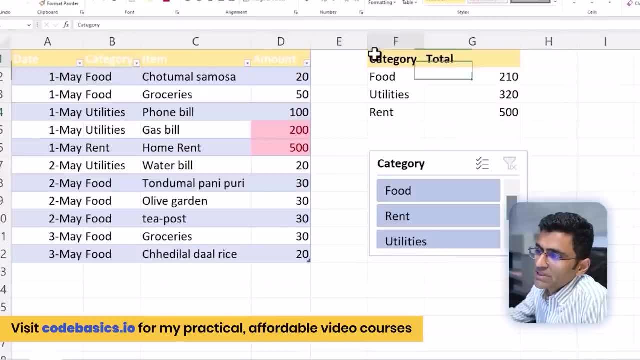 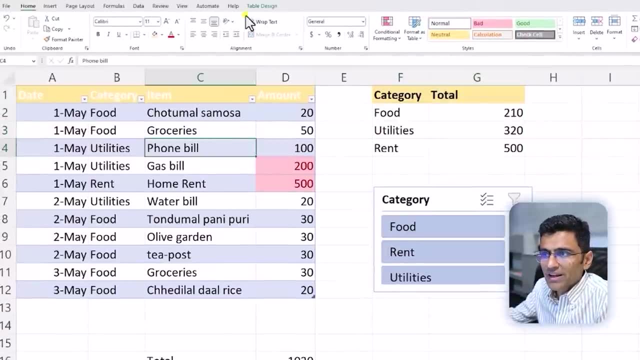 if your cells are table, if you have, see general this is not a table. but if you have, just if you click it see there is no table design. but if i click here there is a table design, you can insert slicer. you can do so many things. you can, by the way, insert total row as well, so you don't need 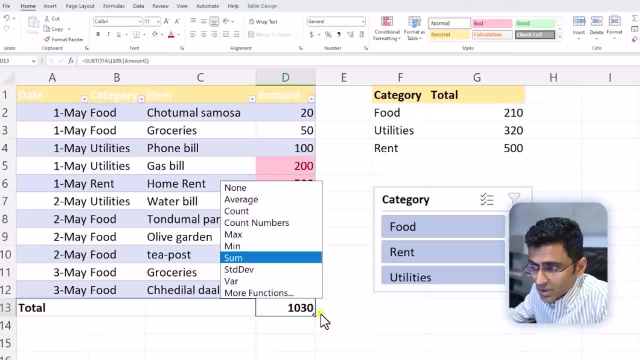 to even even type this in. you have a total row by default. you can say total sum, average, count. let's say i want to know count how many items are there 11? okay, i want some here. there are many more functions. you can do min, max, all basic arithmetic. so these are the benefits. 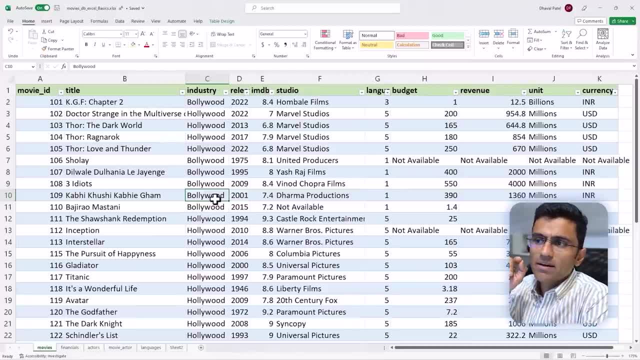 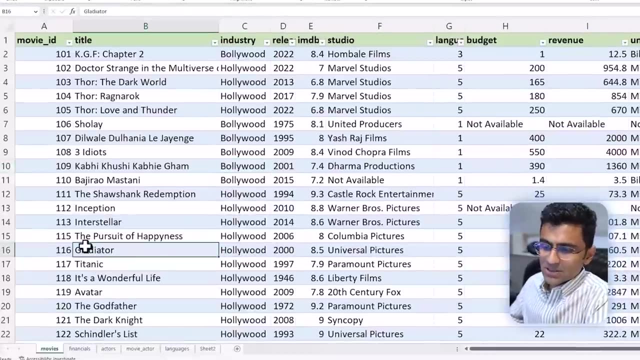 of the table. now that you've understood excel basics, let me introduce movies data set. and this is the data set we'll be using in many of the future videos in this playlist. that's why i want to just give you broad introduction on this particular data set. here you see multiple sheets. 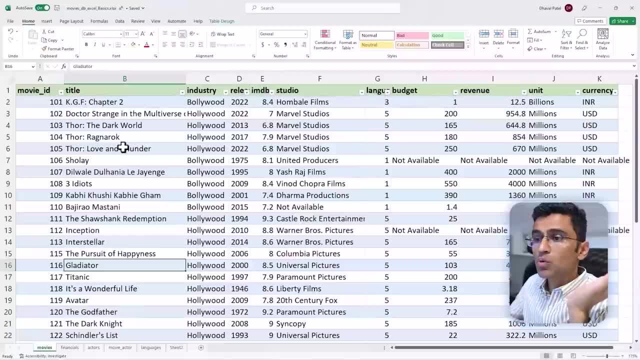 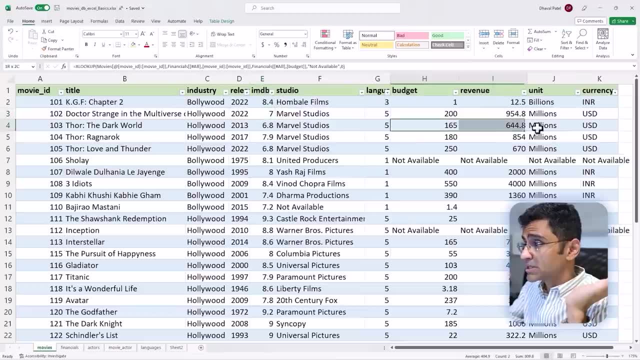 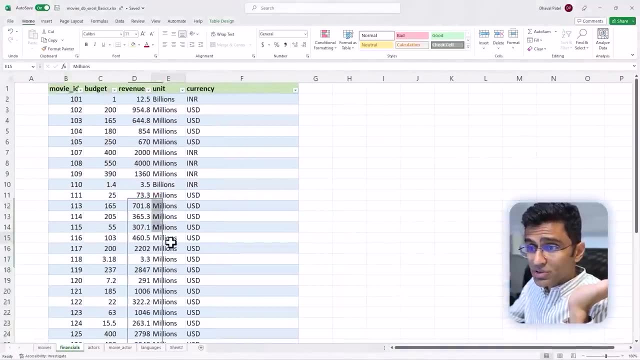 okay. so first one is movies, where we have movie name, which industry- bollywood or hollywood, uh, their studio imdb rating, budget, revenue, etc. and in the second one you have financial. so, by the way, financials. i have used some formulas and i have merged this table into here. okay, you can see that we have used x. 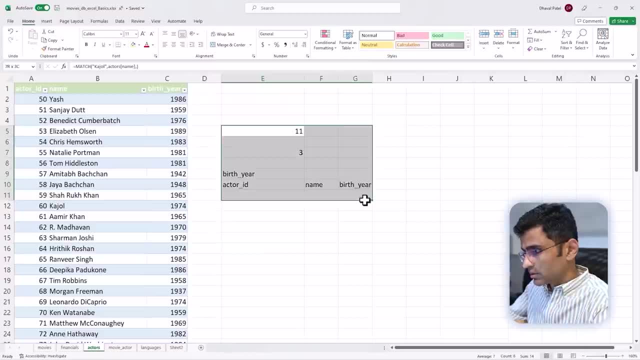 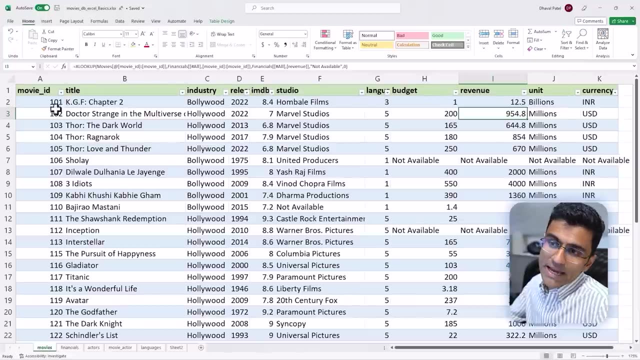 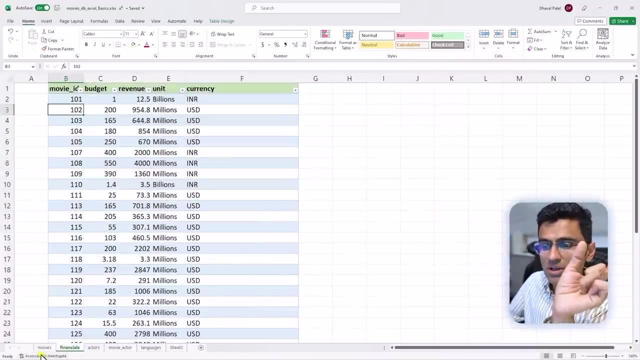 lookup and then you have actors table. let me delete all these extra things, uh, movie actor languages and so on. so movies has movie id, okay, and that movie id you can use to link with the financial table. so let's say this: kgf, chapter 2, it is 101, so it is 101. the budget and revenue was 1 and 12.5. 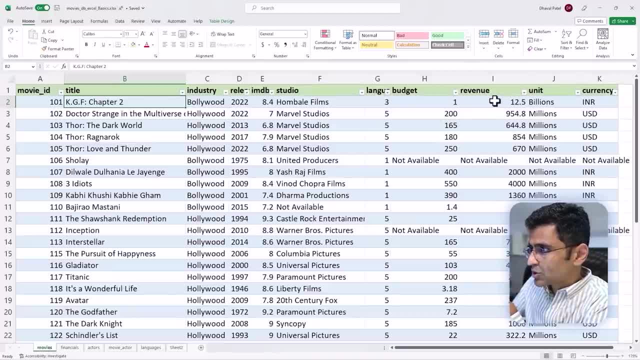 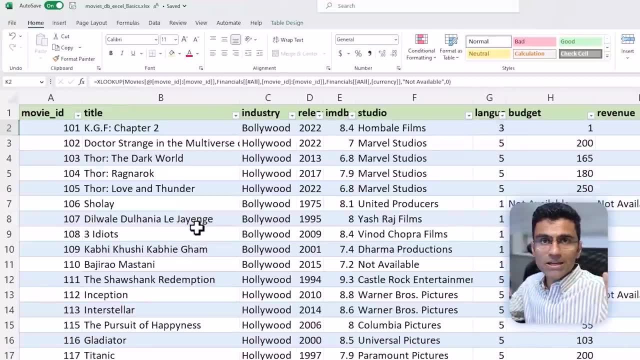 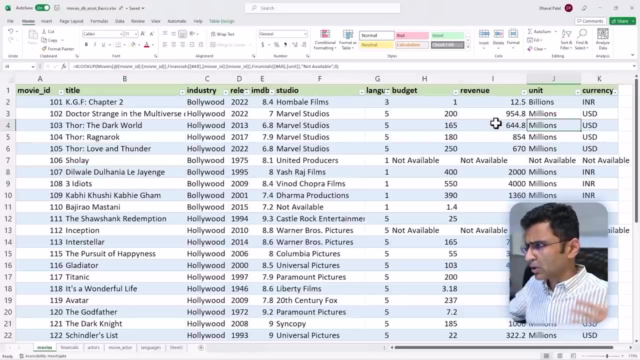 billions inr. so we used 101 movie id to pull this revenue and currency. i'm not gonna go in x lookup formula, but x lookup formula is something that you use to combine these two tables. the information on this x lookup formula and all those details are available in my 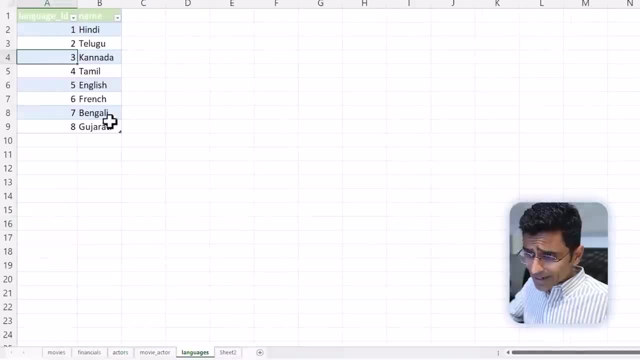 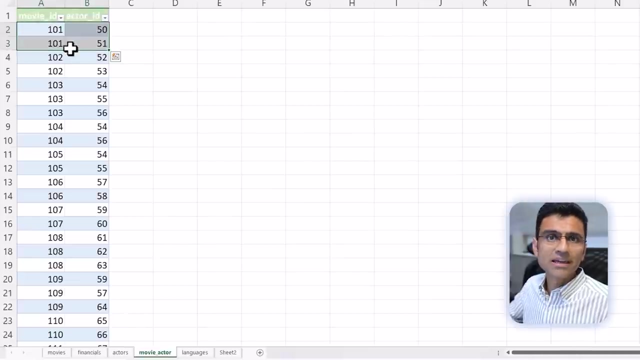 excel course. uh, in terms of languages, see movies have a language id. let's say three: kgf. chapter 2 is three. so what is the three language? karnada, okay, so that's a simple table. then you have movie actor. so 101 is kgf2, the movie actors are 50 and 51. so what is 15, 51, 50s? yes, and sanjay that. so if 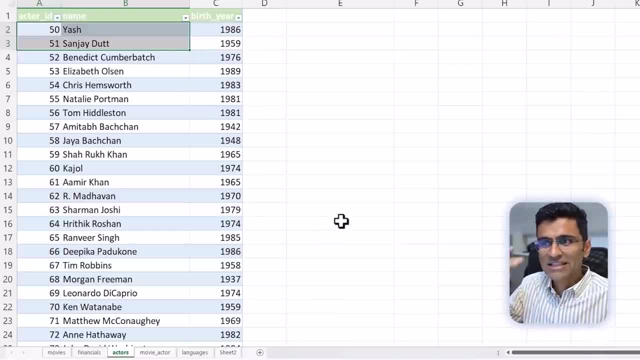 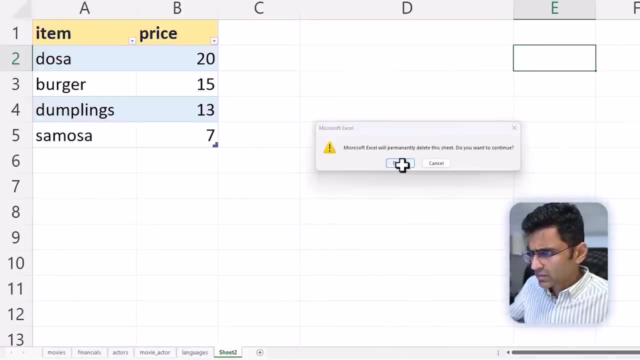 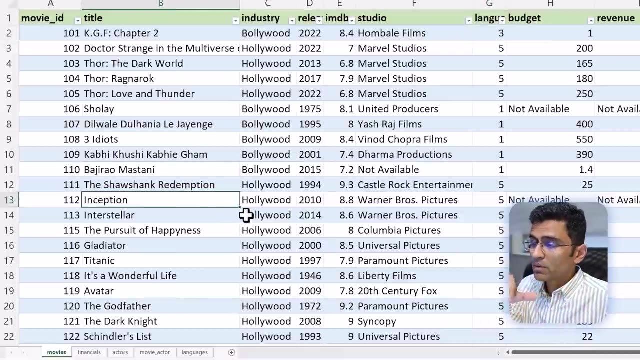 if you have seen KGF 2 movie, you know Jess and Sanjay Dutt are the actors. okay, so these are the things we have. let me delete it. this is an extra thing, so we don't need it here. so these are the tables that we have now. in the future videos we will be performing some data analysis on on this. 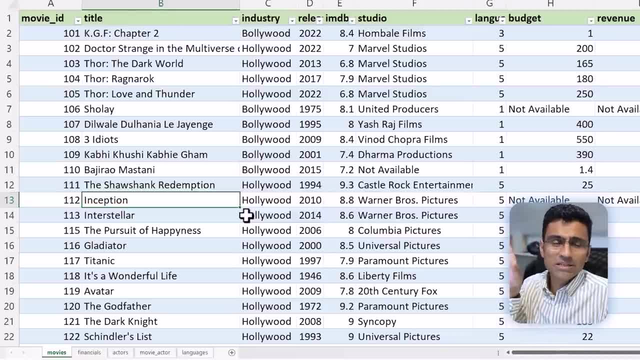 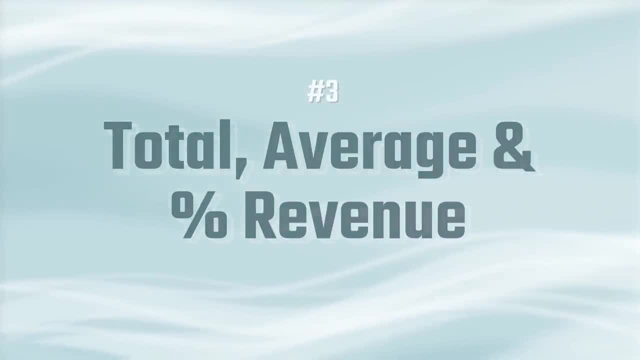 particular data set as well, as we will be using some other data sets too. all right, so keep on watching. if you like this video, please give it a thumbs up and share it with your friends who want to get into data industry on this movie's data set. now let's perform the basic business: arithmetic. 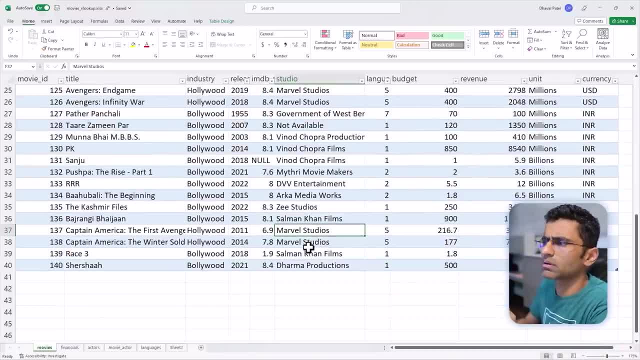 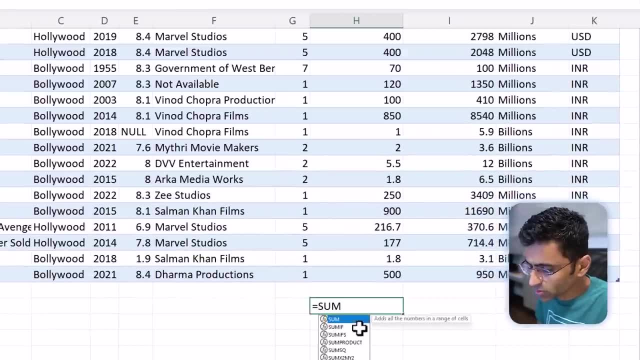 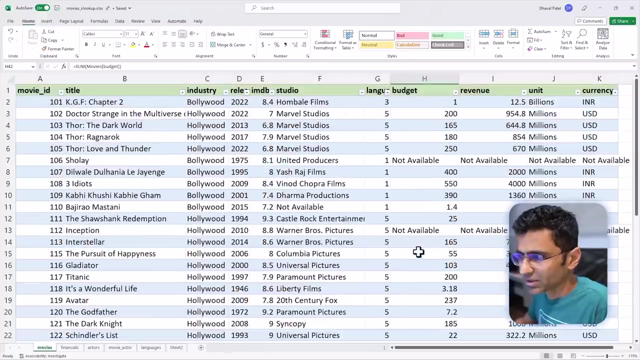 here. when you're looking at the number, obvious question that you have is: what is my total budget, or what is my total revenue, and you can do that easily by doing so, and let's say budget and that is a total sum. but is this number correct? well, it is not, because these numbers are either in. 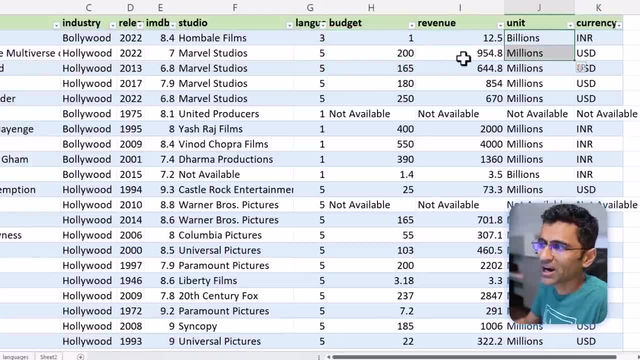 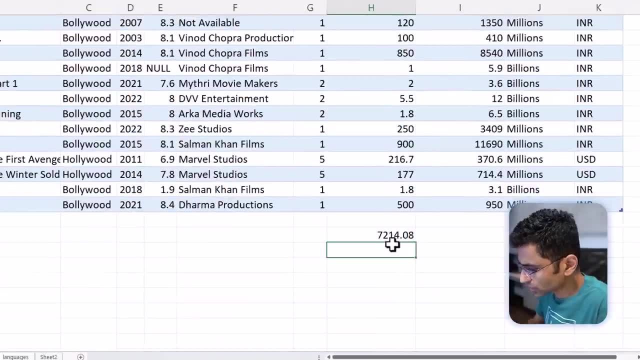 billions or millions, and their currency is also different. so you can't add numbers if they're on a different basis altogether. so you have to standardize them to a common currency and a common unit them. Create a billion between these three captured values. let's do that process right now, so then only you can sum them up. so let's do that process. 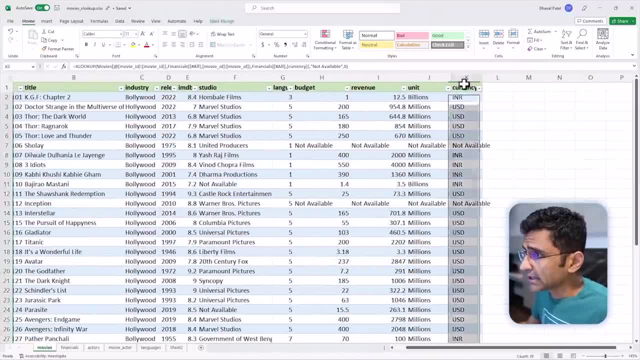 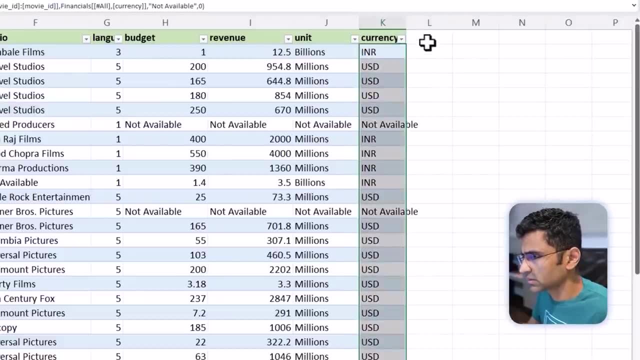 right now. so I'm going to delete this because this number is anywhere wrong. i will do control scroll down so that the font size reduces, and then I will create. I will drag this and I will create. i will create 2 new columns, so I will call this. budget in millions. so first I want to create a column where all numbers are in billion. so let's do this and create a billion and drag it. okayelese never fills out this column and then either refers the number and it is not more than 21, 7 Grams. so let's do that here, let's do this and push'd. 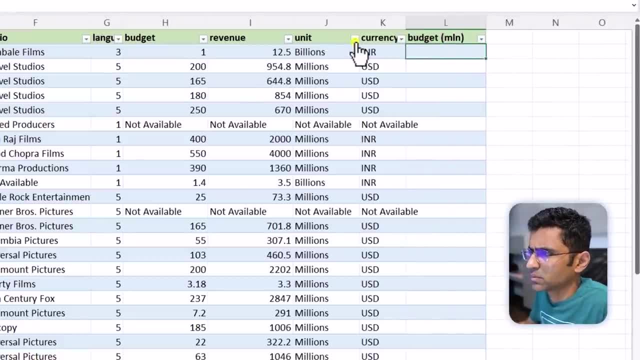 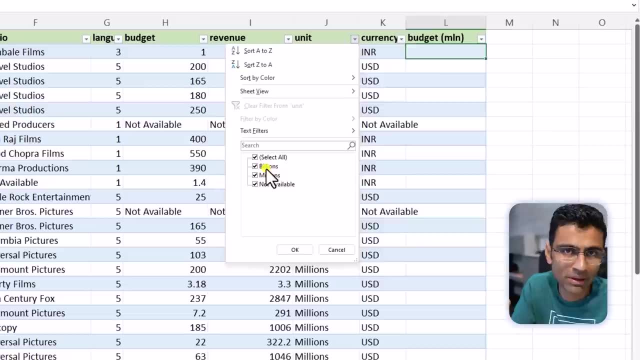 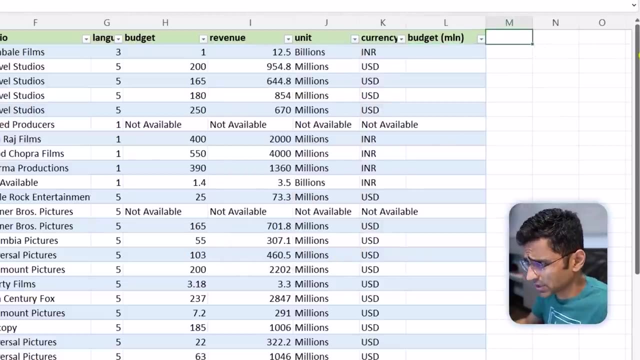 and why do I do that? because when I look at this unit, I have either billions or millions. so I can easily convert billions into millions and get all numbers in a single unit, which is millions. and I will do the same thing for revenue. so I will say: revenue, million enter. okay, now how do you? 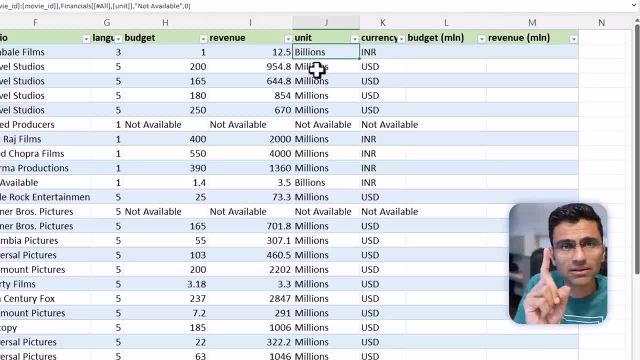 convert billions into millions. so one billion is thousand million. so what you have to do here is use if formula and you can say: if my unit is in billions, so if this is in billions, then multiply the budget number with thousand. okay, otherwise, whatever number is there, just keep it. 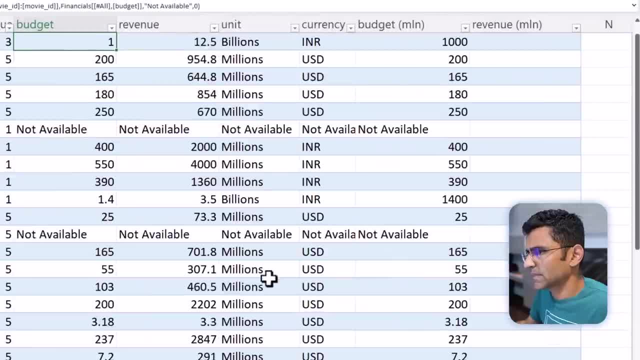 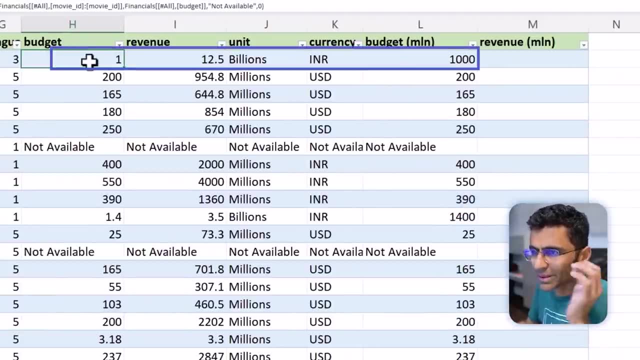 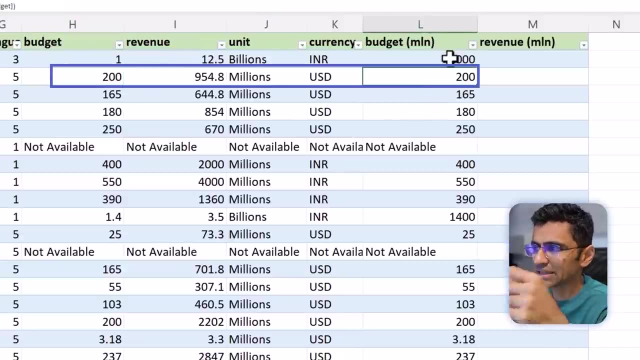 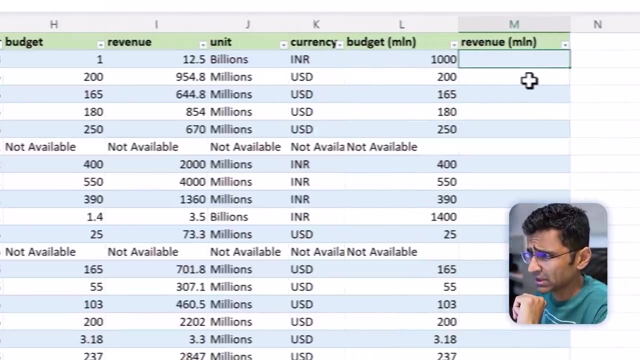 so now you see that, I'll just do control scroll to increase the font size. now you can see that the one billion number is converted to thousand, but two hundred million number remained as is. so you can say that all these numbers are now in common unit, which is millions, and you can do the same thing for revenue. so 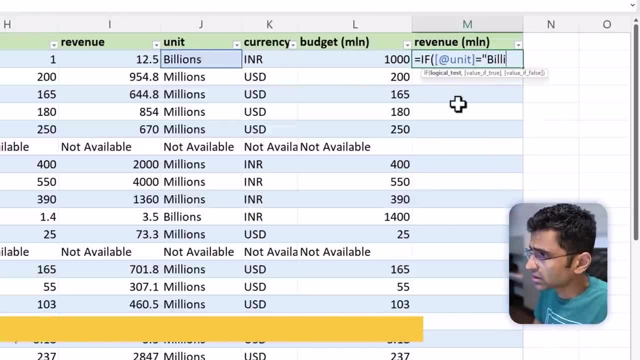 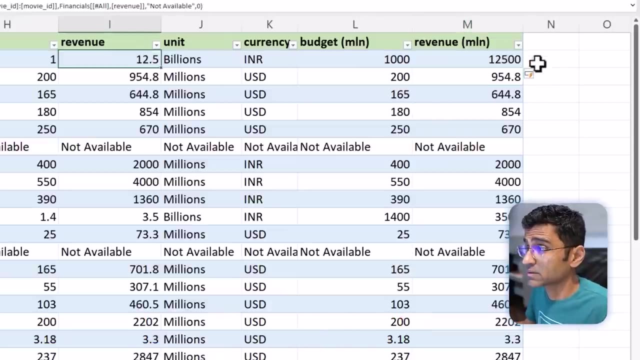 here. I'll say once again: if the unit is billions, then revenue multiplied by thousand, else revenue brackets close, complete. 12.5 is converted to 12,500, which is good. but the 954 million dollar is as it is, it did not change, which is good. okay, now let's. 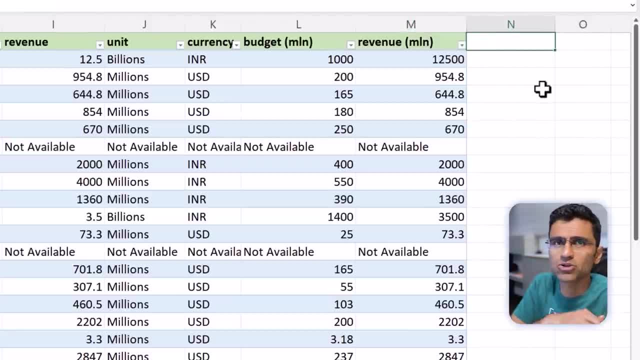 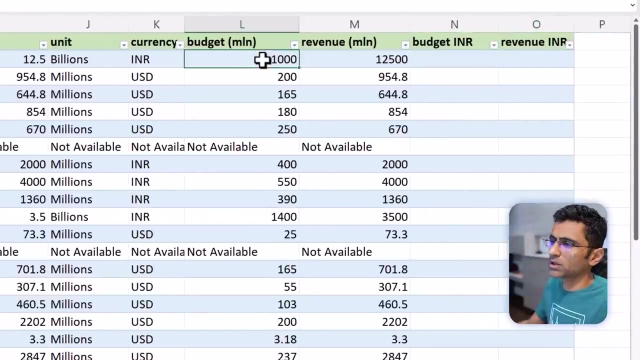 convert these numbers into common currency. so I'm going to use INR. so I will have budget: million INR, but I'm feeling lazy so I'll not write million. just understand that this is million. so this will be budget INR, revenue: INR. and let's convert this number into INR. so if it is INR already, you don't need to do anything. 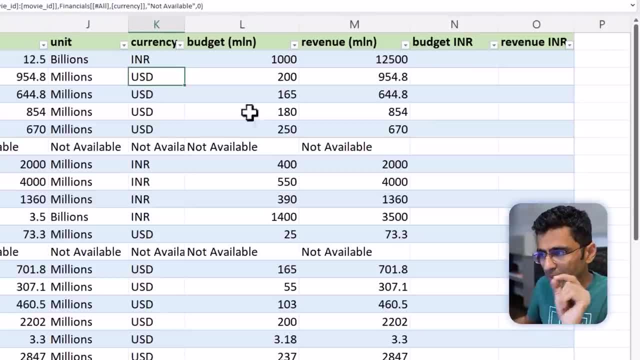 but if it is USD, then you need to multiply this number with USD to INR conversion rate, right? so let's do that. so if my currency is USD, then multiply this number with 80. 80 is the current USD to INR rate. it keeps on changing, but I'm just going to estimate it to be 80. otherwise, 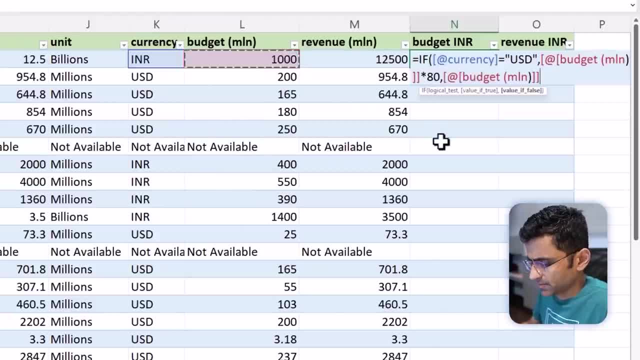 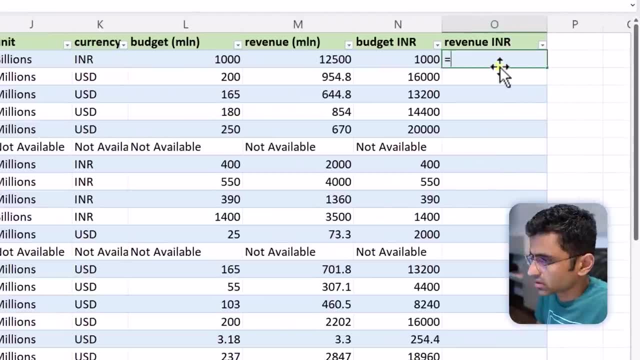 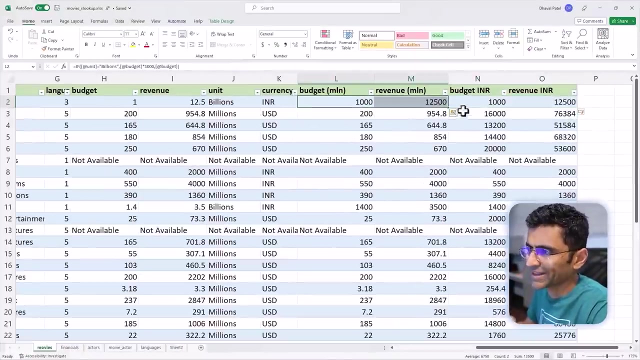 keep the budget in mind- millions, okay, and do the same thing for this one as well. so if my currency is equal to USD, then multiply this number by 80. keep this number done, okay, and you see that this is the number for KGF 112500. it's remains same. 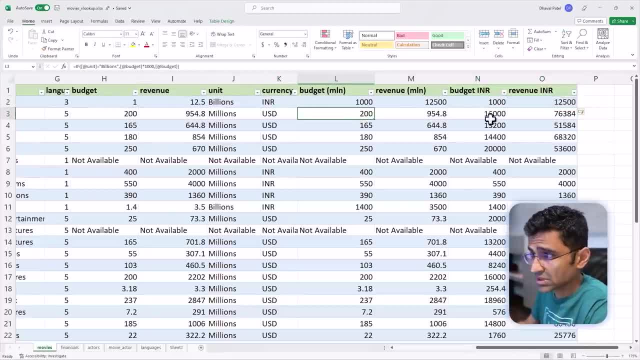 which is EXP for 12500, and so in order to convert my value, it will have to deposit a, because we are in INR. But this number, since it was in USD, we multiplied by 80, so 200 into 80 is 16,000,. 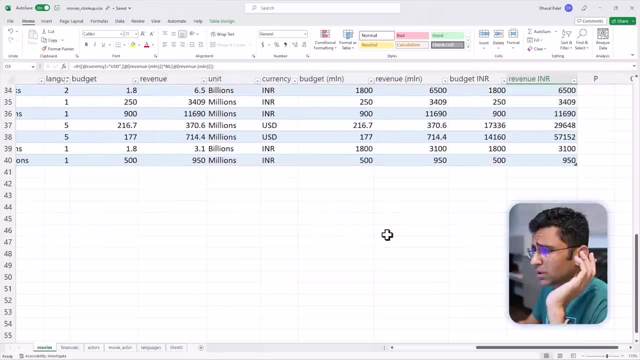 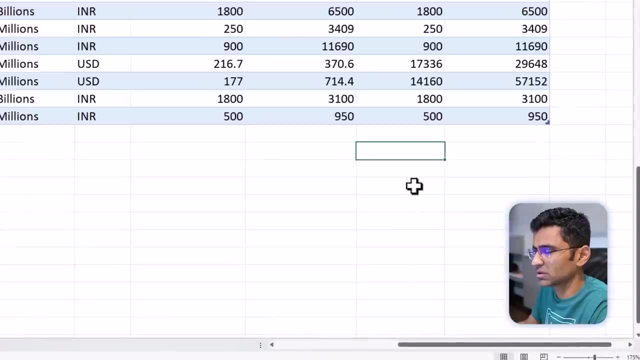 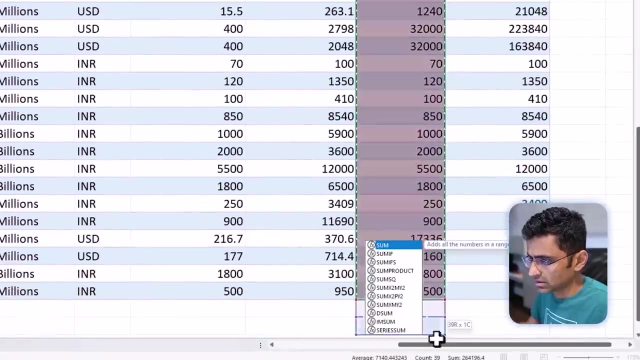 and we did the same thing here. okay, Now, if you want to get the total budget and revenue in a single currency, here you can do that. So here you can just sum this entire, this entire, this entire, okay. 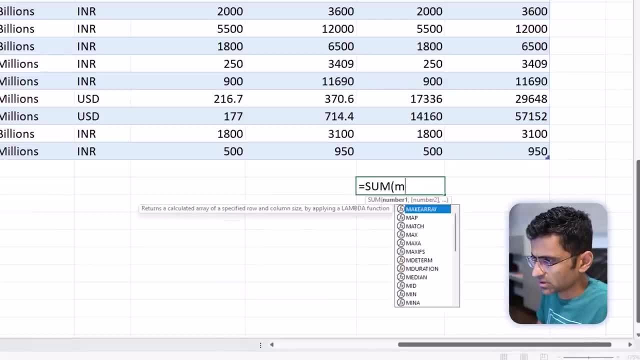 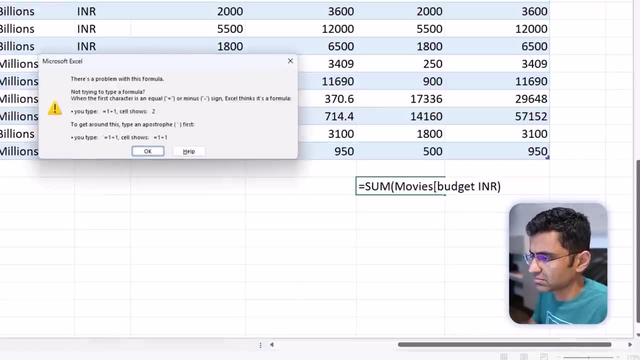 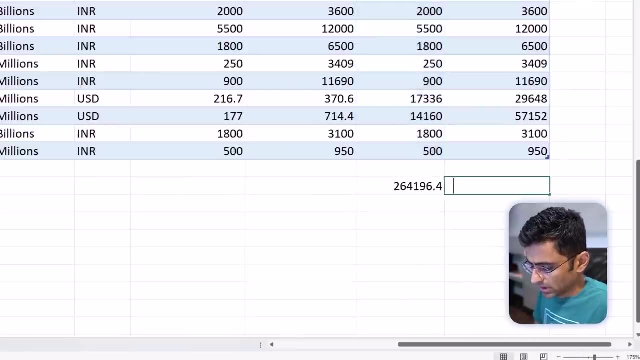 I'm just gonna do it. Some movies: budget: INR. Budget INR bracket was missing. Some movies: revenue: INR. You see, It's so easy actually. So these are INR numbers so you can go here. 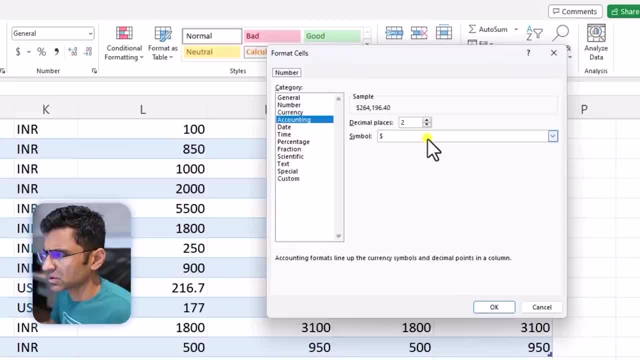 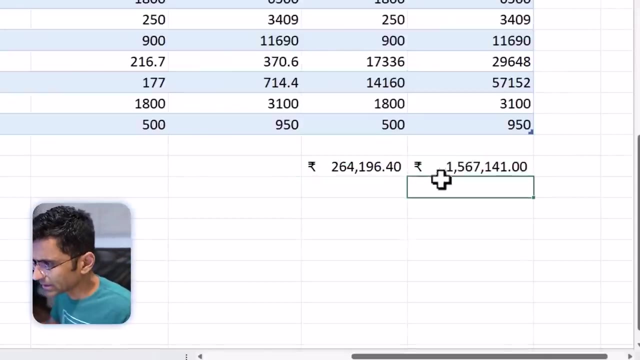 and you can select the INR currency. So you can go to More Accounting Format. scroll down, scroll down And whenever you see INR Symbol, say English India. So these are all INR numbers. And what is this exactly? 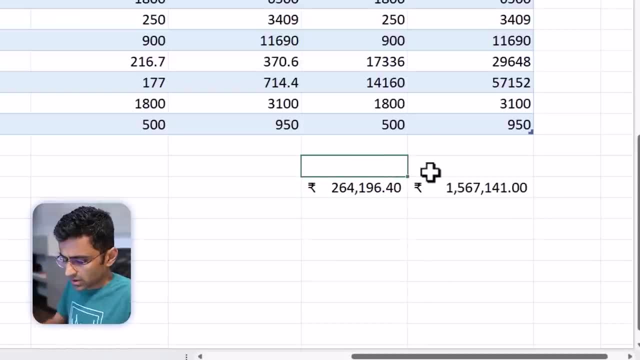 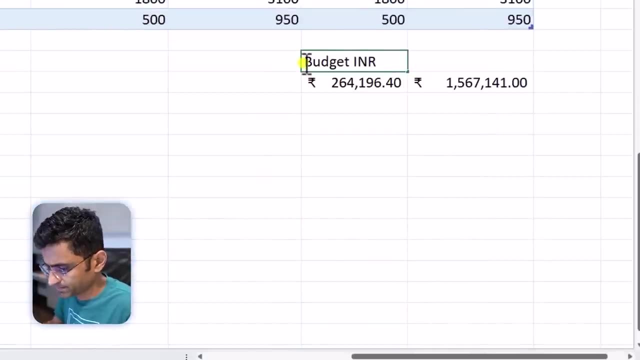 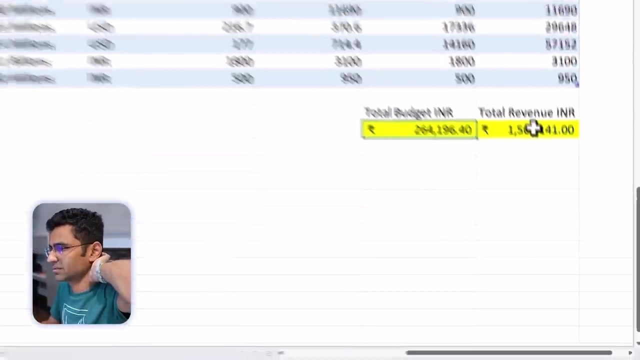 So let me just Control-X, Control-V. This number is budget INR. okay, so budget INR, total budget. you can highlight these cells as well in a special color and this is total revenue in INR, and these are million. so this many million INR, it's a big. 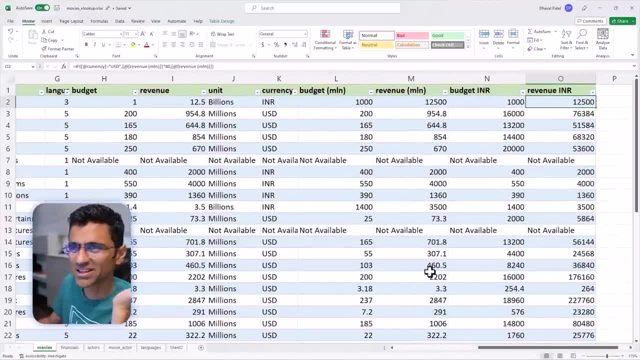 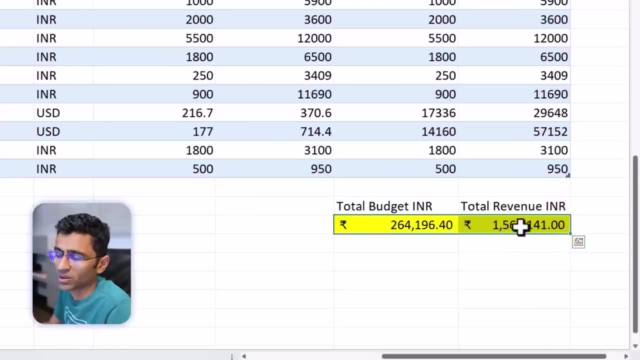 number. but, yeah, all these movies are doing so much business nowadays. KGFRRR, if you're watching Bollywood movies, you know they. they make so much money and, by the way, this is all okay. so this is Hollywood and Bollywood, both, so we can understand movie industry right now. they make a lot of money and if you want to, 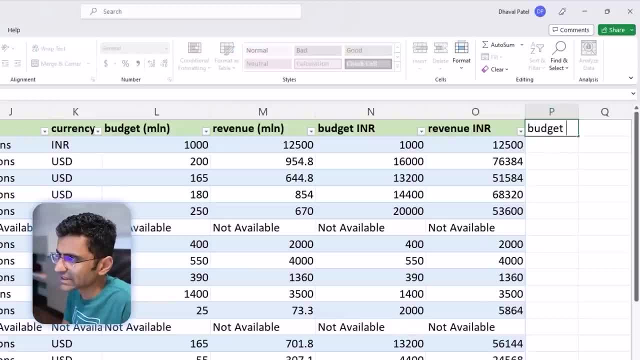 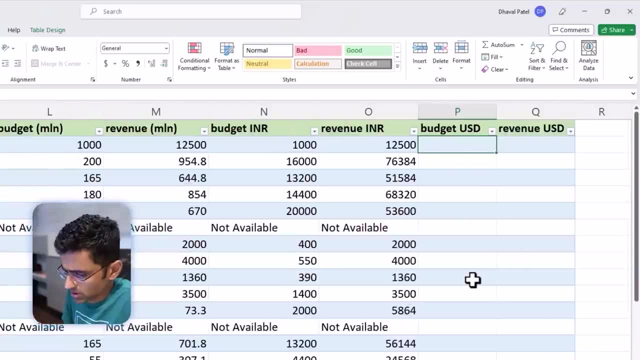 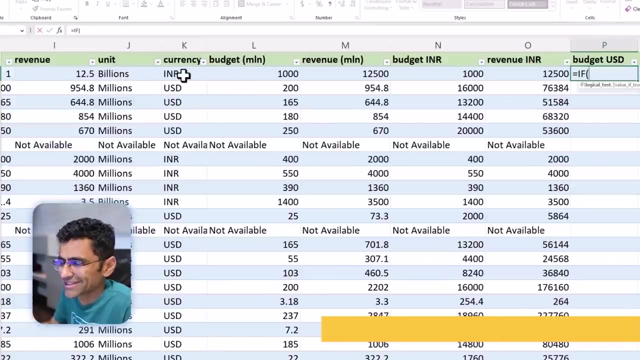 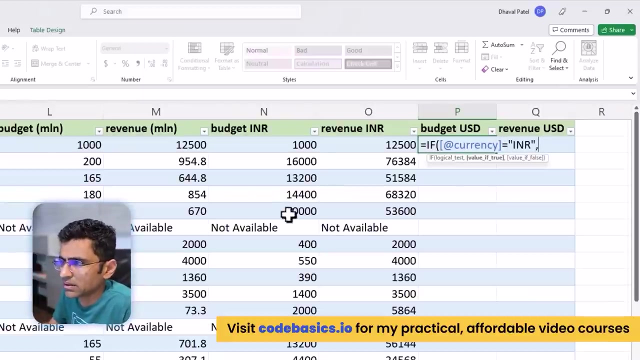 do the same thing for, let's say, USD. so I'll say: budget USD, revenue USD. so what is budget USD? so here you will say: if the unit or the currency is in INR, if the currency is in INR, then you want to divide that number. you want to divide. 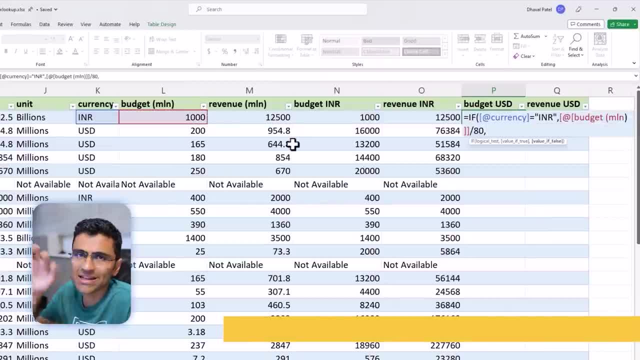 this number by 80. once again, 80 is an average. when I was at Bloomberg also, you know, when I worked at Bloomberg New York office, we used to have these kind of issues with currency and many times we'll use the average of quarter. let's say you are looking at earning estimates of any company and you 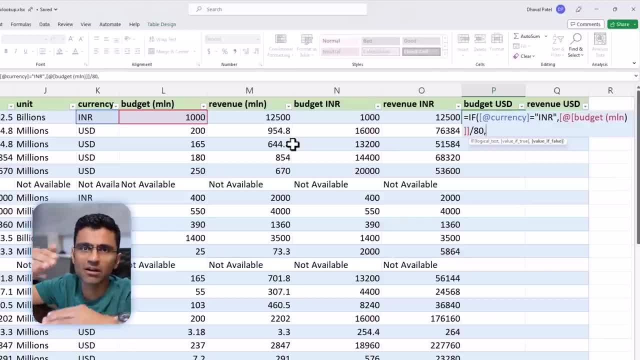 have two cells which are in different currency. you will take an average and sometimes the brokers will provide the currency spot rate conversion rate for average, like average, let's say average of last three months or average of last whatever time period, and they will provide that if you want, or something. 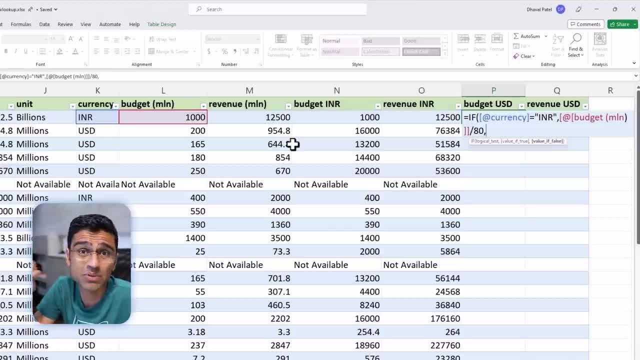 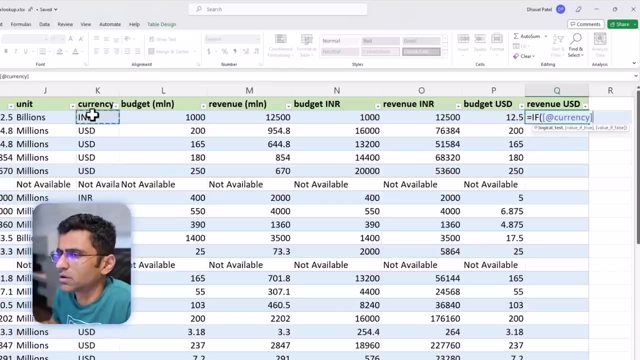 real-time. you can call an API through Excel and get the real-time spot rate. spot rate is nothing but a currency conversion rate, okay, so you do that bracket complete and then once again, if your currency is INR, then revenue divided by 80, else that, and you can do quick verification. so here, budget. 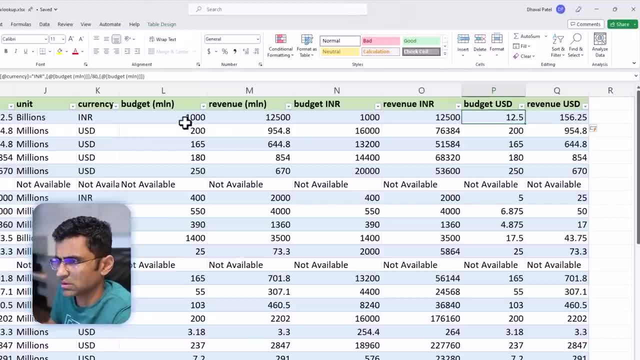 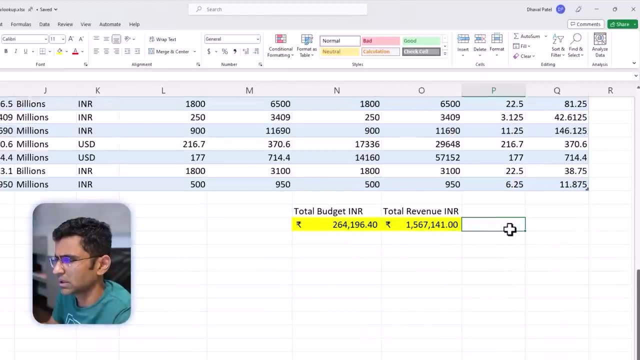 in USD, so budget million was this much. so this divided by eight will be this number, and but for this number, since it is in USD already, you kept the number same, all right, and here you can just sum it up. let's see if this formula is going to work. yes, it is working, okay. so you got all these numbers. now let's 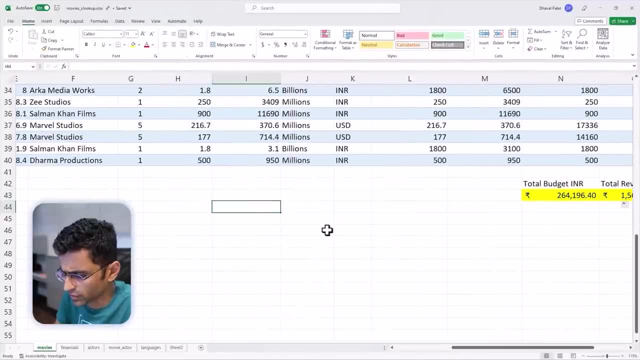 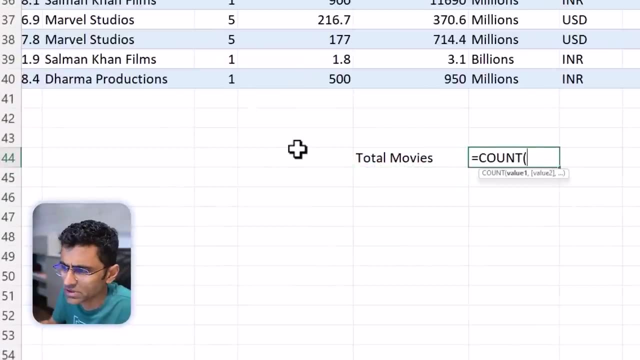 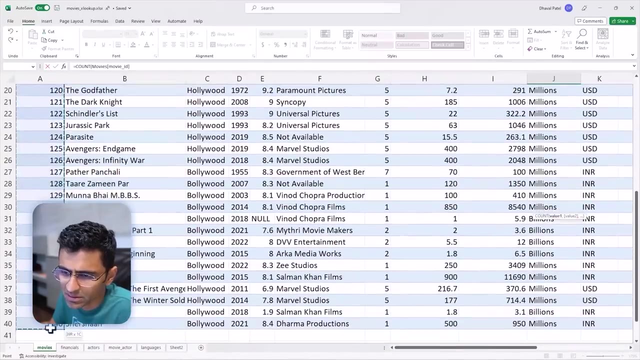 do some other type of analysis. so what are my total number of movies? so I will say my total number of movies is equal to count, count of all the movies. so you can take any, any column actually, but I'm just gonna take movie ID. okay, and so my 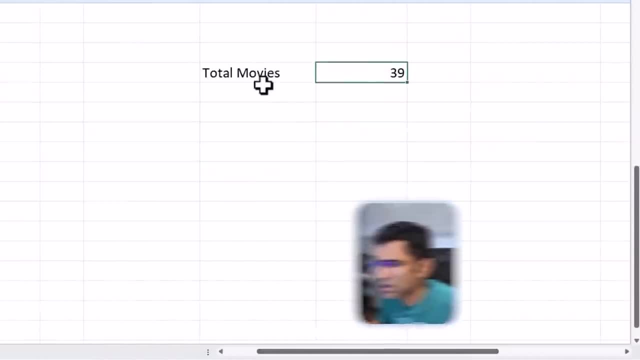 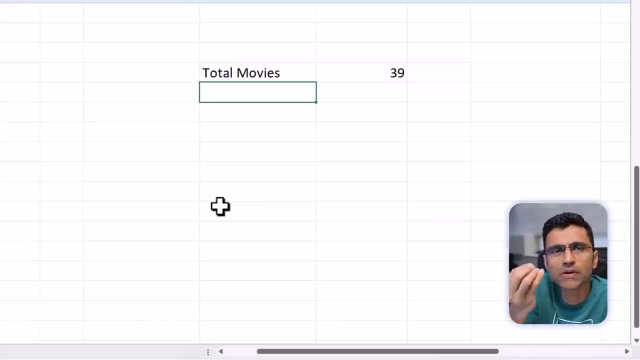 total number of movies is 39. okay, and what are my Bollywood movies? let's say I want to do some analysis on Bollywood movies, such as: what is my average Bollywood movie revenue? okay, so let's do that. so first you need to count total Bollywood movies. so total number of Bollywood movies are: 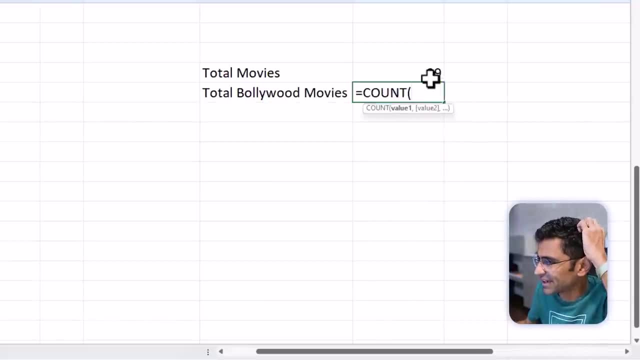 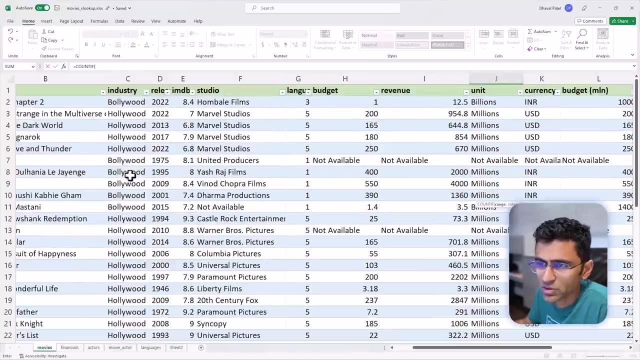 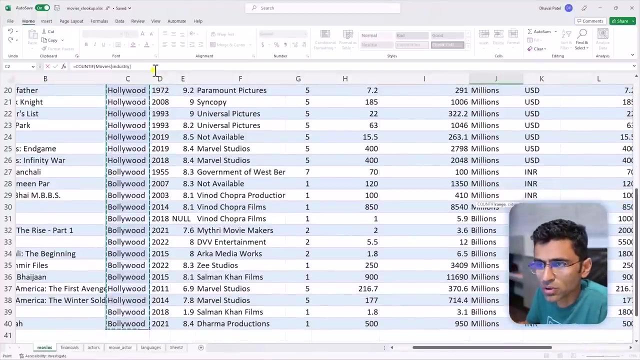 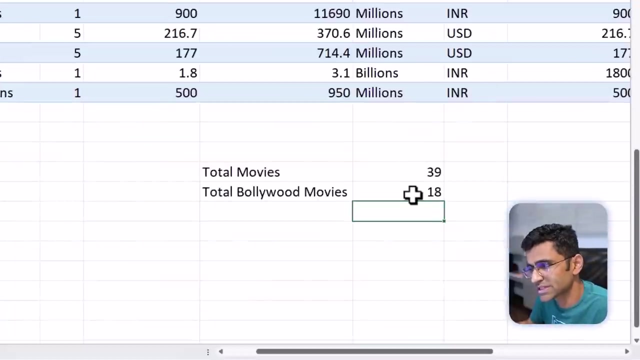 count of movies. but if you do count, it it's not gonna work because you want to do. if so, there is a thing called count if, where you specify the movie because you want to. just you know, if you specify the column on which you want to apply criteria, and your criteria is: I want to count only Bollywood movies, which. 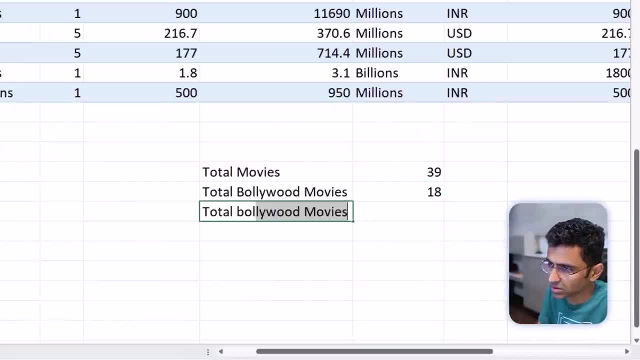 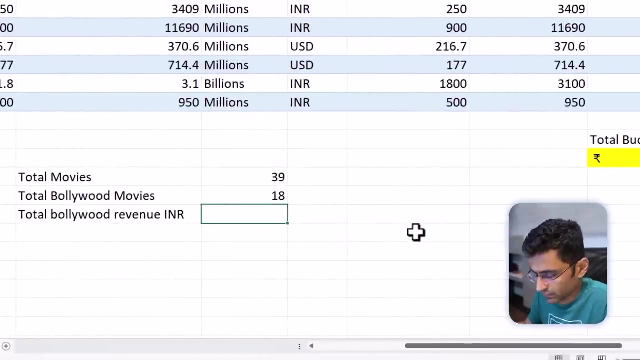 is 18 and what is total Bollywood movie revenue in INR? we can do INR USD, but since it's Bollywood, we'll do Bollywood movie revenue. so what is my Bollywood movie revenue? obviously you have to use SUMIF. see here: whatever you calculate in the yellow cell, that was. 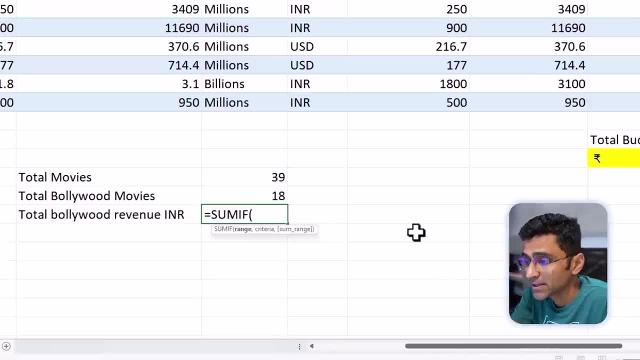 total all the movies, Bollywood, Hollywood. here I want to only count for the Bollywood movies. so, SUMIF, what is my range? so my range is industry. okay, on the industry, you want to apply Bollywood criteria? so in the industry column it will filter based on Bollywood text and then you. 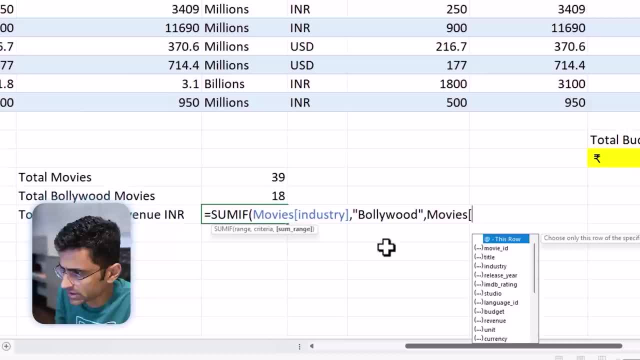 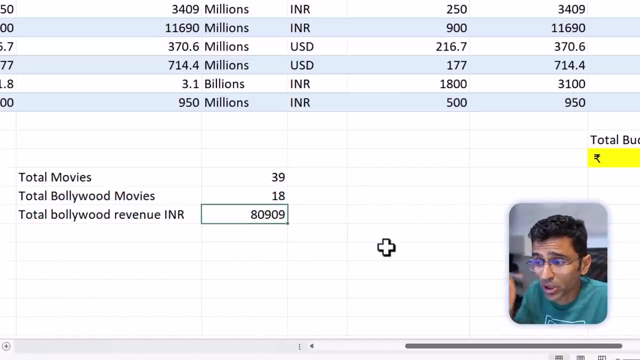 want to sum. how do you want to sum? so, in the movies you want to calculate the revenue. so, whatever revenue INR you have, you want to sum that up? okay, so this is my total Bollywood revenue. okay, and what is my average Bollywood revenue? average Bollywood revenue in INR. once again, 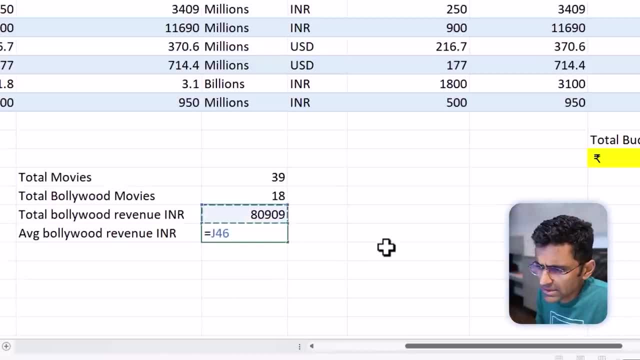 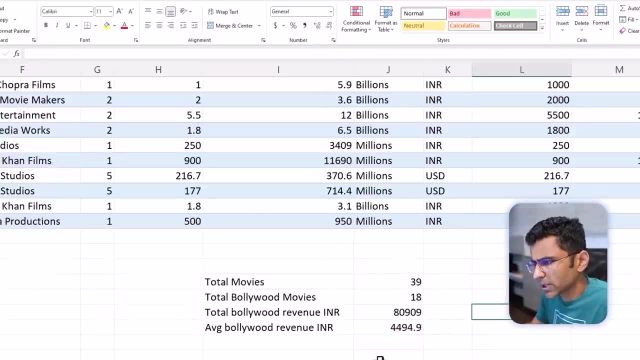 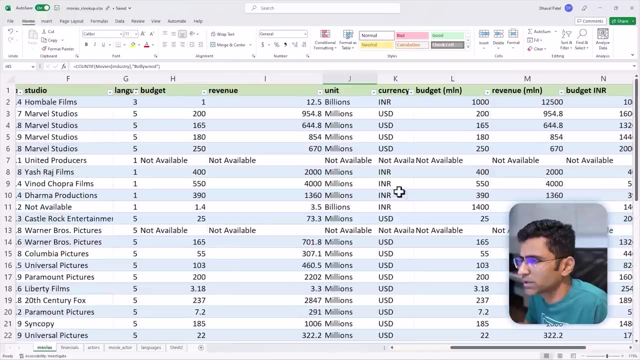 this is million INR. all right, folks, that is understood. that is simple average. we don't know how to calculate. this is simple average between this number and that number, and you can okay. now one question that you might have is: we said 18, but out of 18 movies there was. 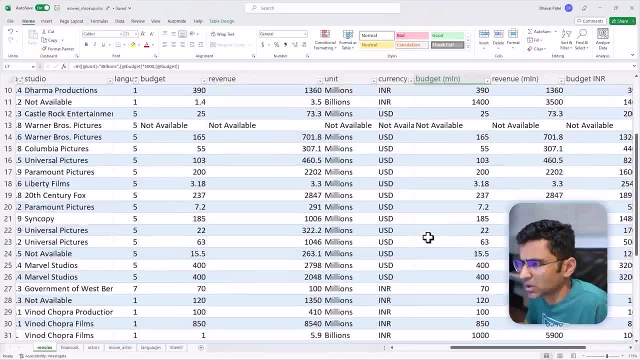 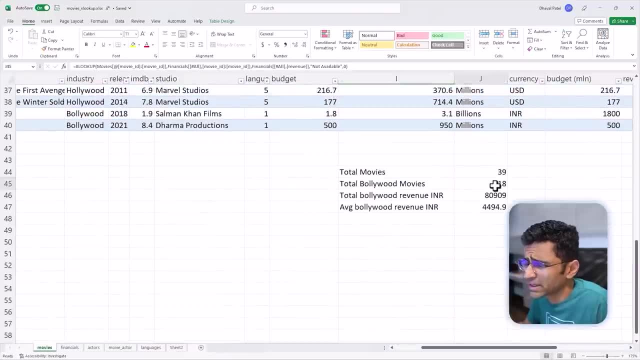 I think a movie which which did not have any data not available- correct, I think it was Sholey. say sholey movie is not available, so actually you should be dividing it by 17, because for one movie data is not available. but I think it was Sholay, so actually you should. 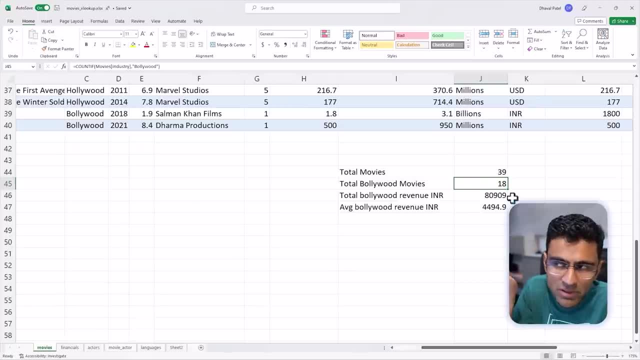 be dividing it by 17, because for one movie data is not available. but I think it is actually not available. but if I take a look at a number and then we can see that the number is no, it actually depends on the situation. you may think 17 is the right answer, so average will come out to: 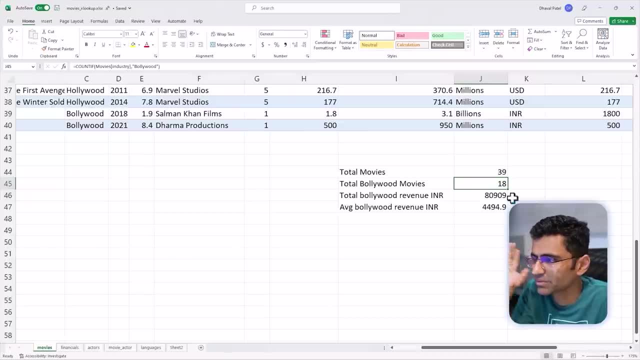 be little less. but i think it's okay just to keep things simple. will not bother about it, otherwise you can handle that na value. you can either delete that data point. you can put mean or median depends. so you have to discuss with your business manager and come up with the conclusion. but 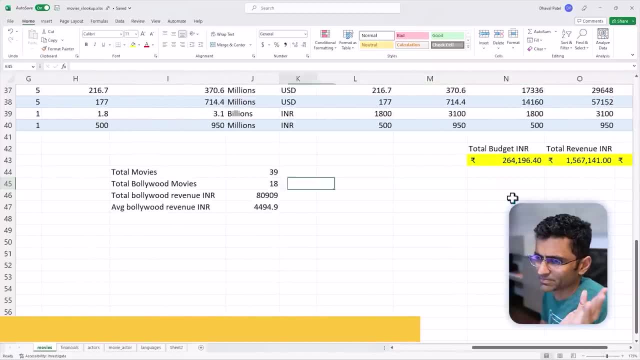 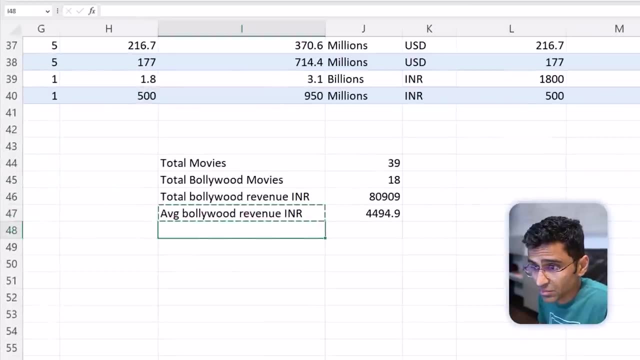 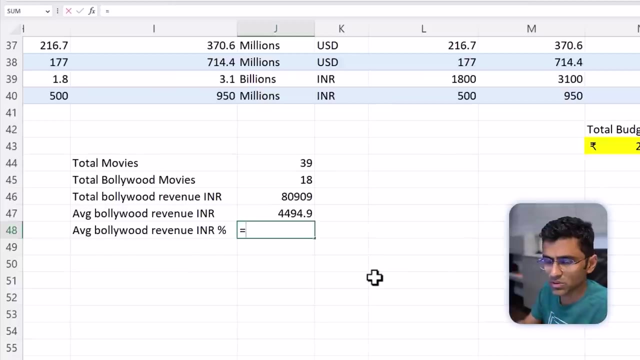 we want to keep things simple, so i'm gonna just just say: okay, this is the total number and you can say average bollywood revenue percentage. what is my percentage average bollywood revenue? that would be okay. so you have to say total bollywood revenue divide by total revenue from. 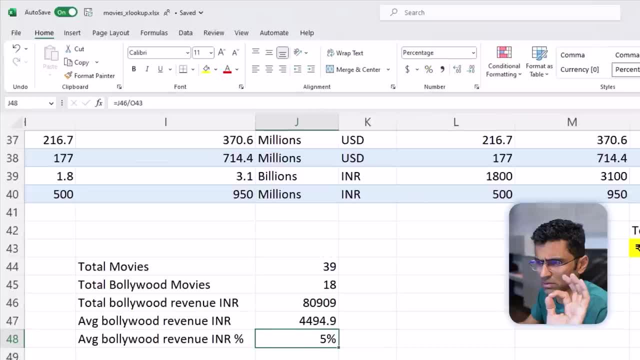 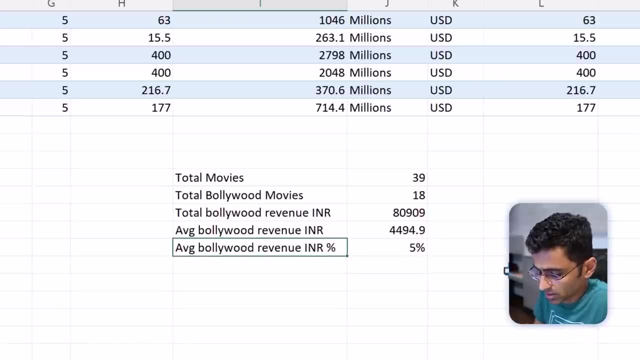 all the movies and if you can take percentage, five percent, okay, it is quite less here. so this number is basically your percentage bollywood revenue, percentage revenue from bollywood with respect to all the movies. and this is five percent because, first of all, our data set is not complete. we don't have all the movies, it's just a small sample and 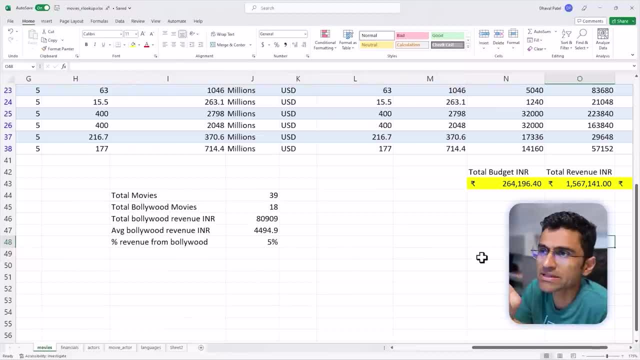 the second thing is: you know these hollywood movies. let's say, if i'm watching the hollywood movie in us, usually it earns more money because it's dollar, and dollar gets converted to 80. so naturally, hollywood movies make more money. all right, that's all we had for this video. in the next video we are going to 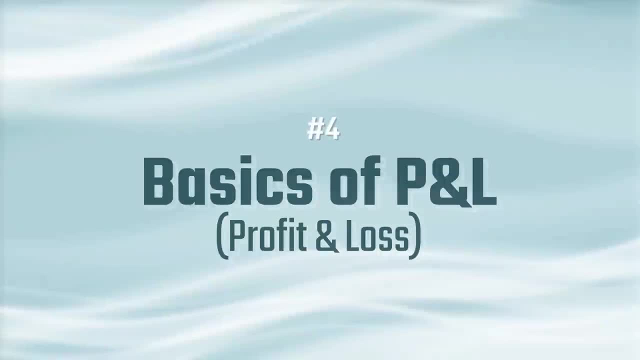 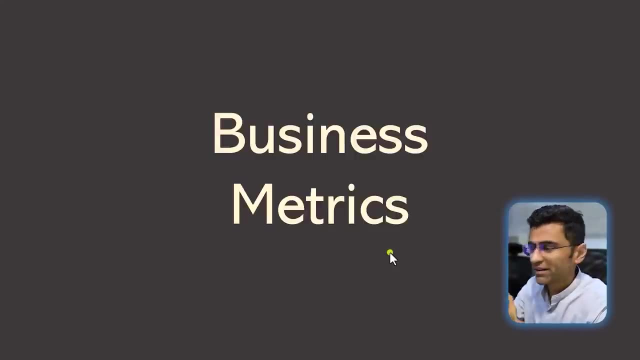 cover basics of profit and loss statement. we are going to discuss some of the important business metrics in this video and we will use marvel studios as our case study. you all probably watch marvel studios as our case study. sell it. its going to matter while possible. 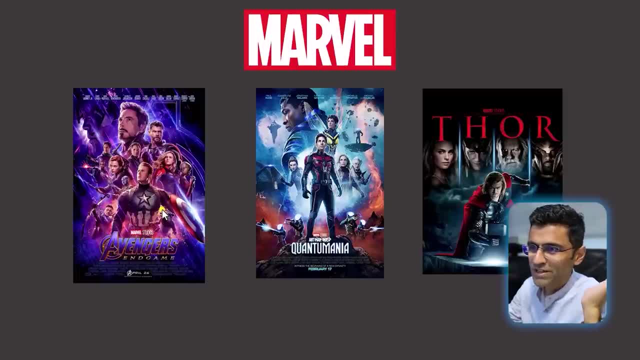 according to dur 봐's guards. they also promise to reduce mm over and over. users- also sennor and including Korean brands- need to be careful when selling movies. they also have some wszyscy to make up. you all probably watch Marvel movies. they are into this business of making movies and it's a. 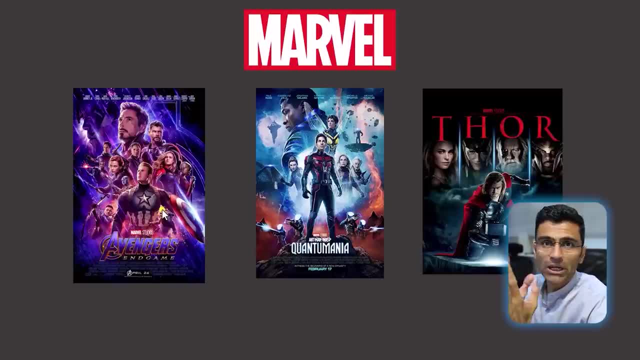 business, so they will have their own profit and loss statement. and when I say profit and loss statement, what it means is they have to spend certain amount of money to make these movies, which is called movie budget. then they release the movies. obviously, you go watch movies and it. will generate revenues for the business, so that is called revenue. so there is a revenue. then there is a cost, which is your budget, and if you subtract the expense from revenue, what you get is profit. so that's a basic definition of profit and loss. if expense is more than revenue, then you get loss. 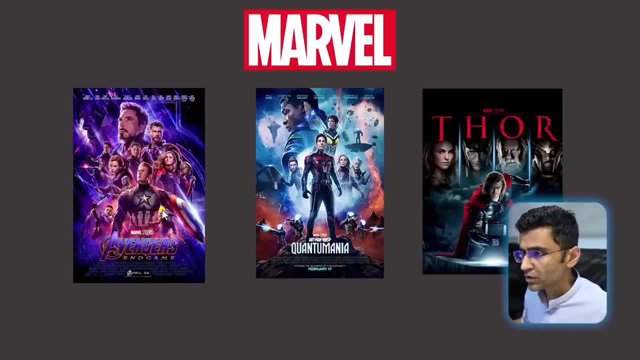 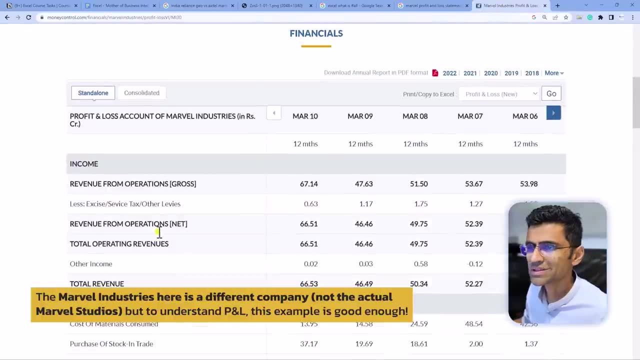 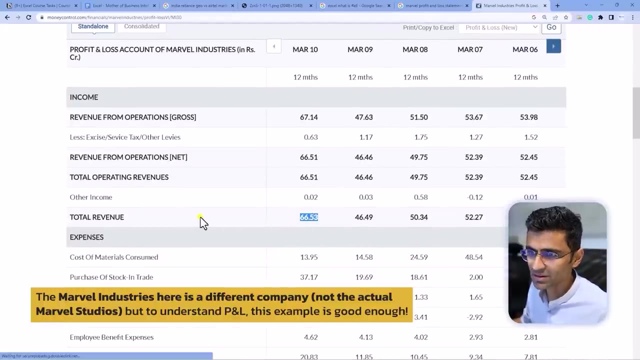 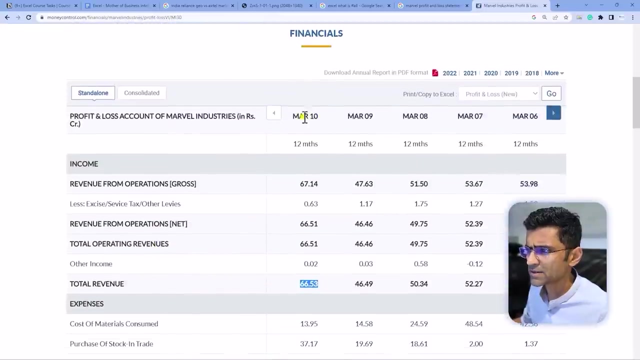 if it is less, you get profit. so if you google marvel profit and loss statement, you will find various websites where you will see a complete statement here and here. what this says is: 66.53 was the total revenue. this is probably either million or billion dollars and this is the. you know March 10 as of 12 month time period, so that's like the. 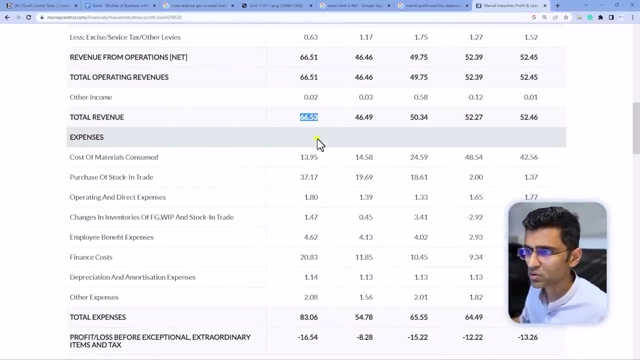 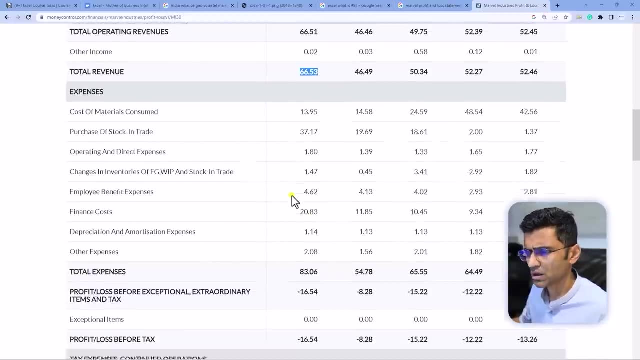 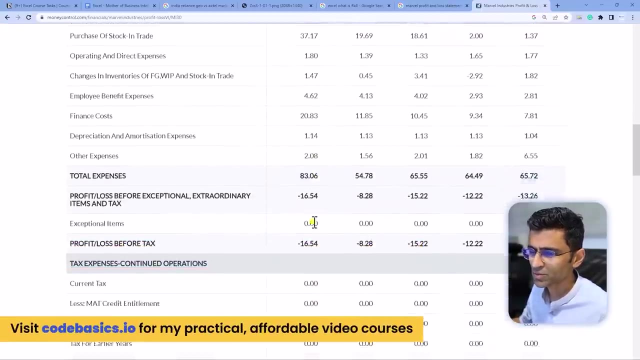 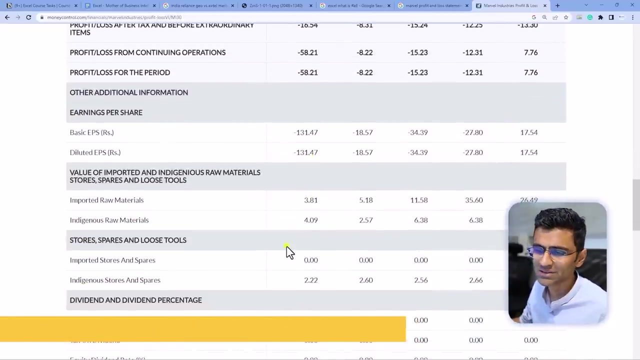 duration. then you have expenses. so from revenue you will subtract all the expenses- see cost of material consumed, financial cost etc. and this is your total expense. and since the expense is more than your revenue, you will have loss, so see minus 16- and then there will be taxes and after you deduct taxes you will get net profit. 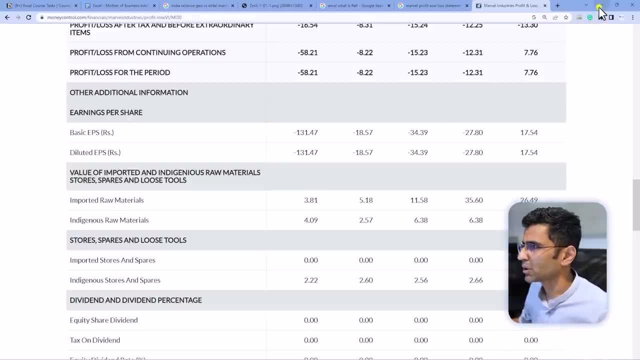 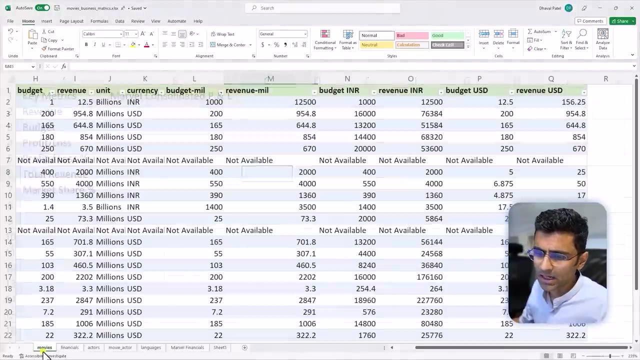 so that's a detailed statement, but what we are going to do is use a very, very simple statement. so we already have the movies data set with us, okay? so let's, let's open up the movie budget. so let's open that here. and in this we have the information on marvel movies here, see marvel. 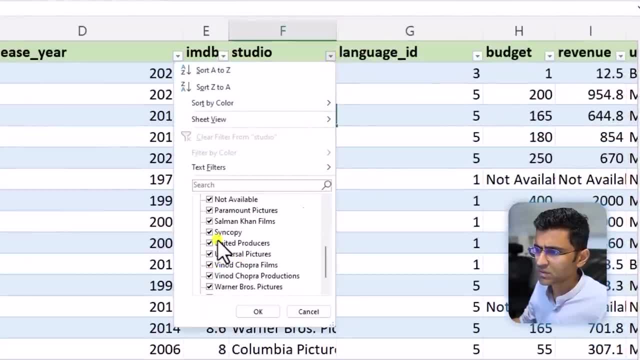 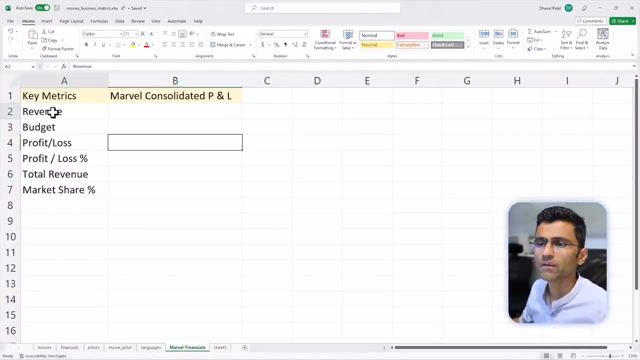 studios. so if you filter things by marvel studios, you will get all the marvel movies and we are going to create this marvel financials, where we will have marvel's revenue, then budget, profit and loss, profit and loss in percentage and so on. so we are going to create all those metrics here. 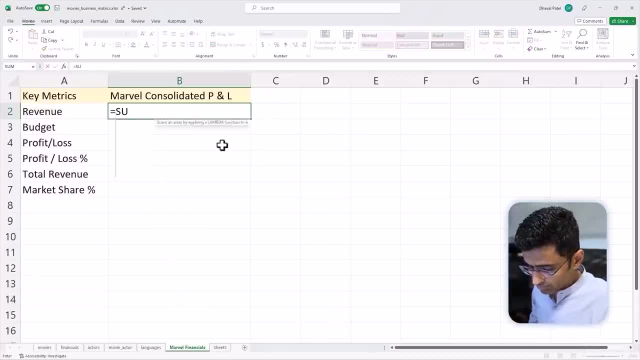 okay, so let's pull marvel's revenue. so obviously you can use some formula and in some you can go to movies table and if you do revenue usd, you get total revenue. so this is a total revenue which includes movies which are not from marvel as well, but you want to include only marvel movies. so 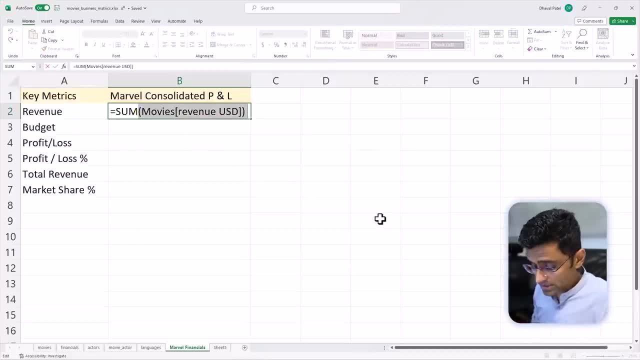 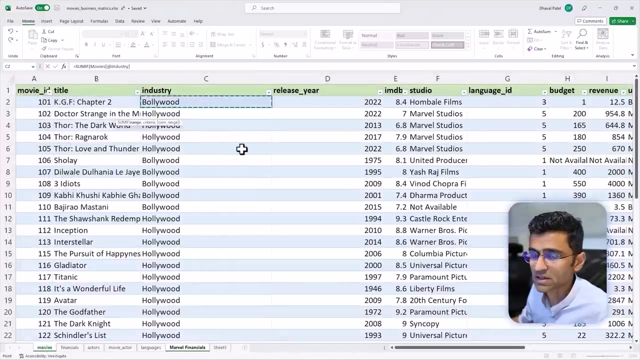 we have looked at this before. you need to use some if formula where you're saying: if the movie studio is marvel, then only sum the revenue. so here, first you are specifying a range so you can go to movies and you can specify this range because, uh, okay, i think studio, because you are. 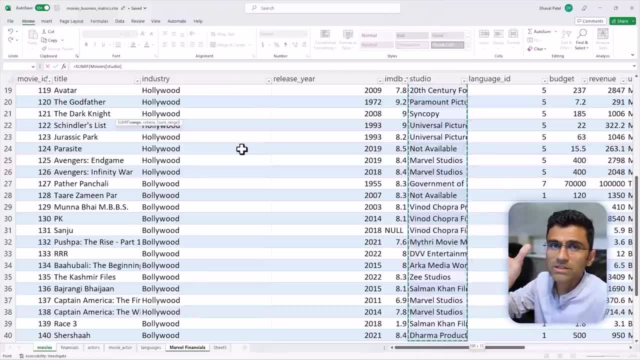 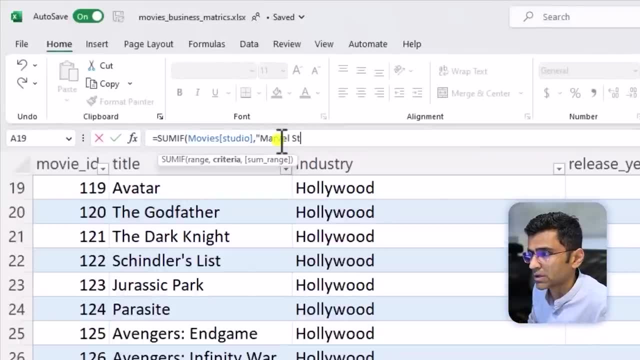 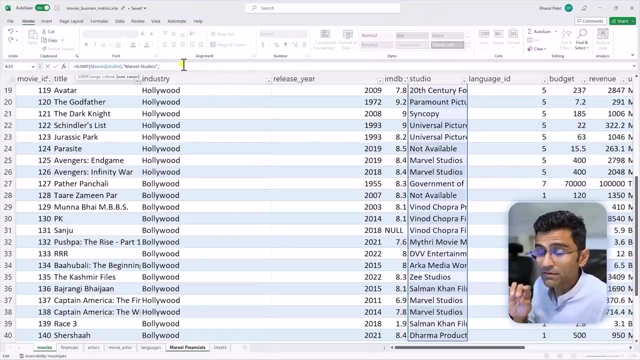 filtering based on the studio. so in some, if the first column is the column on which you're filtering, okay, so that is your studio. and what is the filter criteria? marvel studios: see marvel studio. you see marvel studios here. so that's your filter criteria. and after you have filter, what do you want to sum on? 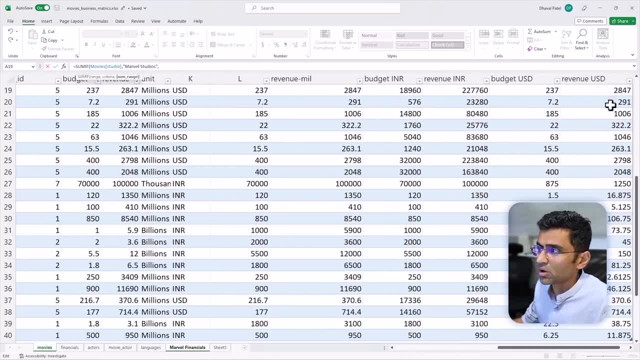 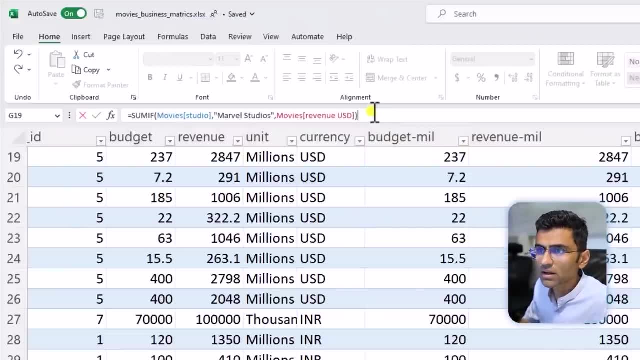 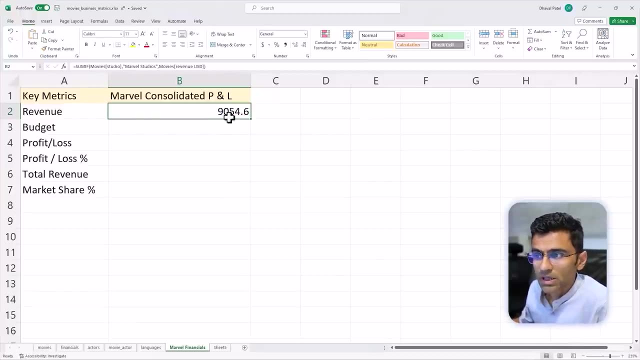 well, you want to make a summation on this thing, which is revenue, usd, so you're going to select that, okay, and finish that, and that's your total millions of dollar, okay, so this is 9 million dollar in total. that's your marvel's revenue, if 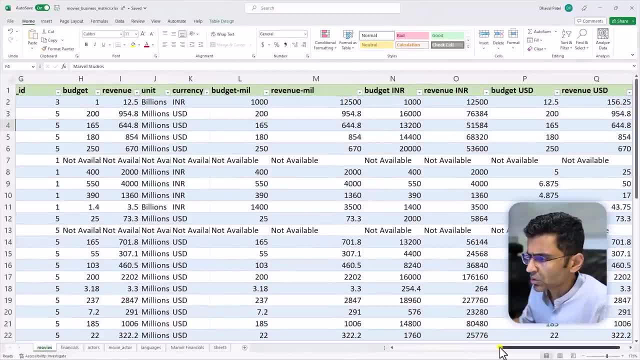 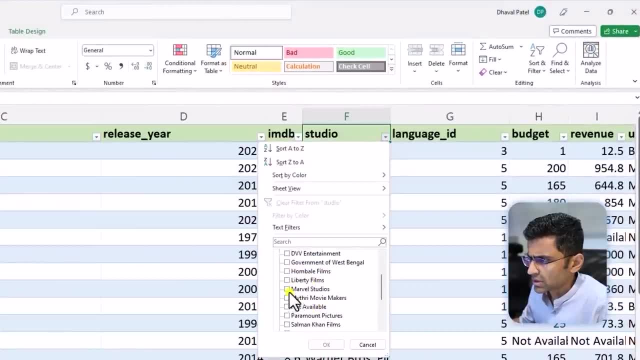 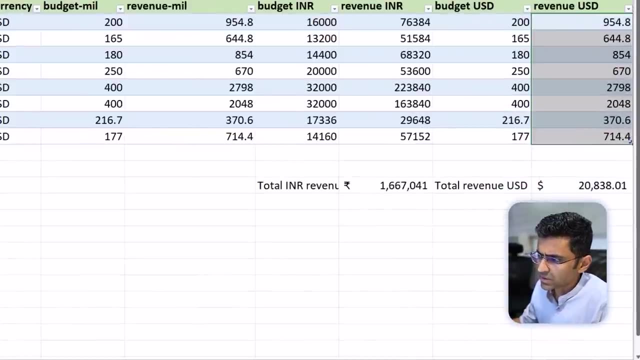 you want to verify anything, you can go to marvel studios. and you can go to marvel studios and you can go to studio here and just filter things out. okay, so i'm just going to select marvel here and i get some eight movies and if you just you don't select these numbers, you'll get nine zero. 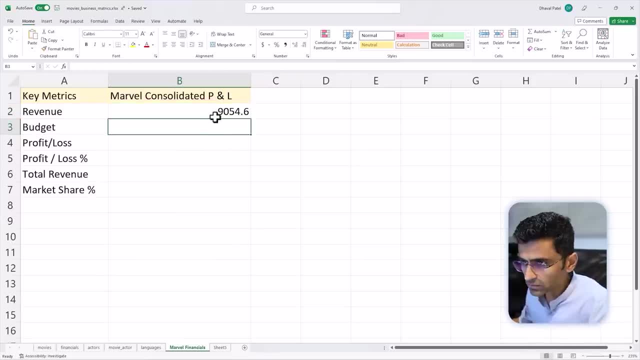 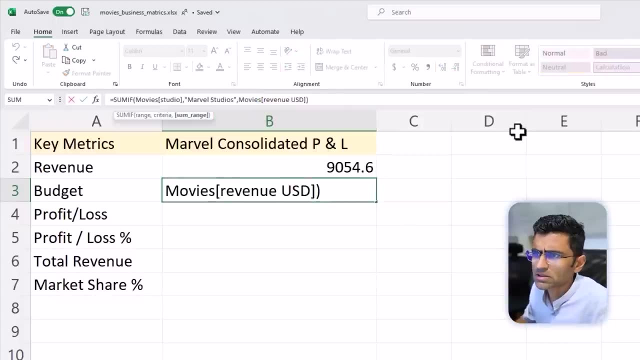 five four, which means our number is correct. see nine zero five four. now you can do the same thing with budget too, so i'll do control c, control v, and here, instead of revenue usd i will budget USD. okay, so you get this now. folks, just be careful when you are doing. 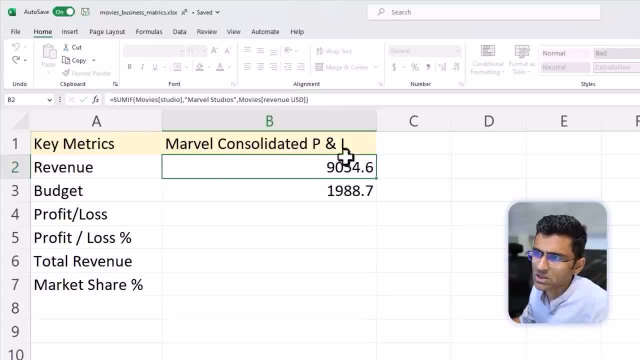 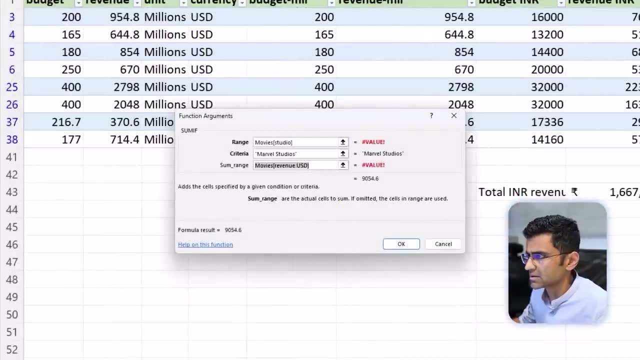 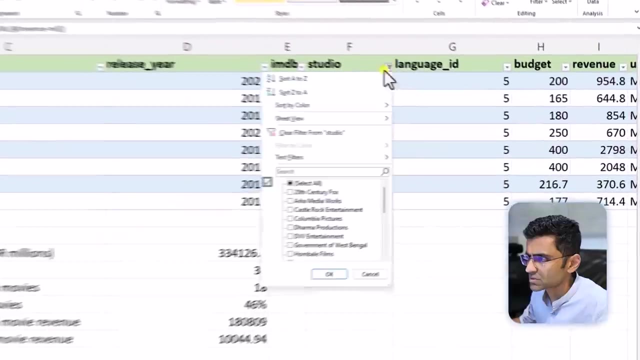 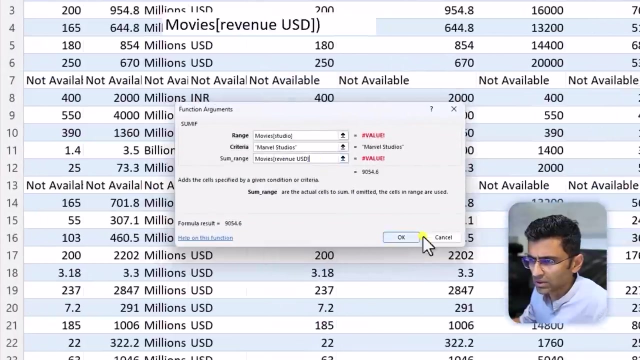 these formulas: see. right now I'm supplying movies. revenue: USD if see in the last one I selected. okay, let me just first clear that filter because, if you remember, we have a filter on the studio. so I'm just gonna clear that and then go back to this one and look at the third column. see here, when you select this, you 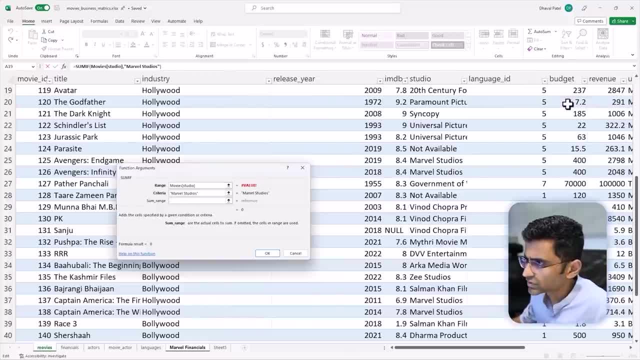 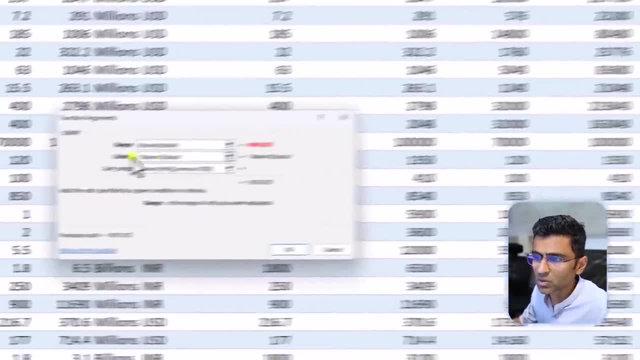 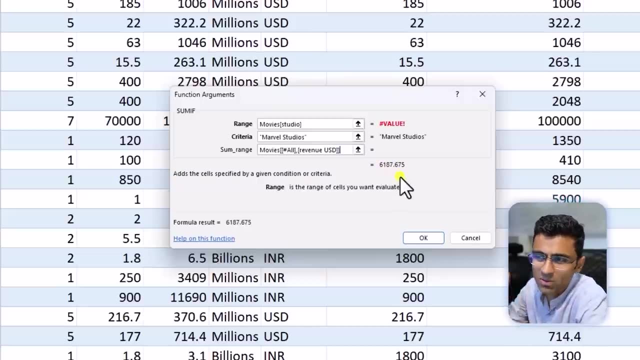 get movies revenue USD. but if you select the whole whole column, including header, you get movies all revenue USD. in that case you can get a wrong number, see six, one, eight, seven. I actually don't know why this is happening, but I have seen this wacky behavior with excel. 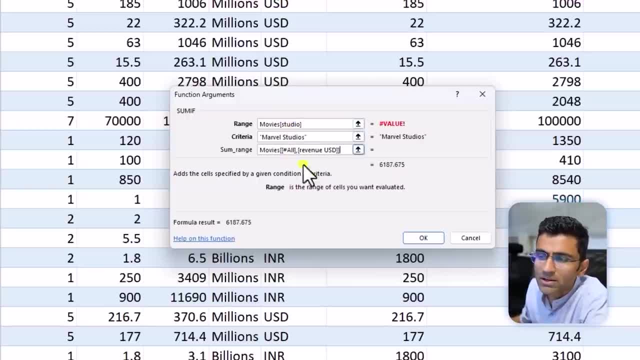 so make sure you're consistent. if you have all here and all here, it will work okay, but you need to be consistent in terms of range and some range. so I'm just going to delete it and just select- see select from the first data row, don't go. 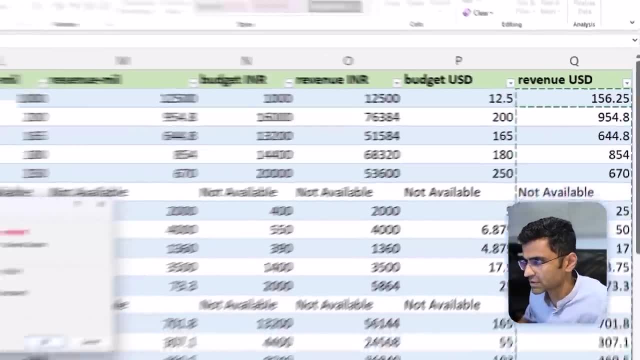 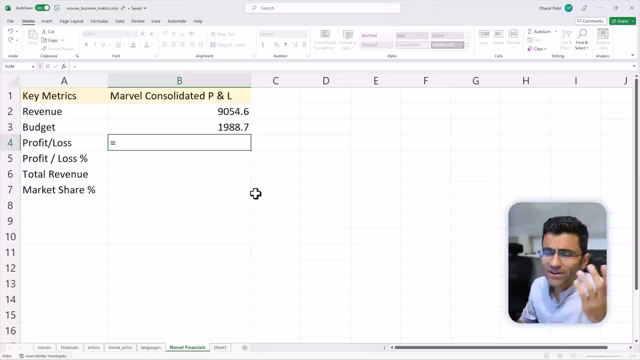 from here, otherwise it will include header. so select from first data row, go all the way, hit enter and then it works. okay, okay. so my what is my profit? profit is simple: it is revenue minus budget. that's business profit. if my budget was more than revenue, then I would end up in a loss and in the financial statements. 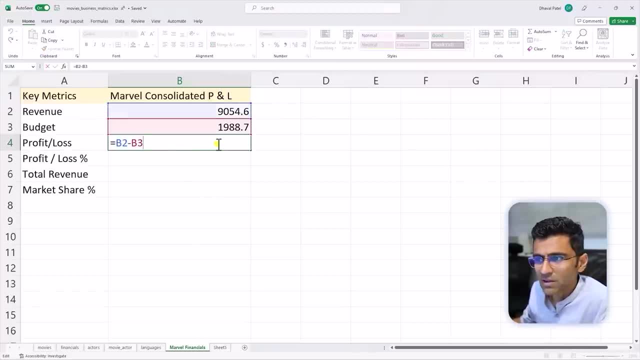 they just say profits, less loss, and whenever the number is negative, it is common understanding that that means it is a loss. okay, now what is percentage profit loss? well, this number is on. number is. on which baseline should I use? revenue is my baseline or budget is my? 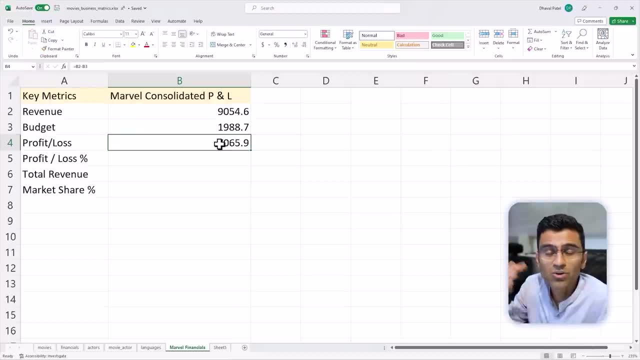 baseline? well, it's it's budget. so it's like you are Marvel movie producer. you spend hundred million, so that is your budget. and let's say, if you made a profit of fifty million dollar, that's a fifty percent profit. but that is always calculated with respect to budget. therefore, I will say this: divide by this. 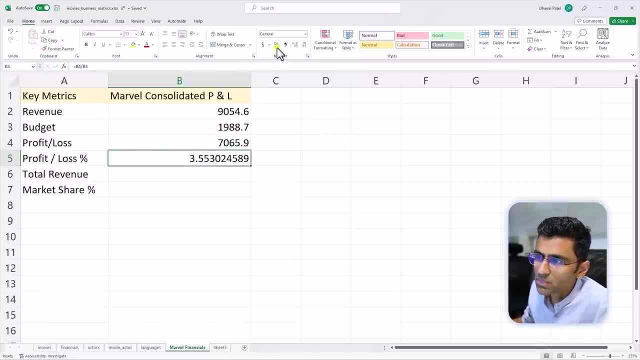 because that is your budget. and if you convert this to a percentage, which I can do by clicking here, you get amazing three hundred and fifty five percent profit, and this is based on the limited data that we have. this is not the real Marvel profit. okay, this is based on our data. 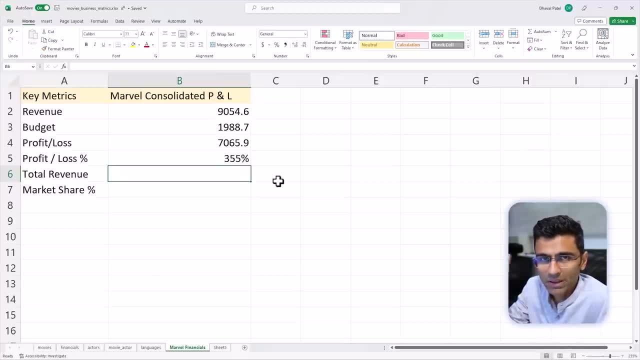 set. if you want to look at real PNL statement for Marvel, you can google and find it out. okay, so that's my profit. now I want to know market share. so what is market share? so this is market share and it's a common thing in the market as we are. 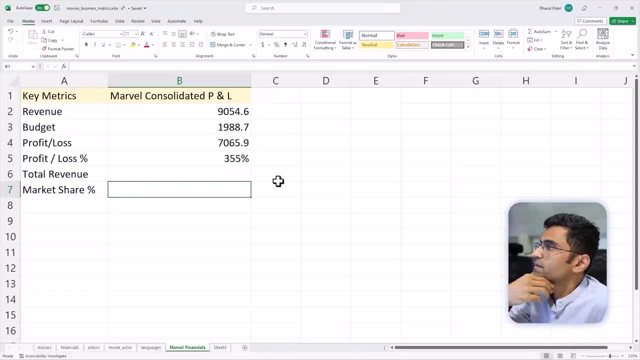 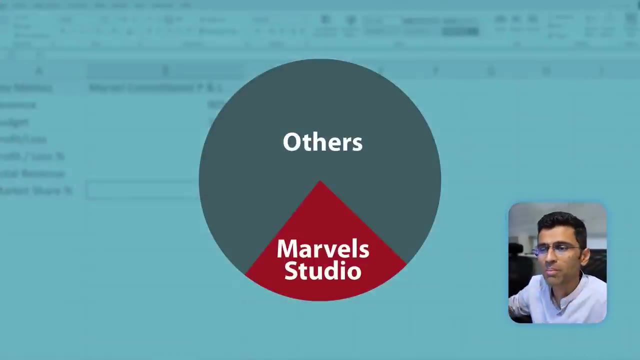 so market share is basically: if total Hollywood movies revenues, let's say, 100 million and Marvel is 20 million out of it, then Marvel's share is 20 percent. it's like a pie chart. in this pie, how much is the revenue from Marvel? okay, so in order to calculate market share, you need to first calculate. 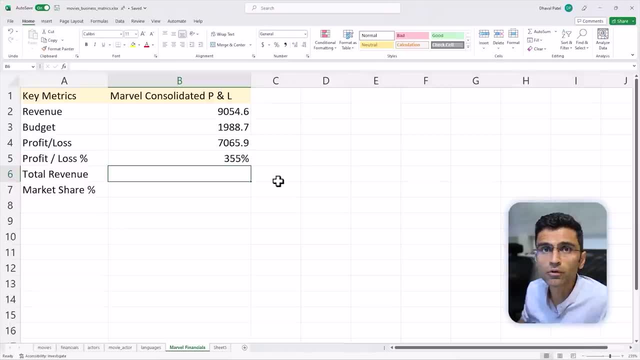 total revenue of all Hollywood movies. okay, and that you can calculate using some, if function once again. so I can say some if I don't need to even now look at the movies table because you know, I know that it's called movies and when you are saying Hollywood, you are basically 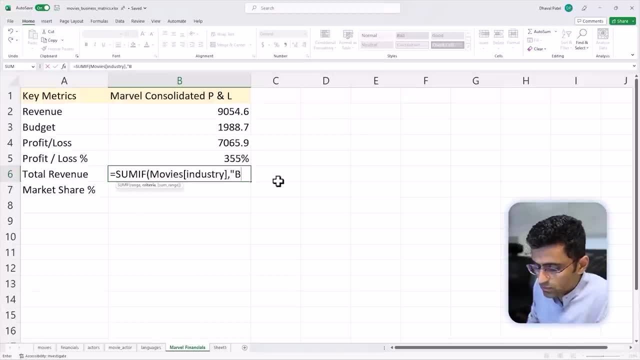 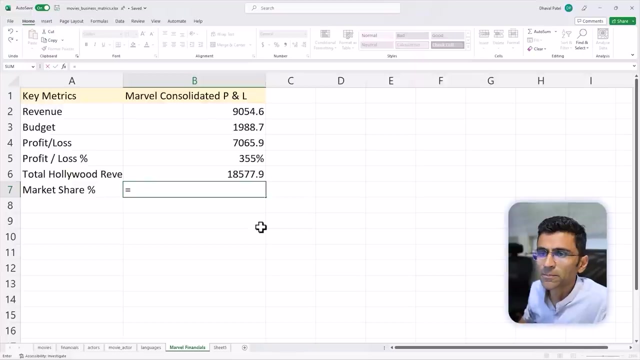 referring to the industry column. so in the industry column, give me all the records, you which has Hollywood in it, and then sum the revenue. so revenue is present in which column? this one, correct? so this is total Hollywood revenue. I should say total Hollywood revenue and my market share would be what is my Marvel's total revenue? 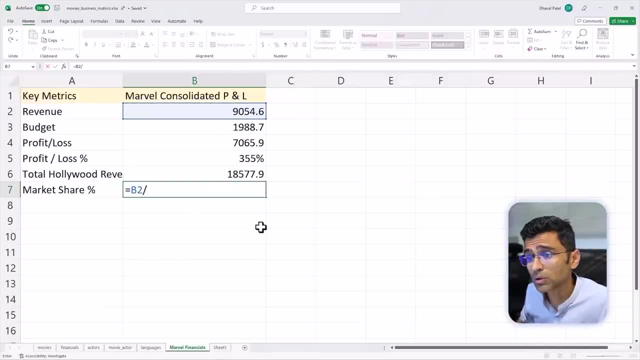 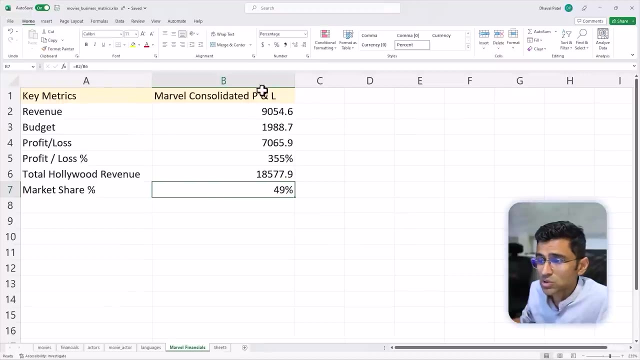 Marvel's total revenue is this. and what is total revenue is this? and if you convert that to a percentage, it is close to 49. I mean you can increase the decimal and you get the better number, but it's okay, I don't want to have any decimal. so total market. 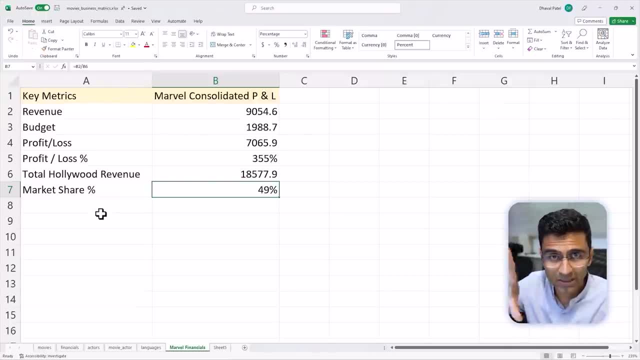 share of Marvel in our data set- okay, not in reality in our data set is 49 percent, which means 49 percent of the revenue generated by total Hollywood industry is coming from Marvel's total Hollywood revenue. 49 percent of total is coming from Marvel. okay, I hope folks just think about it. this is common sense. 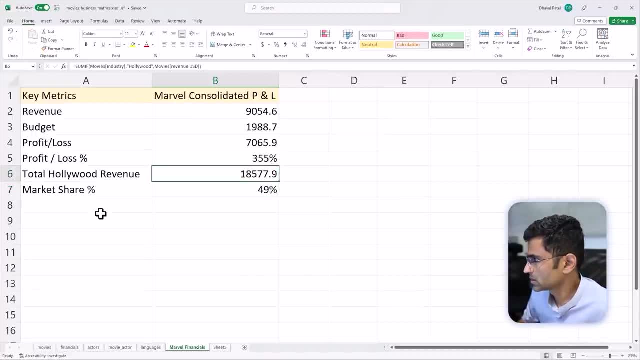 so you should be, I think, able to get this pretty easily so we can generate this. inside that Marvel is almost half of the Hollywood revenue. I know in reality it is not, but based on this data set, see, you are generating this, this, this kind of insights where you need to learn how you can. 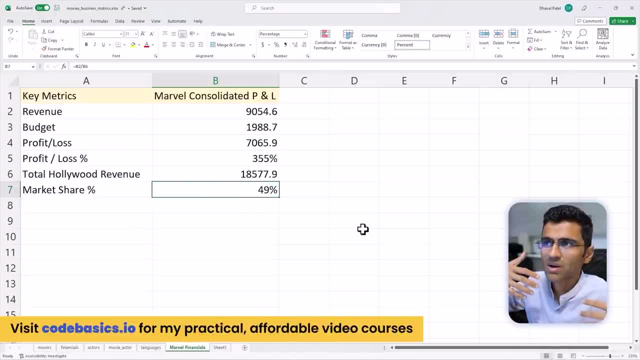 talk in business terms, as a data analyst or as an excel analyst when you're working with other other business stakeholders, or don't use this number. that okay, marvel's revenue is 35 percent. you can say: marvel's revenue is almost one third of the total hollywood industry. or here, marvel's revenue is almost half of. 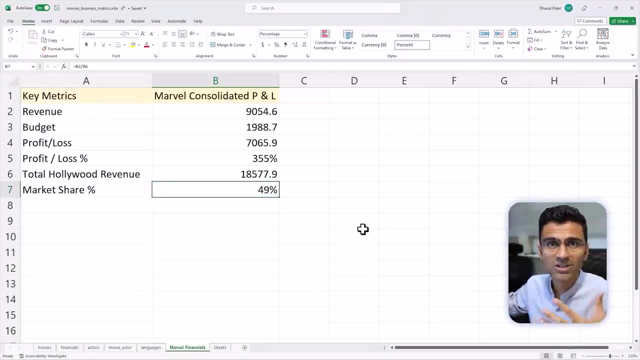 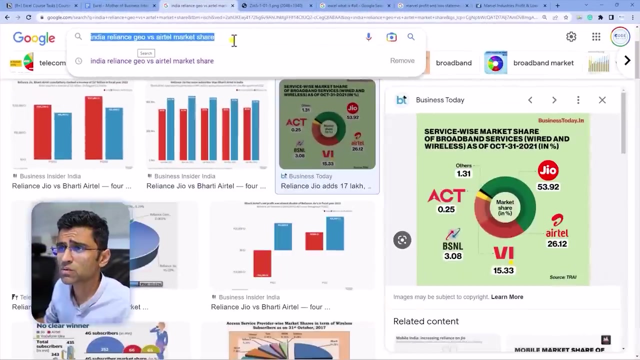 what is generated by the entire hollywood industry. so when you are using this kind of business language, you can do effective communication. so that's very important. learning business communication where you put all your technical- uh, your code monkey behind, that's very important skill to have in terms of market share. i can go to google and say india's reliance geo versus. 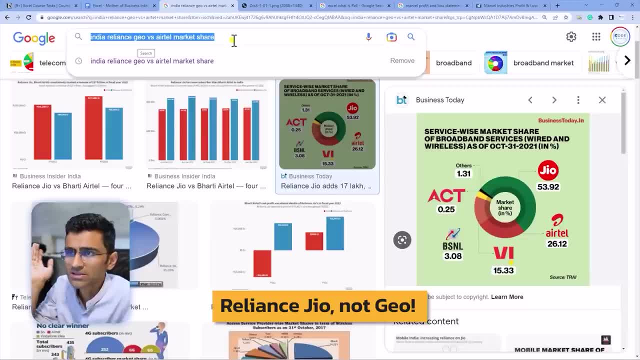 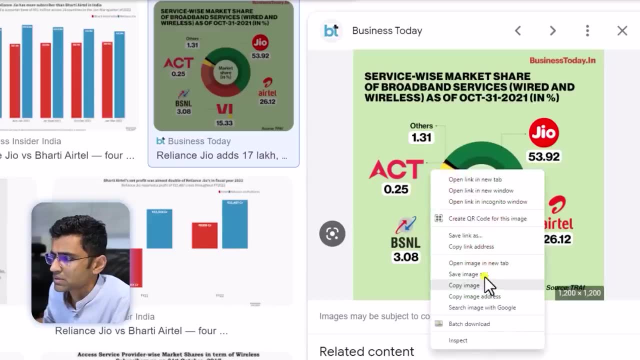 airtel market sales. so in in india there are these wireless companies- reliance, geo, airtel and so on- and see you see this nice picture. so if you open this picture, if you say right click open image in new tab, see this shows the market share. 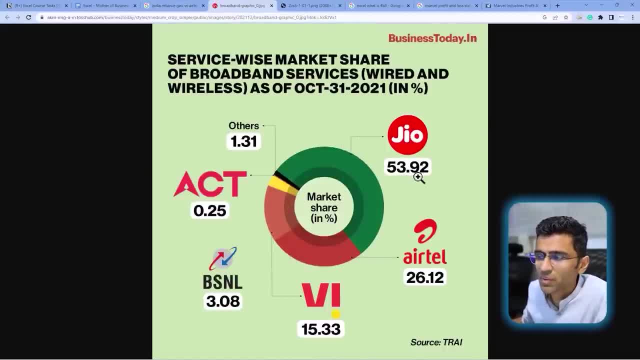 so when they say reliance geo is 53.92 percent market share, now you get it. so you have to take a revenue from reliance geo, divide that by total wireless industry revenue in india and that that's when you get 53 percent. airtel is 26 percent, which means if total wireless industry in india is 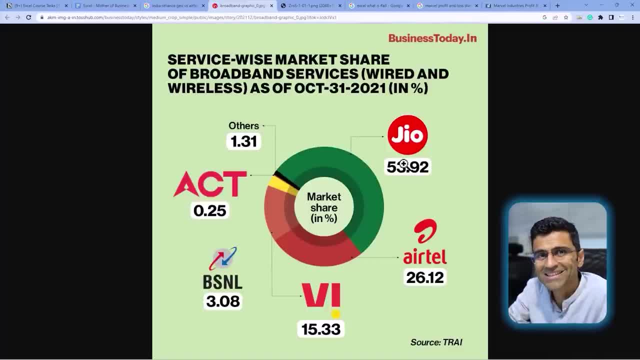 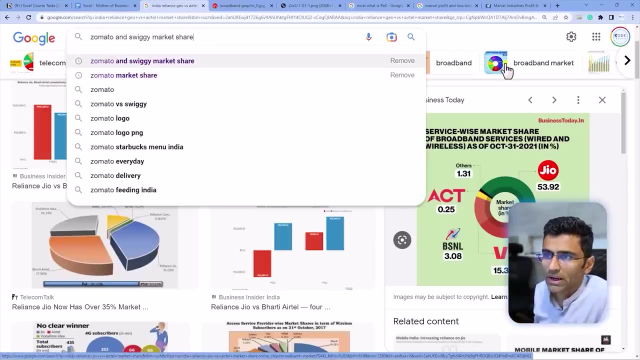 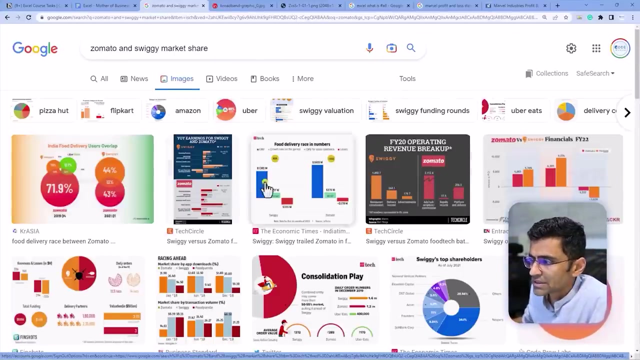 generating 100 rupees revenue. 26 rupees revenue is going to airtel and 53.92 rupees revenue is going to reliance geo. you can do similar analysis on, you know, zomato and swiggy market share. these are like food delivery services in india and you will see. 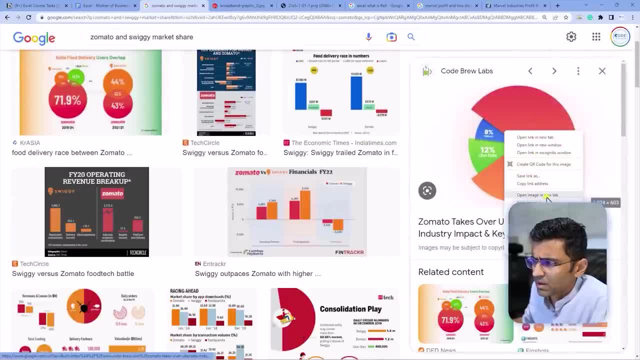 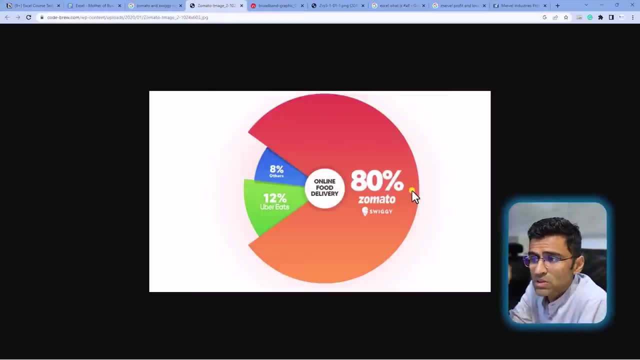 various charts. for example, look at this one open image in new tab here. it says: eighty percent of online food delivery market in india is covered by zomato and swiggy combined. twelve percent of online food delivery market is covered by zomato and swiggy combined. twelve percent of homeless families have food delivery society. so 63% of homeless families actually mostly work for mash, facing unlimited funding, access and employment contracts and paying full living expenses. in india business 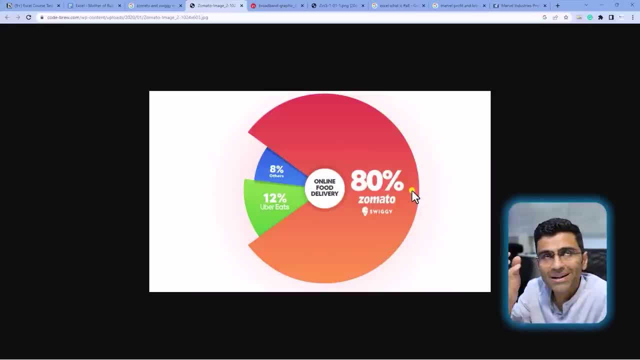 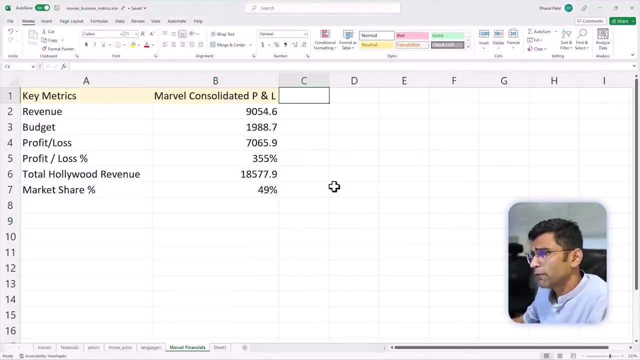 is uber eat and eight percent is others. market share is something which is very important concept, and when you go for interviews for data jobs, they can ask these kind of questions, so it's an important concept to learn. okay, now, in every business, there are always targets. okay, so let. 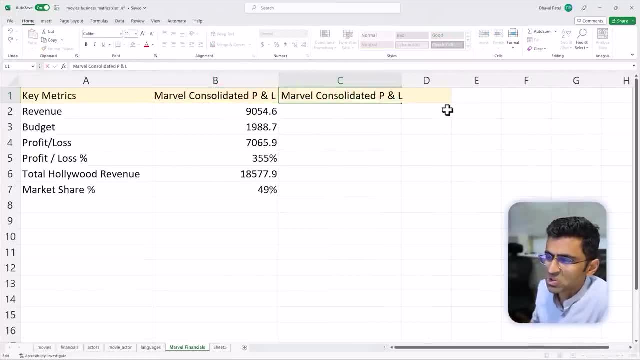 me talk about target. so if you're looking at, you know any financial statement or any, if you're doing any studies. when i was at bloomberg in bloomberg- uh, i used to work in earning estimates team, where every company would have their earning estimates and when the actual numbers come, they 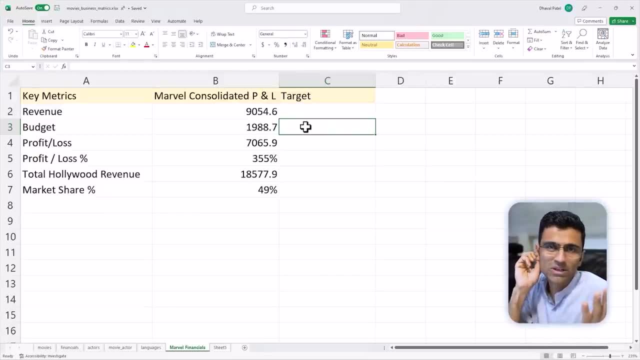 will be different. earning estimate is basically your target. so let's say you're trying to hit 100 million revenue, but actually you hit, in reality you get only 80 million revenue, which means you are 20 million dollar behind, behind the target. okay, so let's say, for my marvel, someone set a target of 8 000 and, by the way, i'm 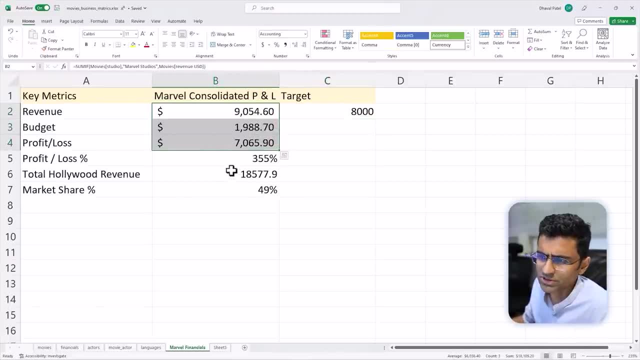 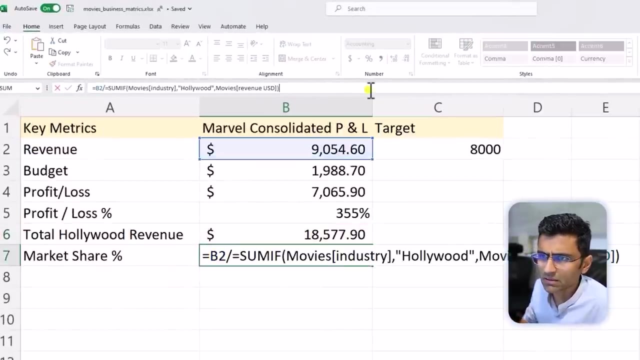 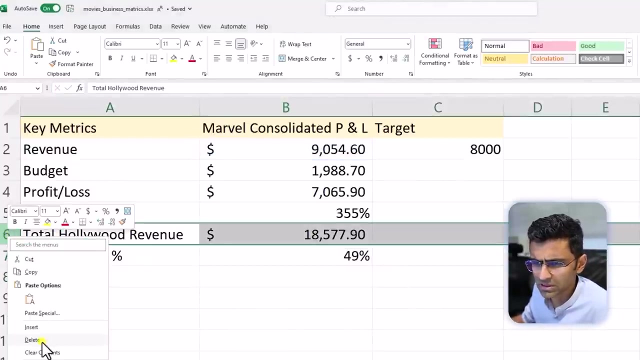 just going to convert this into just i'll put the dollar sign so that it's very clear and you know what i can. i think i don't need to have total, however, revenue here i'll just say ctrl c and here formula. that way it is more compact. so let me just delete this row. 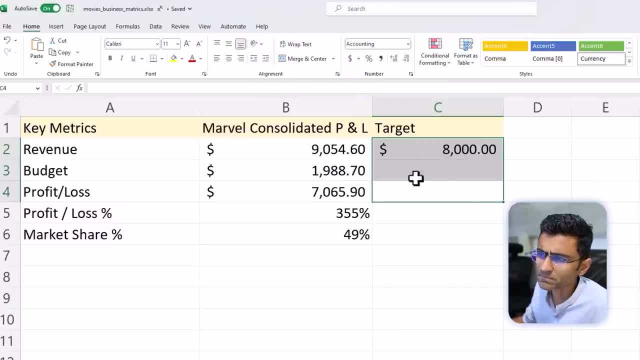 okay, and all these three rows also. i want it to be in dollar. and let's say, my budget was 2000- okay, and my profit goal out of my 2000 budget was, let's say, six thousand. okay, and my profit percentage was obviously this, divided by this: 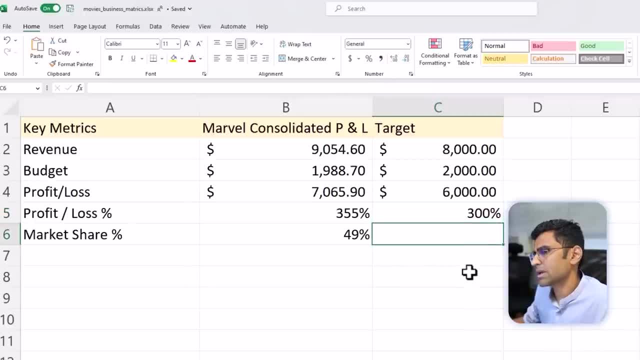 percentage. okay, and let's say i wanted to capture a total of 55 percent market share. let's say, if that was my goal, okay, so i can say 55 percent here. so this is the target which is set by business in the beginning of the year. 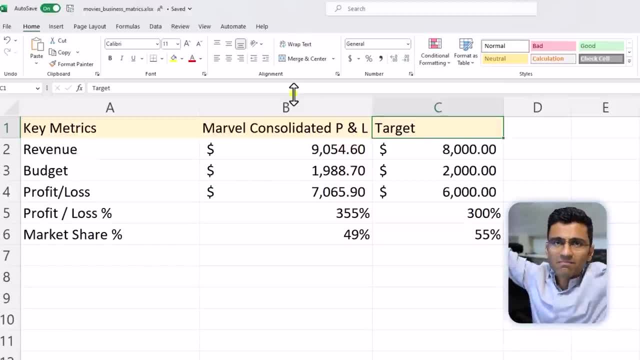 before the business cycle starts, they will say, hey, this year has started, these are my targets. okay, in my own company- right now i'm sitting in, uh, my own software company at lick technologies, and we have business targets and when the year finishes, we try to compare the targets with the. 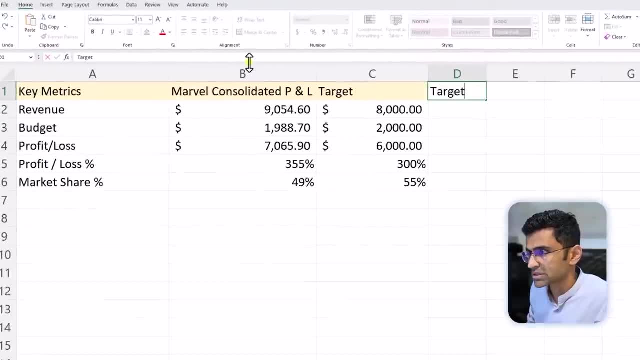 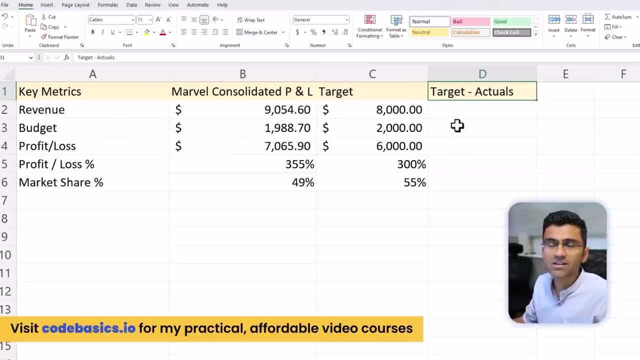 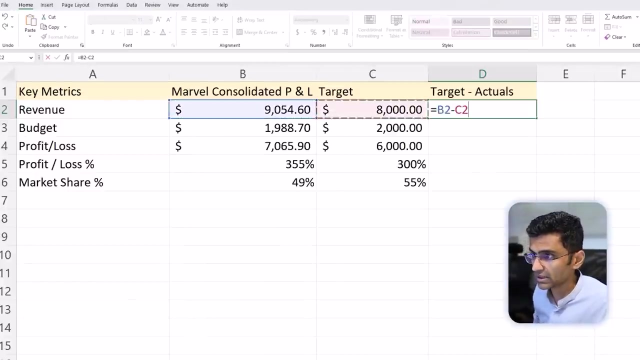 actuals. okay, so here you will say target minus actuals. so what is actuals? actuals is this number, the reality, and target is whatever target you set at the beginning. so target was this? in reality, you got this target. was this actually? you know what? in reality, you hit this and this is my target. 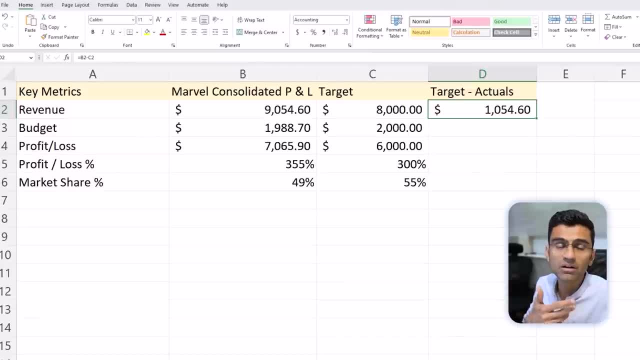 so you achieved, uh, 1000 million dollar above your target. that's what this means. okay, so your budget was this and your actual profit is this, and your target was this, so you achieved, once again, one thousand million dollar extra. i can just change it so that these numbers are different. okay, and 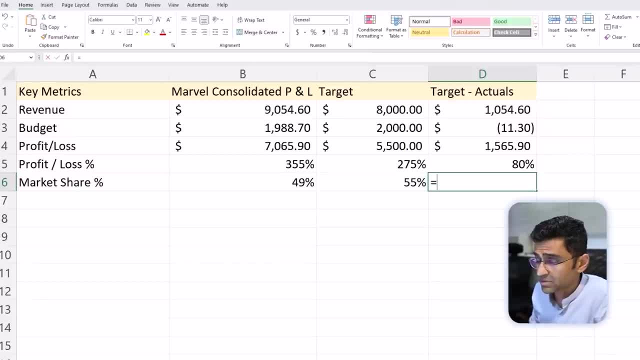 percentage-wise, you achieved 80 percent gain more. okay, because that is your profit. but market share wise, you achieved 6% less. so your goal was to get 55% of the entire market, but you got actually 49. so it is 6% less, but in terms of 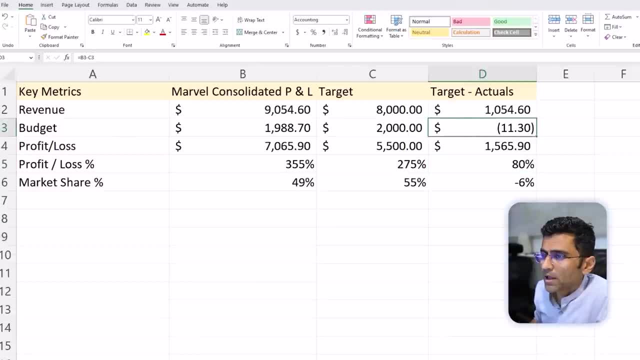 profit. you achieved 80% more profit. okay, in terms of budget, your budget was actually- you know this- this particular number should be, because this is an expense, we need to reverse it. so I expected I would spend 2000, but actually I spent 11 million dollar less, so actually it's this positive thing. 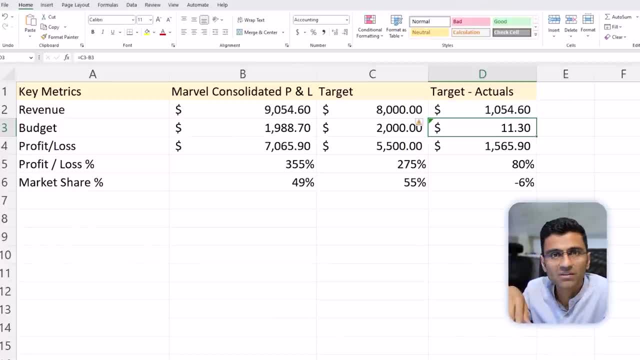 I spent less money, okay, or I mean, it depends how you are interpreting it. by the way, you can also do this one as well. see, whenever number is in bracket, it means it's negative. so in any financial statement, whenever you see any number in a bracket, that is negative. you know, that is just a general. 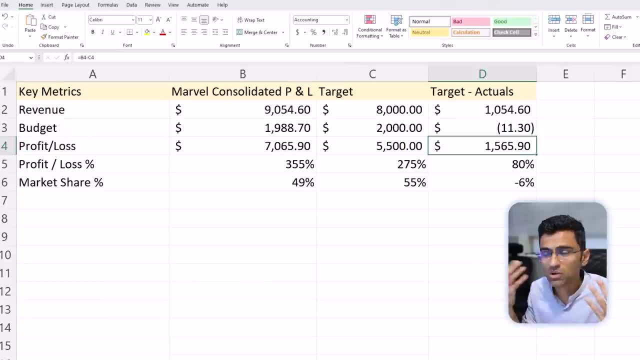 accounting, a convention when it comes to company's financial statements, so you have to remember that. so here this: this factor, target minus actual. it actually shows how you perform overall and sometimes you know the bonuses that people receive- bonuses that sales managers and engineering and marketing team receives- are actually based on this number. you know: are you achieving your targets? if you're, 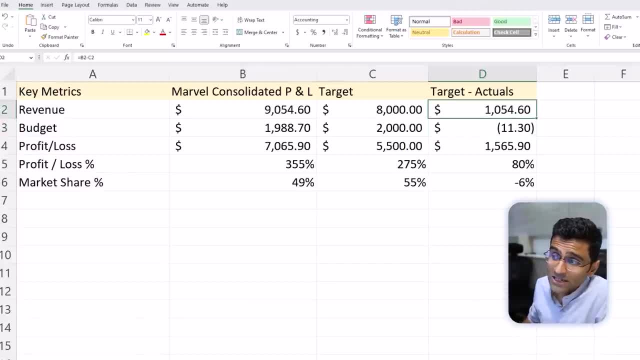 achieving your targets. how much above your your target? let's say I went 1 billion above my target. they did good, so they will. marvel studios will distribute extra bonus to their employees, actors and so on. but let's say, if they did badly and if this number was negative, then they will do. 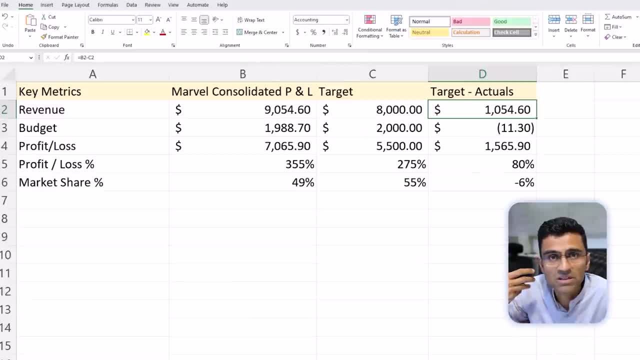 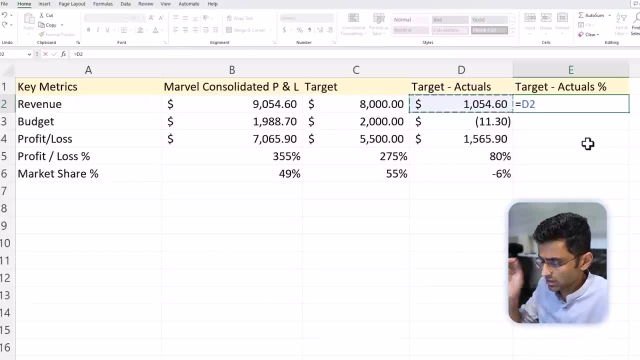 evolution. you know they'll ask questions why this happened. our business did not meet the target, what can we do better, and so on. you can put this into percentage and what this means is the difference that you got on your baseline revenue number is, let's say, 11 percent. 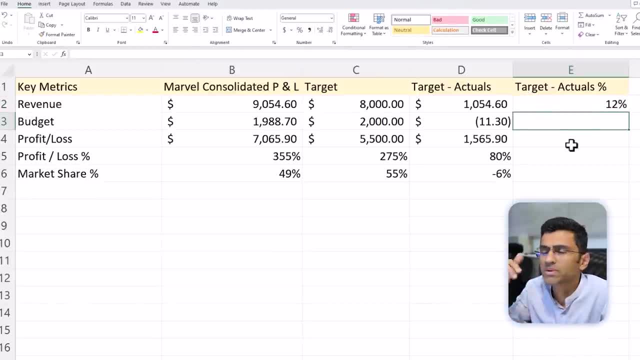 12 percent person, you know. so you got 12% surprise basically. so that's that's a way to look at it. when I was at Bloomberg, when companies meet or beat estimate, there will be this surprise number. surprise means how by percentage, how much you're above. so let's say, if company's revenue target was 100 million, 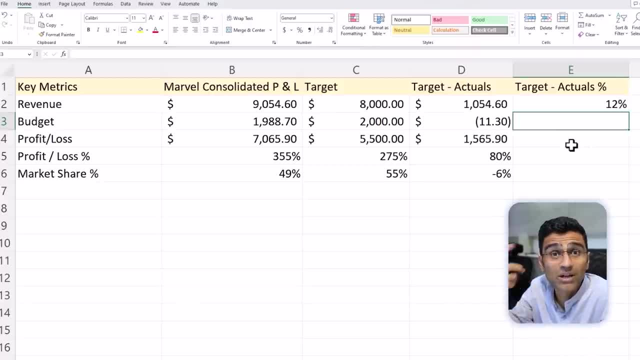 dollar, but they achieve 120, they're like 20% above the target. so that would be, that will be the surprise factor and the stock prices will move based on that number. okay, so this was a very, very simple basic P&S statement. in the future videos we are going to look at much more detail. 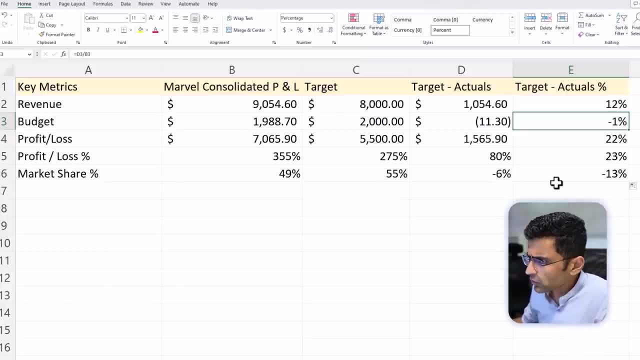 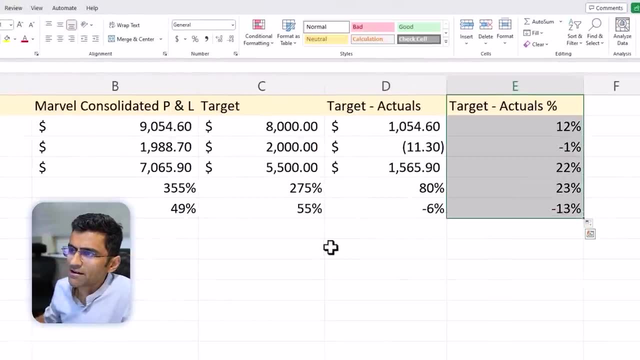 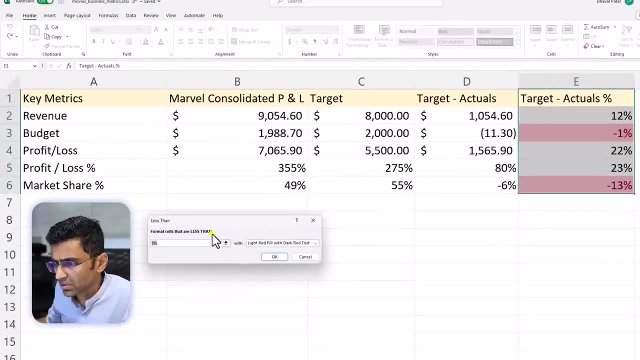 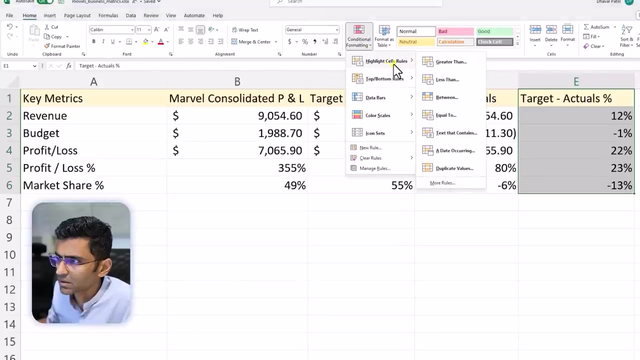 and advanced statement. now, many times, what happens is you want to do conditional formatting and whenever any of your target is, let's say, less than 10%, you want to highlight that. so you can just say conditional formatting and you can say: if this number is less than minus 10, then highlight it, okay. so if it is less than, 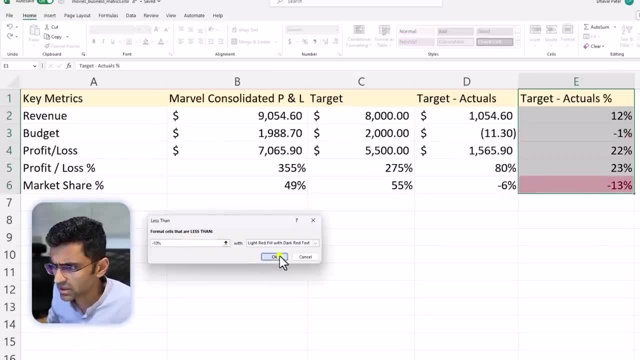 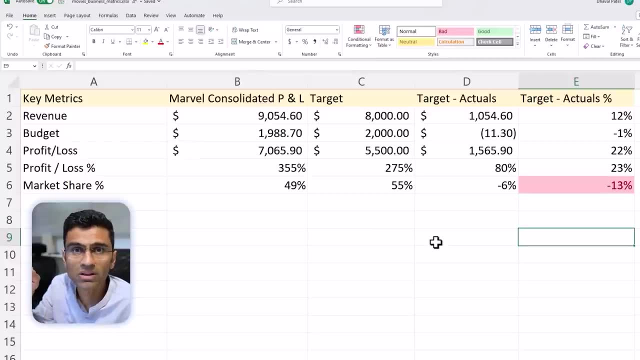 minus 10 percentage, then highlighting. so then you know on which metric you are doing horrible. it's like your threshold. it shouldn't go beyond this threshold. so in terms of market share, you were 13% less than what you were doing. so you can say if this number is less than minus 10%. 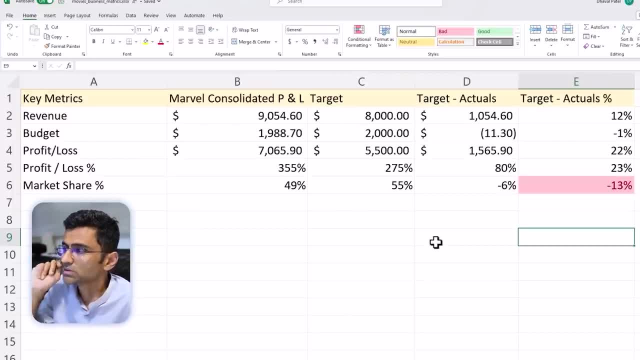 you actually set as your goal. so in excel files, I'm pretty sure when sales and marketing department in big companies they sit together they would have these kind of excel files where they are reviewing their targets and they would have this conditional formatting and they would be reviewing those, you know red highlighted cells carefully. all right, that's all I had. 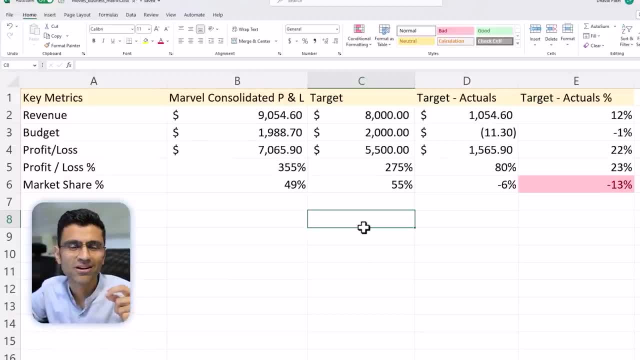 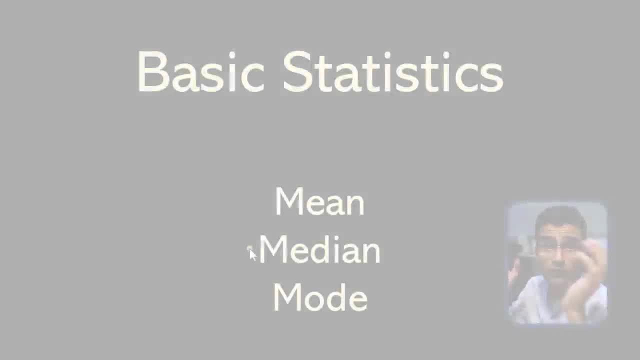 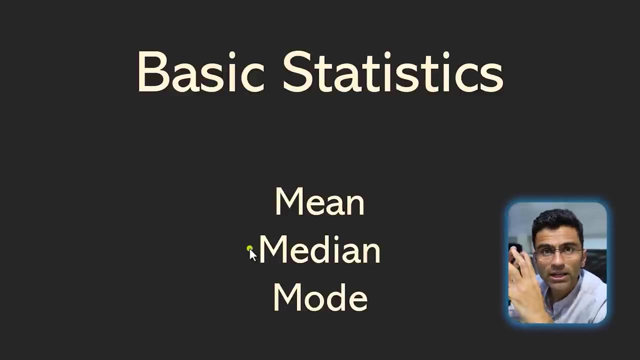 for this lecture. in the next lecture we are going to look at the basic statistics. now we will talk about basic statistics, especially mean median mode. remember that you can do 80% of your data analysis work using 20% basic statistics, so you don't have to know advanced topics such as 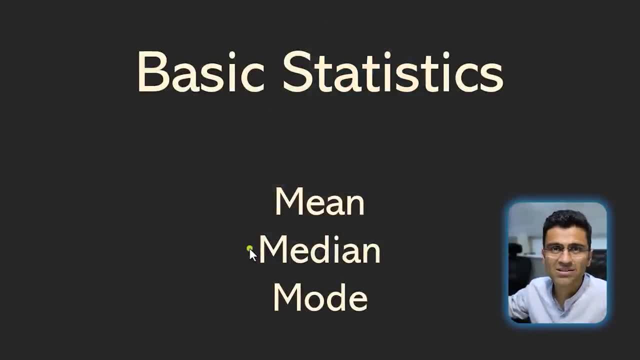 hypothesis testing, chi-square test- all of those things are needed if you're targeting data scientist career. but if you're targeting data science career, you're not going to be able to get 80% of your work done. so let's talk about mean and median first. I will use an example. let's say 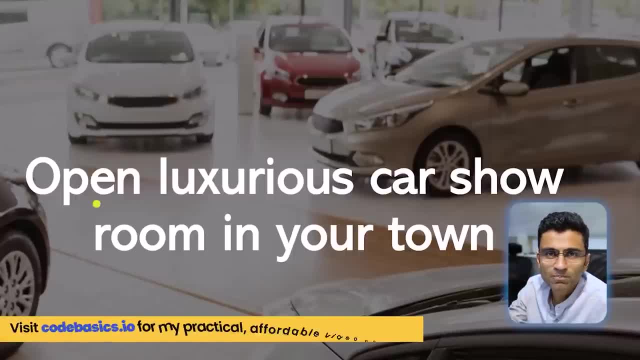 you want to open luxurious car showroom in your town. now, before opening a store, what kind of analysis will you do? well, you will go to town, you will try to measure income level of people and if people are earning a lot of money, then only you can afford to have luxurious car showrooms such as Mercedes or BMW, so doing income. 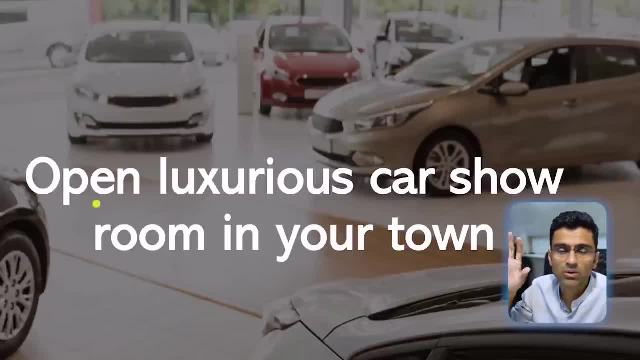 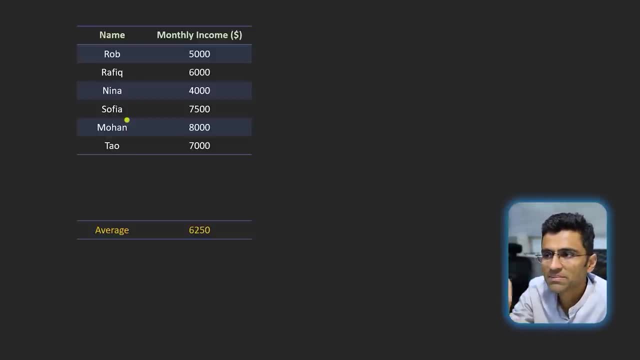 analysis is a usual industry use case when you're opening a new store and let's say, in my town there are these people, let's say six people are living. their monthly income is these many dollars? you can take a simple average. you know right. it's just a sum of all these numbers divided by the total count. 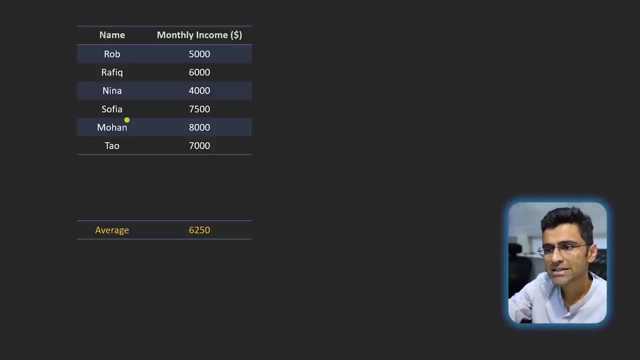 so here I summed all these numbers divided by six. so total number of records are six and that is your average. and average and mean are same thing. okay, so here the mean value is six to five zero and you will realize that this income is not huge enough that people will be of able to afford a luxurious car. so you will not. 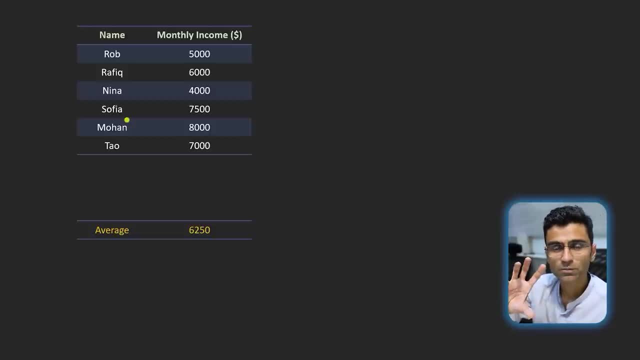 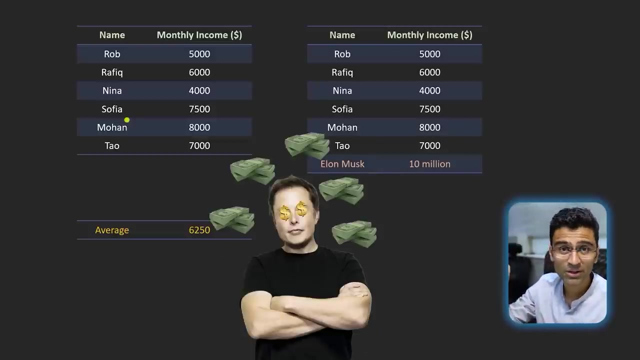 open the showroom. so this is called descriptive analytics. now, what may happen is: in your town there could be one very rich person. let's say Elon Musk is living in your town. let's say he's your neighbor. well, he earns freaking 10 million dollar a month, actually. he. 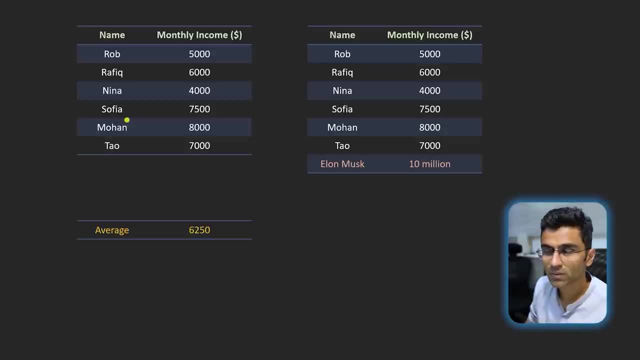 earns probably more, but just giving the example. in that case, whenever you have extreme values like this, the average will not represent the true picture because due to the presence of extreme values known as outliers- by the way, here, elon musk is an outlier- because other people's income levels are. 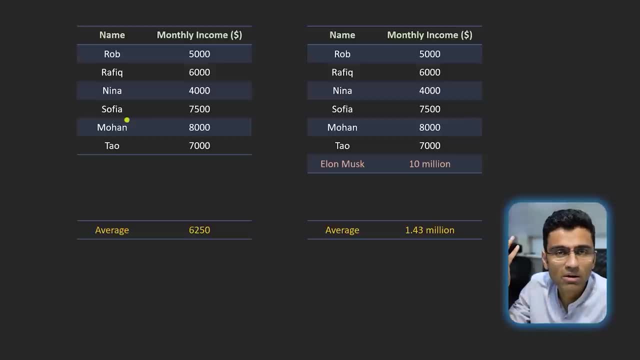 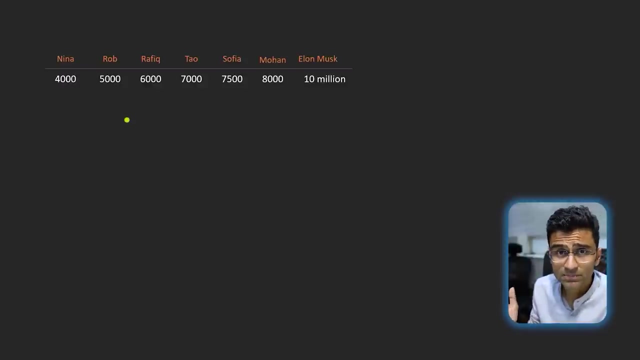 five thousand, six thousand, maximum eight thousand. this guy is earning ten million dollar. it's like too high. so whenever you have extreme data points, uh, using average can be risky. so what do you do then? well, just think about it. uh, one approach you can do is short the numbers. okay, so from less. 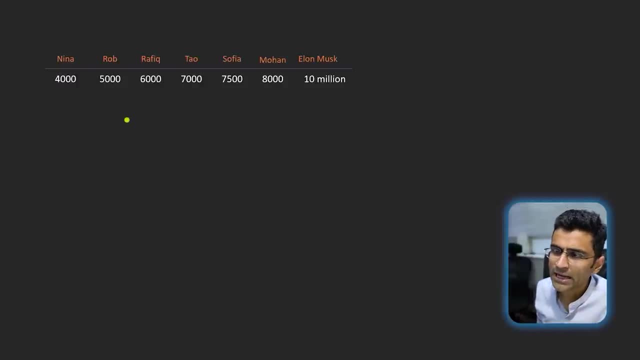 number to more in ascending order and try to take the middle point. so middle point is seven thousand and that middle point is nothing but median folks. so you can use median number or to make your decision. so once again i found seven thousand dollar. it is not a very high income, so i will. 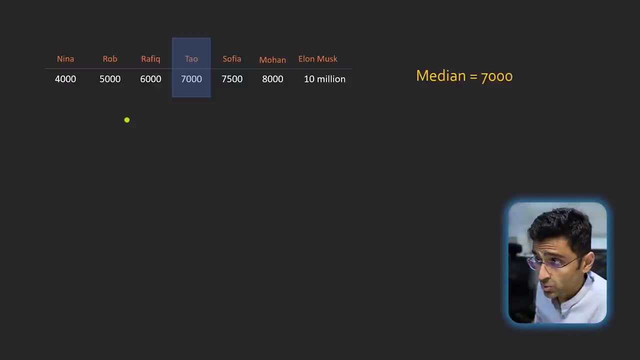 not open my luxurious uh showroom, car showroom, here. the number of data points are odd. that's why middle number is seven. thousand is easy. what if i have even number of data points? i have total eight data points now. well then, also it's easy. so you draw a middle line here, then you take those two values, you 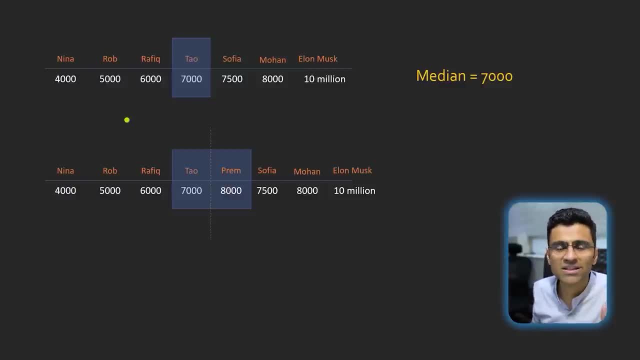 you basically have two values in the middle and you just average it out. so average of seven thousand and eight thousand is seven thousand five hundred and that is your median. so see, median is very easy. if you have odd number of data points, it's a middle number. if you have even number of data points, you 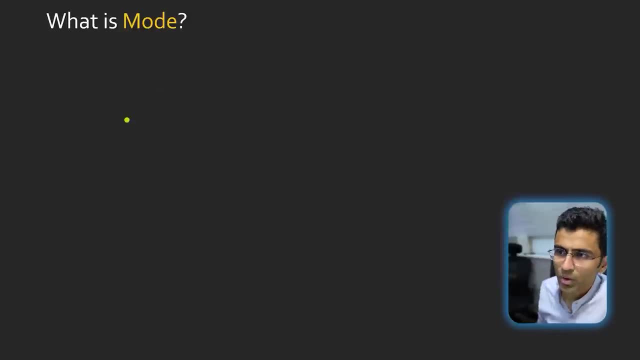 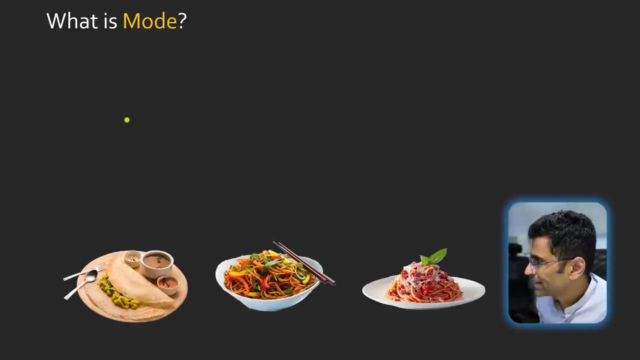 take an average of two middle numbers. now let's look at mode. so what is mode? okay, when you want to go to a restaurant with your friends, what do you do? you will do a survey. you will ask: okay, do you want to eat south indian, do you want to eat chinese, do you want to eat italian? and you take a sort of like: 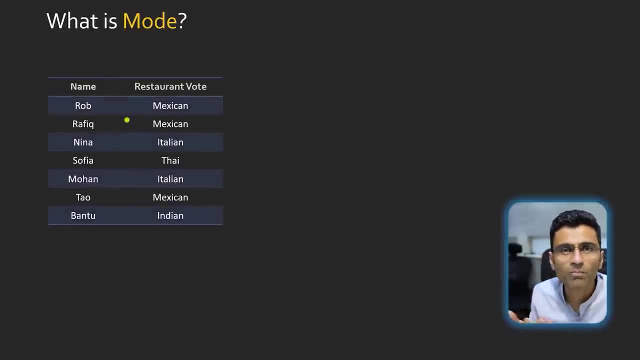 a survey. okay, you ask all your friends where do they want to go? and then whatever is the maximum count, you go with that. so here you have the average of two middle numbers. so that's an average of two middle numbers. see, three people want to go to mexican mexican restaurant. so that will be the decision and that. 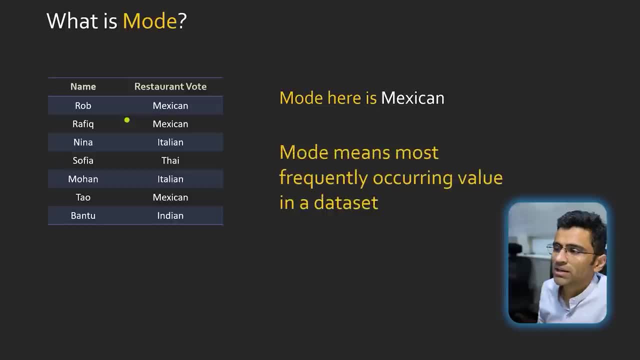 is your mode. mode is nothing but a frequently occurring value in a data set. see more is just a, some kind of jargon. you take any data set and whatever value is occurring most number of times, that is your mode. they use mode in in a way in a voting also right if three candidates are. 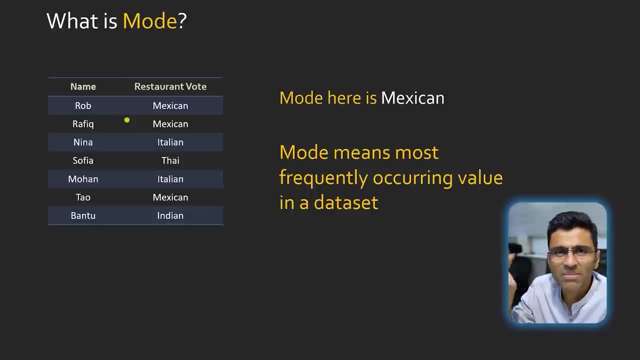 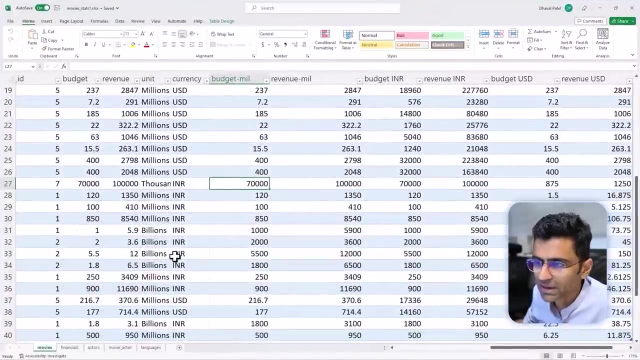 in election, then you do voting. whoever gets the maximum votes, they get elected. so that is your mode. all right, now let's look at our data set and try to use all of this in our excel file. so i have this excel file and i have this imdb. 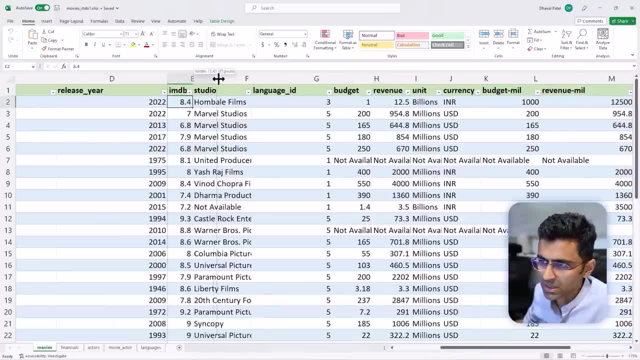 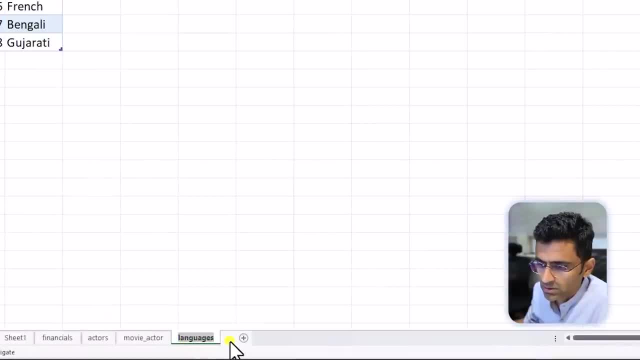 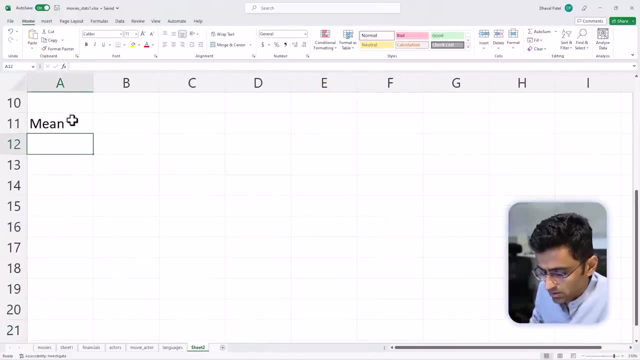 rating, which is the rating of all the movies, and i want to now create a new sheet here. okay, so that's your new sheet. fine, and in this new sheet i can have mean, median and more, and mean for mean the function that you use is average, so you use average. the name of my movies table is movies. 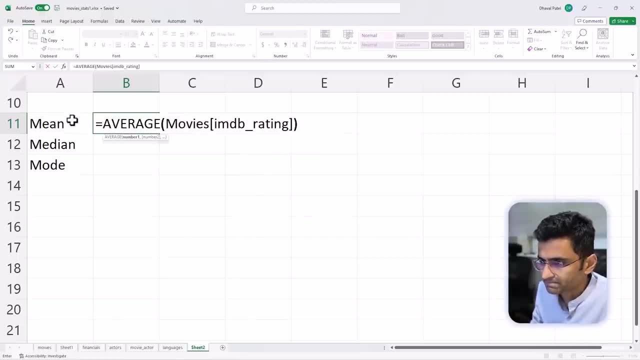 and that imdb rating. so my average imdb rating is 7.94. you can use this percentage here. similarly, median: there is a function: median- once again, movies is my table name and then imdb rating. so my median is 8.1, which means if i take all the ratings and kind of 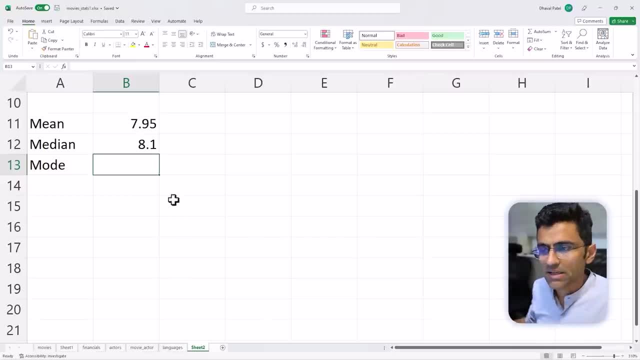 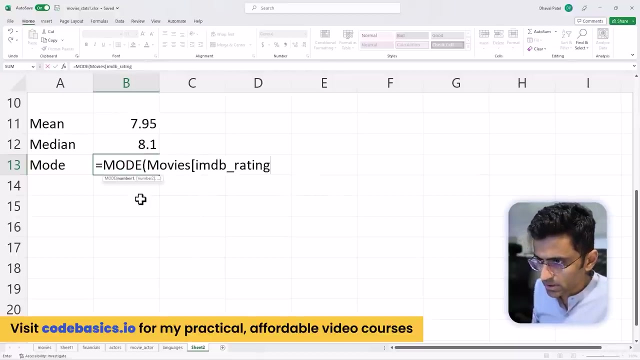 arrange them in a certain way. i can have a rating of 8.1, which means i can have a rating of 8.1 ascending order. in the middle you will find 8.1 and then mod is once again i will do movies: imdb rating. 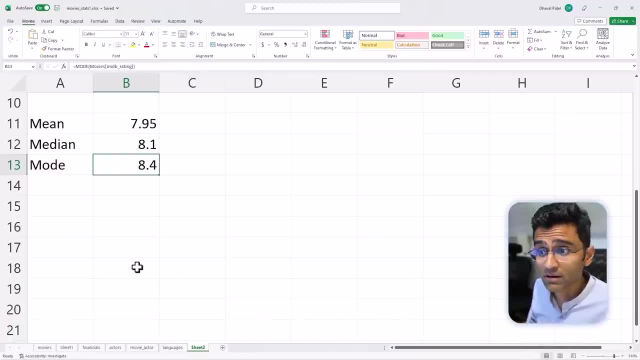 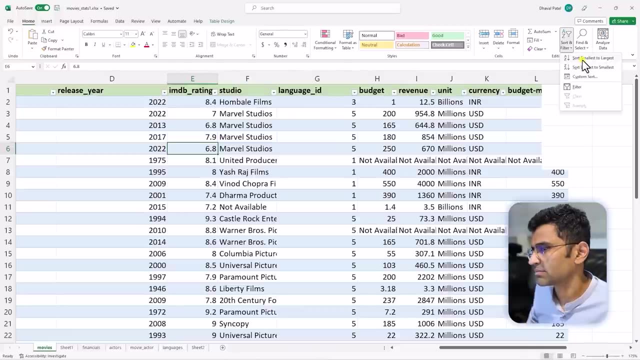 so 8.4 is the most frequently occurring rating. so you can go to movies data set. you click here and you can sort these values. uh, let's say small is two largest. you get all these values and you'll realize 8.4 is appearing four times. 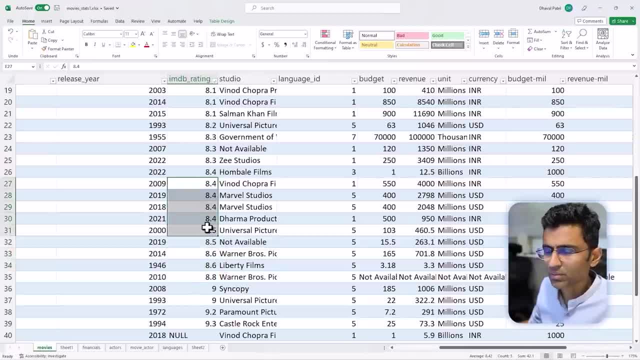 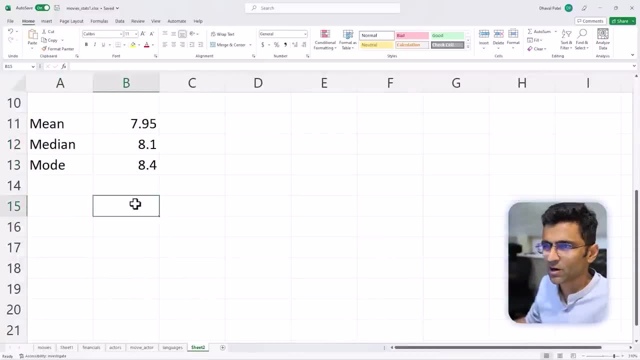 say, 8.5 is two times 8.6. so that is your mode mod, not more mod. okay, so mean median mod. we just cover basic. these are a very, very easy concept, folks, so i hope it is clear in the next video we are going. 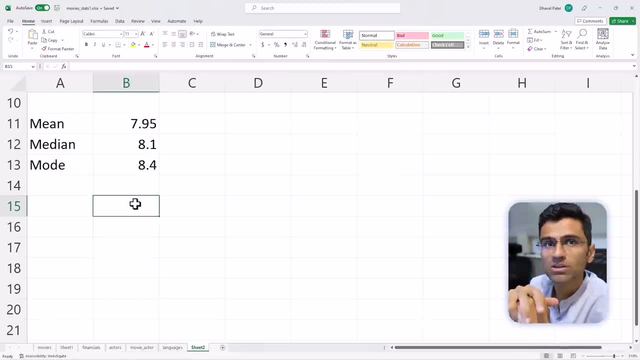 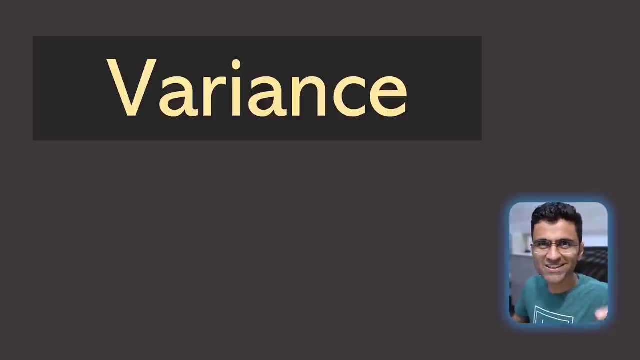 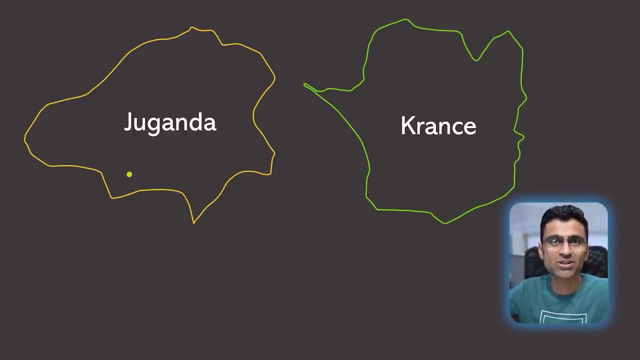 to cover few more uh statistics concepts. in this video we will understand variance and standard deviation using a very simple example. the definition of variance is it measures how far each number is from each other in a given data set. let me give you a simple example of two countries. these are imaginary countries. 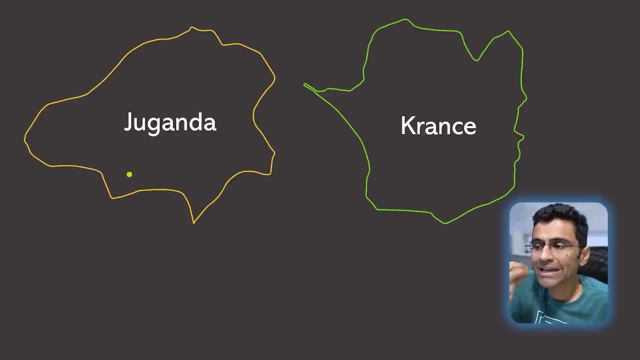 juganda and kranz and you are doing study on the income level of people in these two countries. usually countries have per capita income level, which is an average income of a person in the in a given country, and if that per capita income is higher it means country is economically doing. 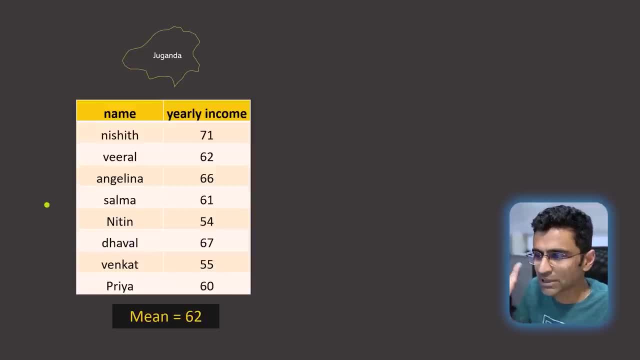 better. now, in these two country, let's say total, eight people live, and when we collected their income level, they were like this, and these are, by the way, thousand US dollars. so Nishit is earning 71,000 US dollar every year, and the average income level in Uganda is 62,000 dollar a year. 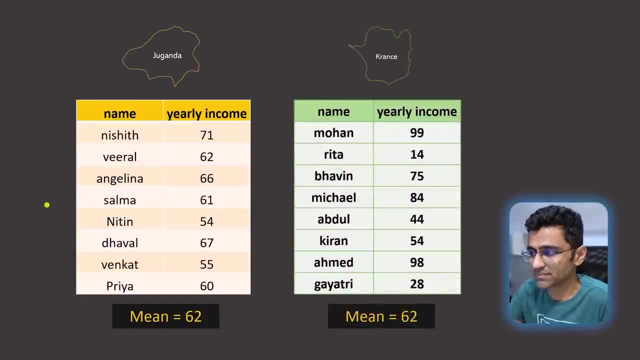 in Kranz. these numbers are these, but the mean is same. so the average income in both the countries is 62,000 dollar. is that an indication that both countries are doing similar in terms of their economic performance? well, if you look at the individual income level, you get a different. 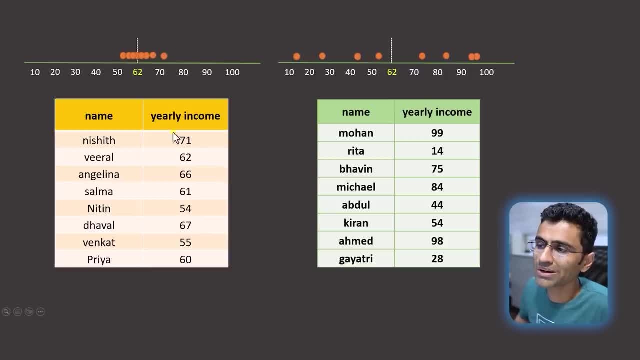 picture here the income levels are more or less the same. so see, 62 is an average and most of the people's income levels are more or less the same. so if you look at the average income level, income are around 62, like plus and minus five or ten thousand dollars, but in Kranz the income 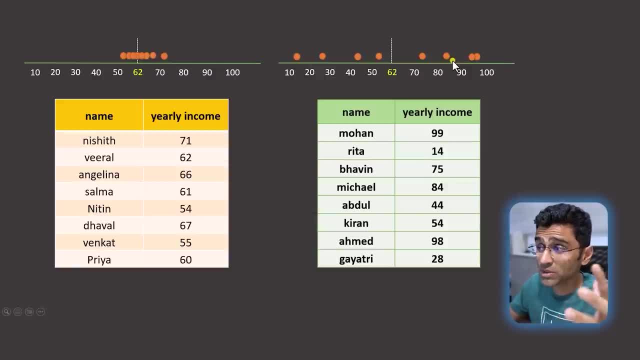 inequality is higher. the data points are very much far apart. so you can say that in Kranz the variance is higher, in Uganda the variance is lower. now you got an idea. okay, variance is higher or lower, but what is it? is it 10, 50, 20? what is it? that has to be some number, so let me show you. 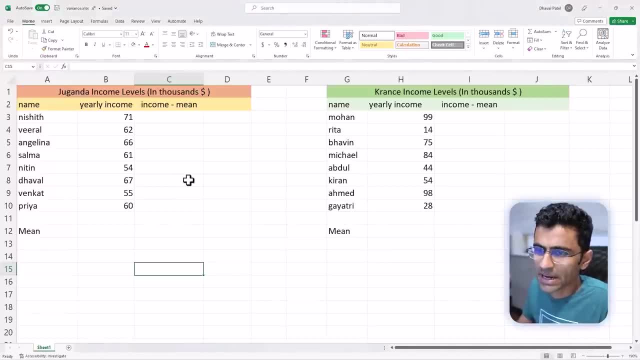 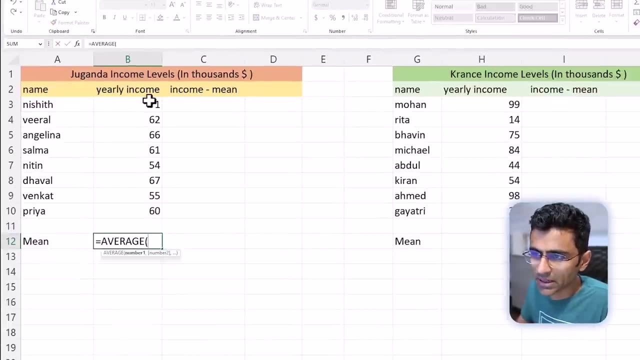 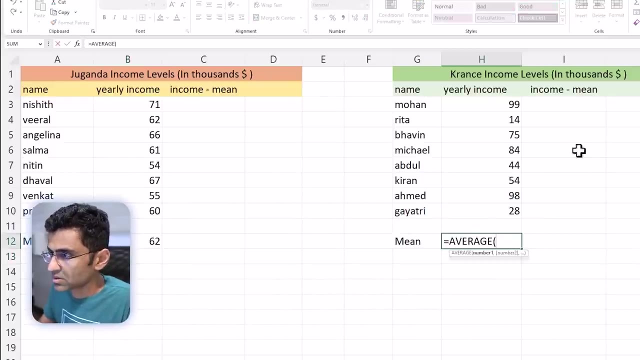 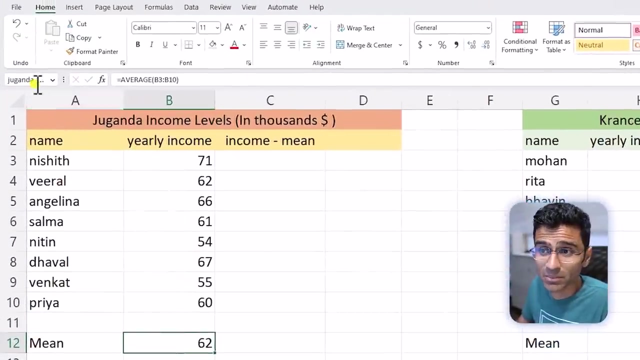 that number using excel. so here I have shown their income level. I will calculate the average income by using the average formula. okay, so that's the average income in Uganda and Kranz. now I will assign this a label number. so see here what I have done is. 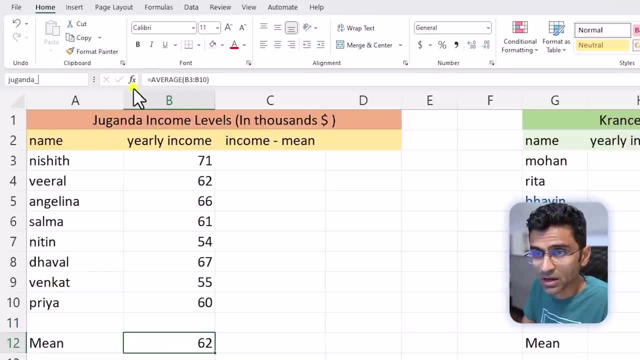 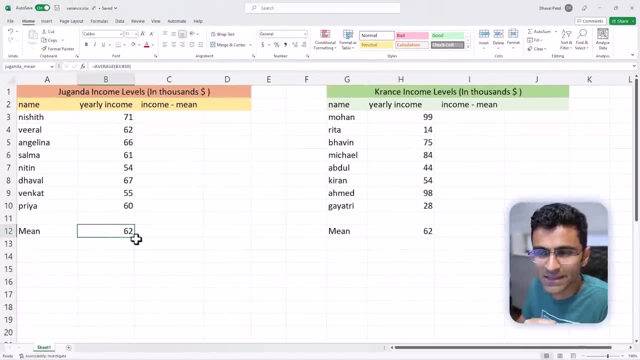 you can say Uganda and Kranz and now I will assign this a label number. so see here what I have done is: you can say Uganda and Kranz, and now I will assign this a label number. so see here what I have done is data mean. what that will do is: let me explain so, but first Kranz means so I have given them. 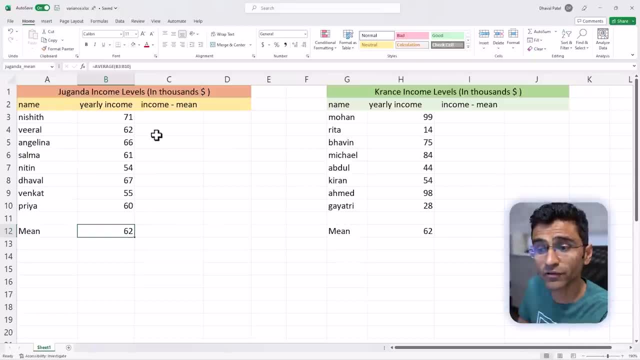 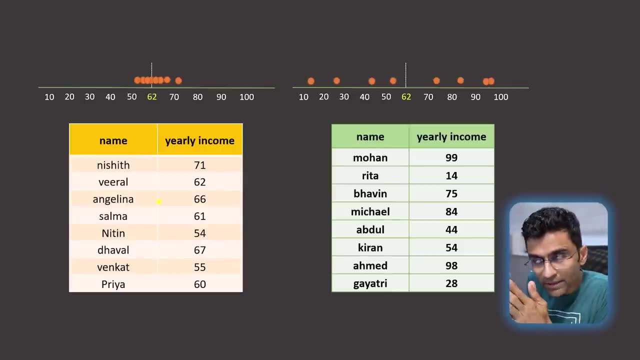 label. okay, and using this label you can refer to that cell. so to calculate how far an income is from each other, you can first measure how far individual's income is from the mean. okay, so let's say there is this data point so you can measure difference between mean and this, so that you can 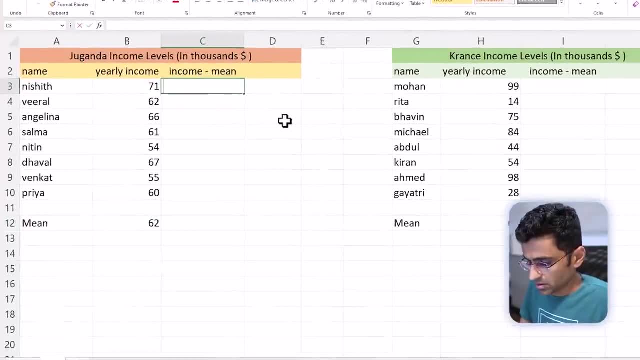 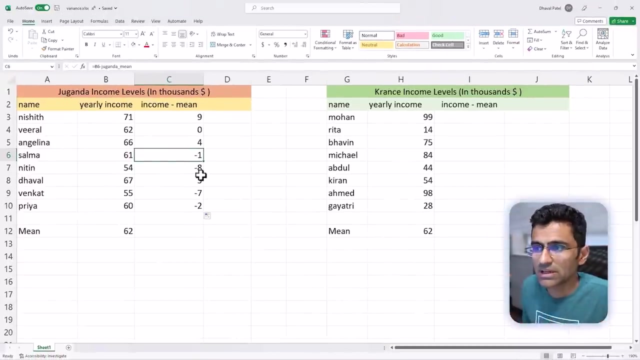 can calculate by saying: okay, individual income minus this mean and this means is Uganda mean. okay, so individual income minus Uganda mean. so that's your difference, and when you do this you get all these differences. now one way of calculating variance that you can think about is: okay, you find out how far they. 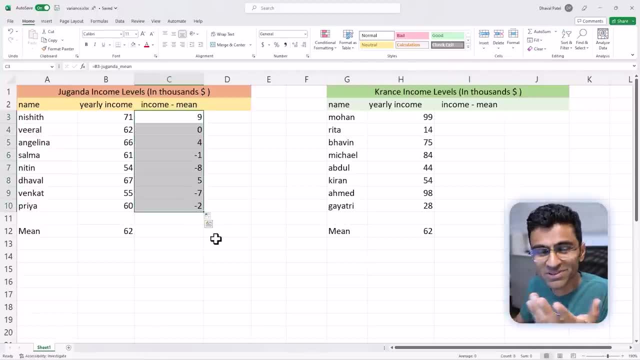 are from mean and then sum them up. but when you sum them up, see you are getting zero. why? because there is negative number and there is positive number. so negative and positive is cancelling out that effect. so to tackle this problem you can maybe take absolute value, so forget the negative sign you. 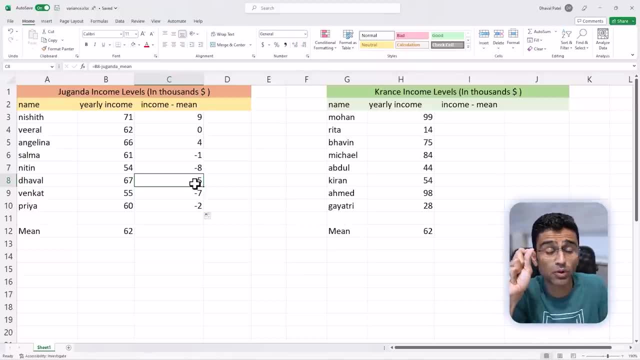 can just take absolute value. but even if you take absolute value, it will have some problems, and I will discuss that problem in a minute or so. but let's just use different approach, which is you can square these numbers. so when you square any number, you get positive number as a result. so you are cancelling. 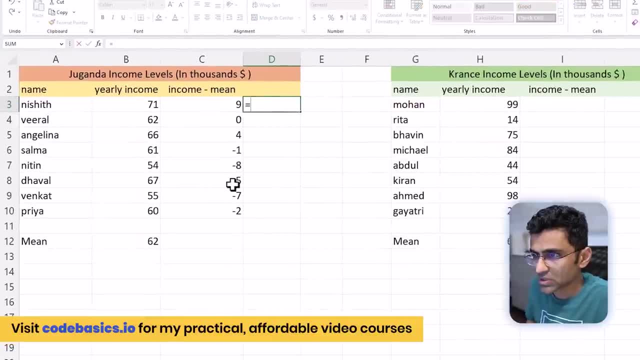 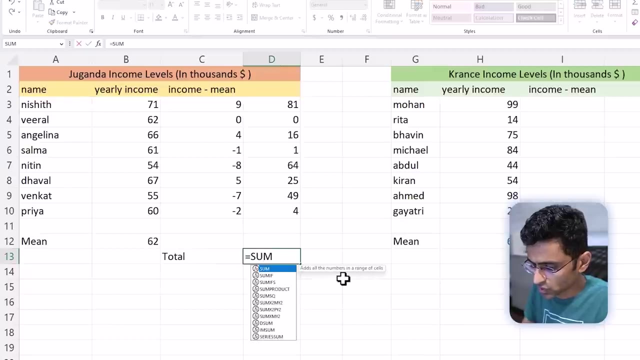 out that negative effect. okay, so I am going to square this number. this is how you square it. so numbers are squared. okay, numbers are squared, and then you can make a total of it. so, total of these squared numbers, is this the count of these numbers? how many numbers? 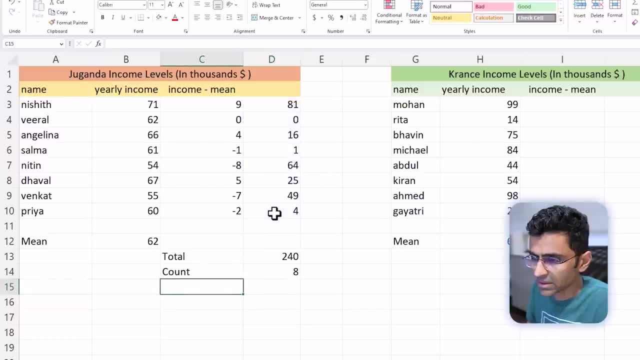 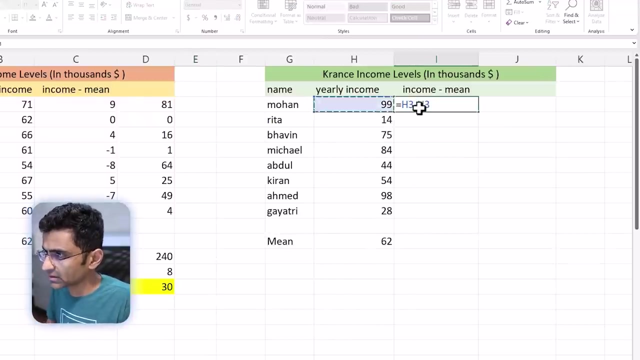 are there total. it is this many, and then when you divide this total by count, you get variance. so this is what variance is. okay, let me highlight. so the variance for Uganda income is 30, and when you do the same thing for this here, okay, canons mean when you do this and then the 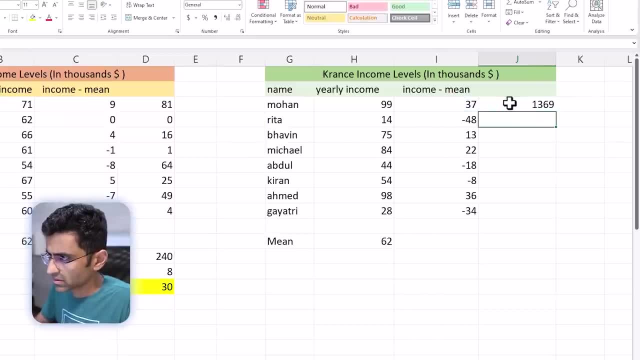 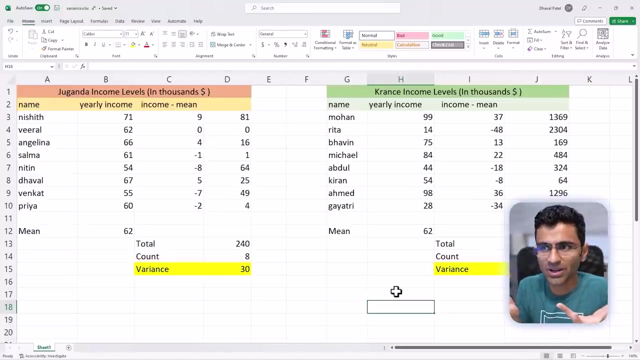 square. I will explain why we do square. okay, so just hold on. and here, when you do total, it is the sum formula you is. count once again this and the variance. look at the variance here, folks. the variance is here is so huge, it is 895. so when you're comparing these two numbers, okay, you get an idea on how far data. 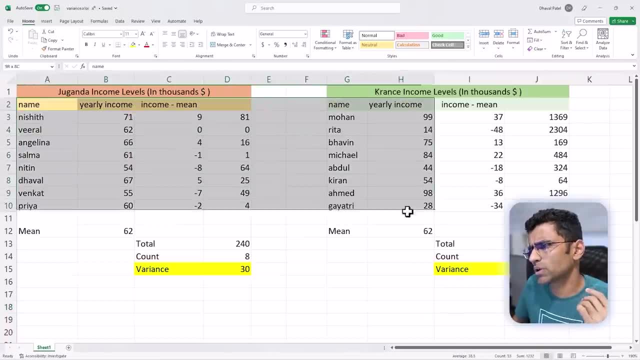 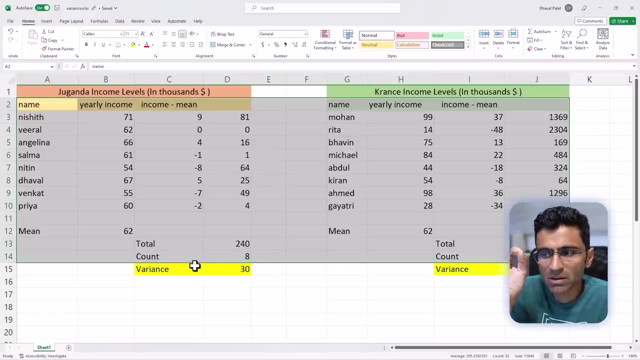 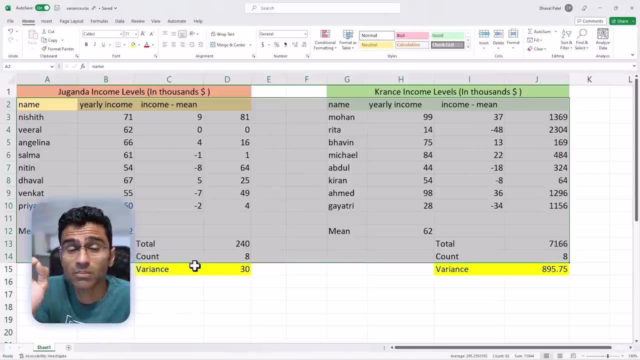 points are so. let's say, someone comes to you and they don't give you all this information. they simply make the statement that in Uganda the average income level is $62,000 but variance is 30, whereas in Kranz, average income level is $62,000 but the variance is 895. just by hearing this, you 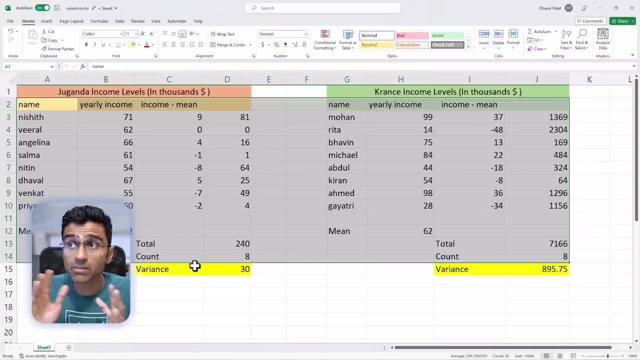 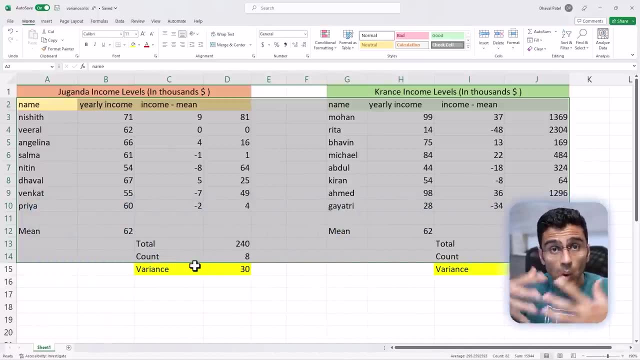 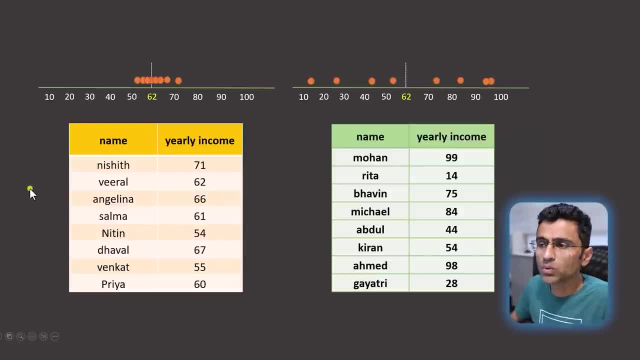 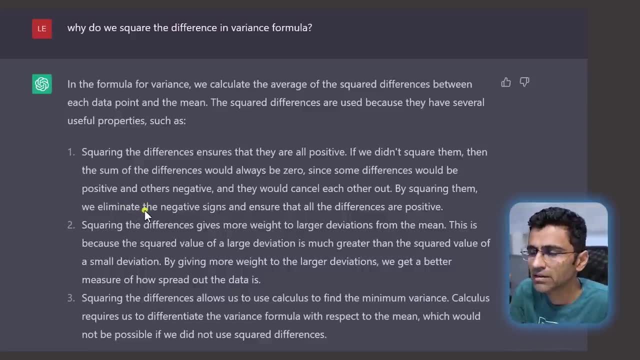 overall data set. so now let me tell you: why do we square it? why don't we just use absolute value? so I asked this question to chat GPT and it said three reasons. number one is obvious: you want to make every number positive. number two is very important: you want to penalize the difference. so 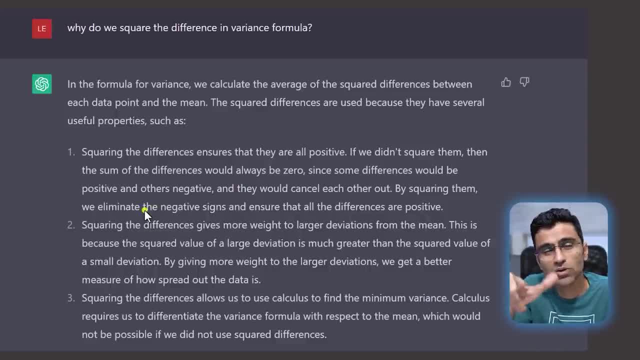 if the difference is higher, you want to penalize it, and the way you can penalize it is by squaring it. so let's say you have a class in your school and let's say you go at nine o'clock, so 9 o'clock is a usual time. 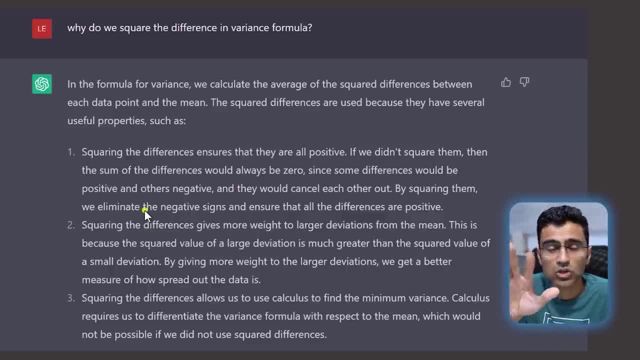 but if you go at 9 and 5 you are 5 minutes late. so then teacher will punish you. they will say: make one round of our football ground. that is a punishment. but if you come at 9- 10 you have to make 5 rounds. so see, as 5-5 minutes increases, your penalty increases substantially. and if you come, 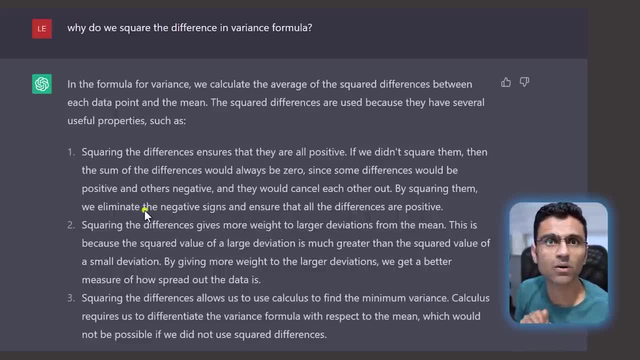 at 9- 15, you have to make 20 rounds. so 9- 5, just one round, 9- 10: 5 rounds and 9- 15, 20 rounds. so as that deviation increases, you want to penalize it and you want to increase the effect. so that way. 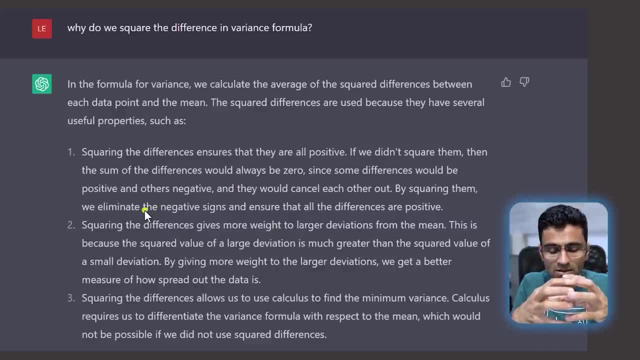 you can get a better understanding of how far or how. what is the spread in data points? um, okay, and the third reason is calculus. so calculus works better with the square numbers? uh, discussing calculus is beyond the scope of this tutorial, but i think at some point in my youtube channel. 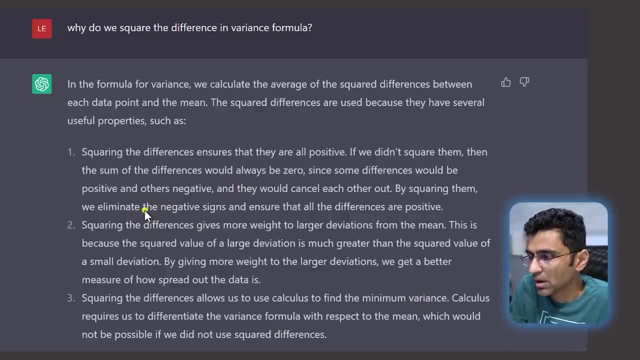 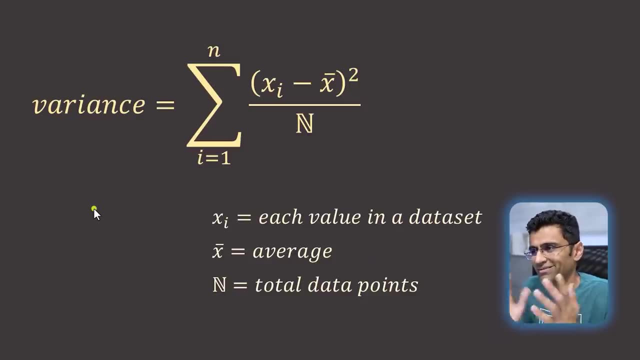 maybe i'll make a separate video on this, but in differential calculus, uh, it will help if you have the square, okay, so that's the formula. and when you look at this formula you know you think, oh my god, this is so complex, but it's not right. see here xi. 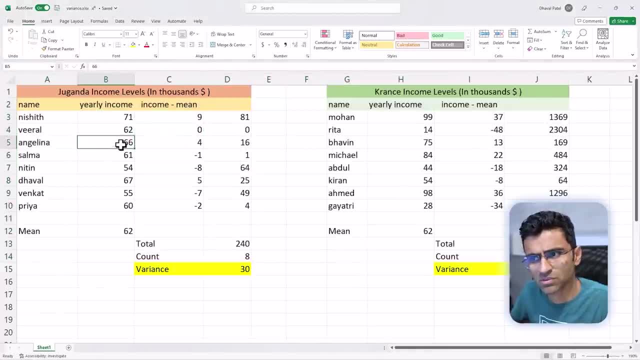 is each data point. each data point is what- 71, 62 extra- you are subtracting mean from that data point. that's what we did. we took the individual data point, subtracted the mean, then we square that number. so this is the square. then we divide it by n, which is c, which is the count, by the way. 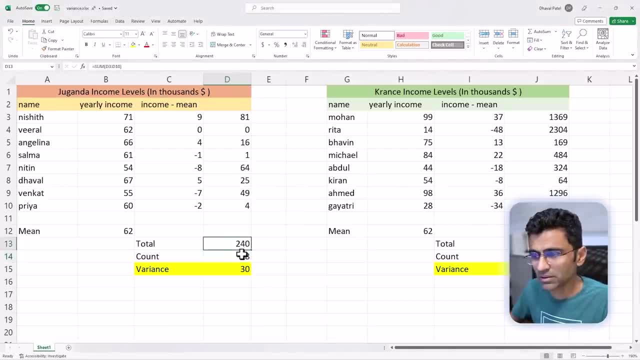 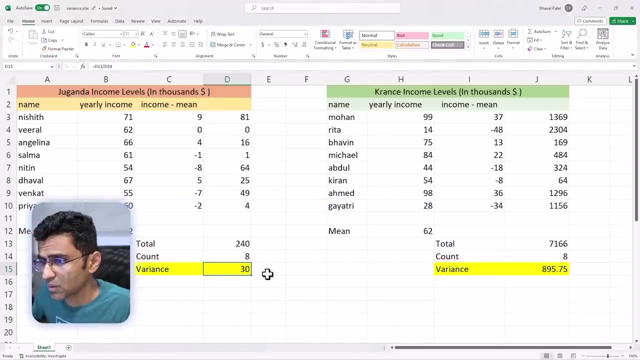 this is the sum. okay, this is the sum. so we summed it, then divided it, and that's when we got the variance. so the formula is clear. now the question is: what does 30 and 895 mean? does it mean 895 000? am i 895 000 apart from the average? no, that's not. 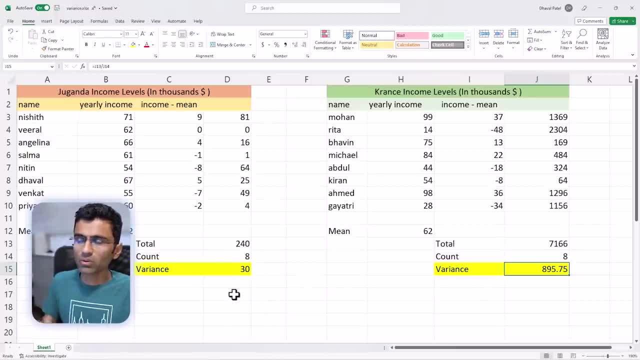 what it means. you square the number. so if you want to make any sense out of it, you have to scale it down. so what is the reverse of square? tell me square root. square root is the reverse of square. so if i do square root of this number, 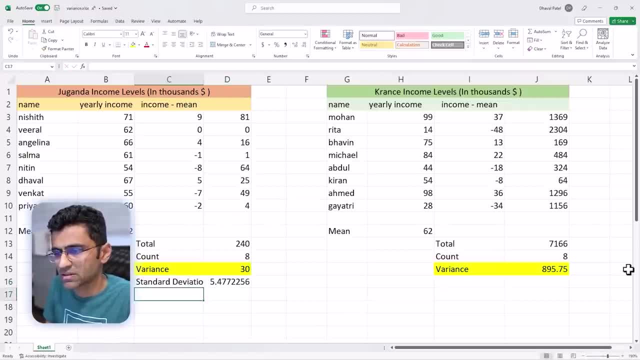 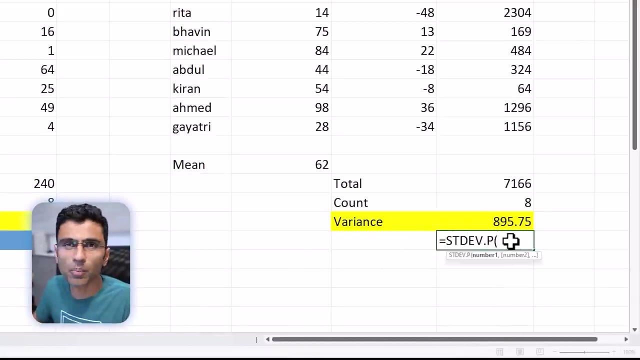 what i get is standard deviation. so standard deviation is nothing but that. okay, so that is my standard deviation. so my standard deviation is 5.5 here. and same way stv dev p by p. it means population, okay, population and mean okay. i can just use a square root. 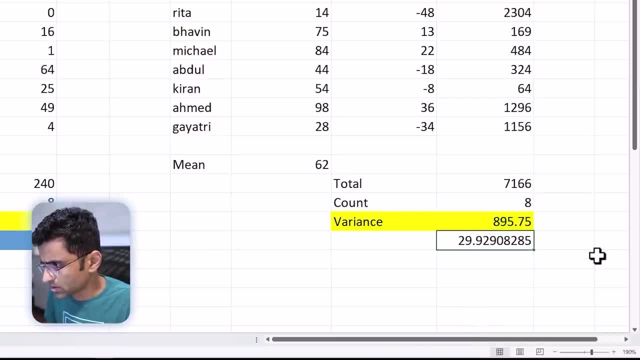 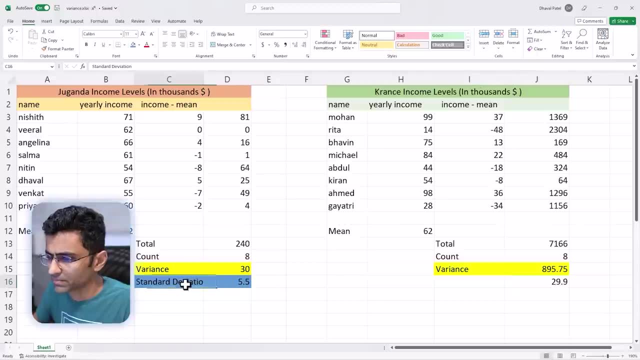 i'll show you the ready-made formula later on. so the standard deviation here is 30, close to 30.. so what this means is: in kranz, on average, person's income is 30 000 plus and minus from the mean, whereas in juganda, person's income is around 5 000 plus and minus, so that you can get. 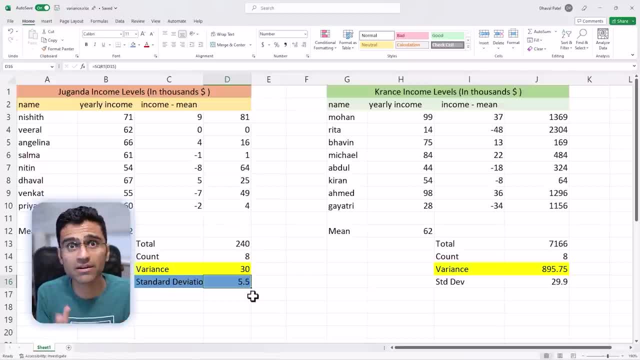 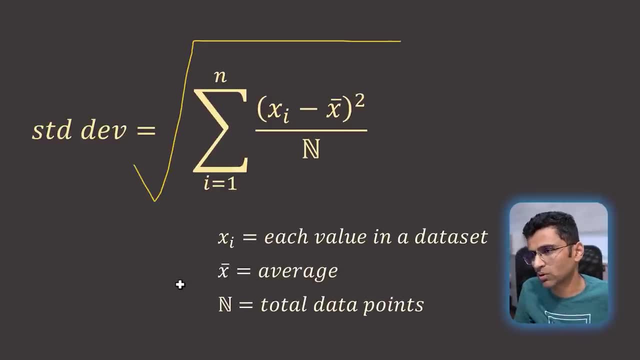 some sense out of it, this number. if you use standard deviation but for variance, it doesn't give you that, that kind of concrete information. so standard deviation is nothing but the square root of variance and there are real life use cases of variance and standard deviation which is stock. 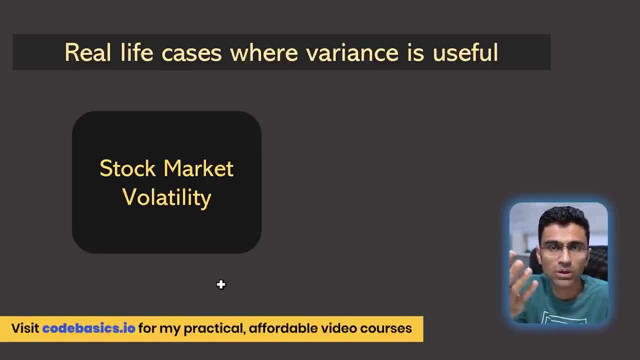 market volatility. let's say you want to invest into stock tata motors and tesla. you want to actually invest in one stock, but you are trying to figure out which stock is better. you take the 1st stock and find out which stock can you invest in next. so let's say you have an average and 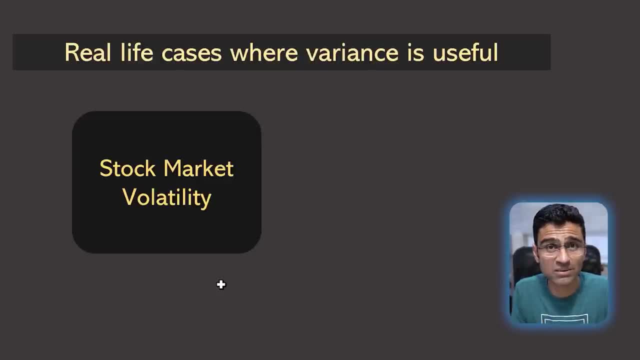 you find out that at the maximum this stock is 100 and you players didn't invest on it because of breaks, so never slowly dollars in the stock, so you can imagine what this stock is going to look like. so now that you know how much it is, you have no idea. 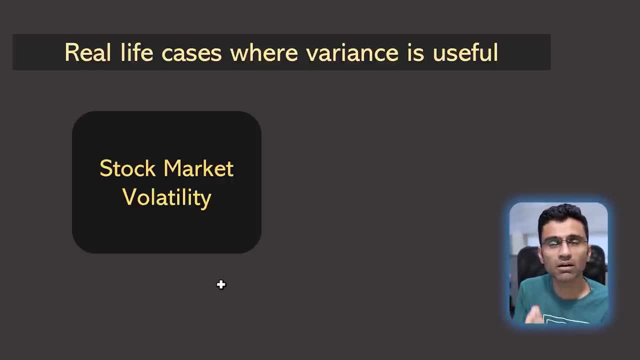 you also know that as thisíamos stronger- 970 or 100 dollar- making you цветed this stock. so you find that both of these stocks were 100 dollar on average, so now they are same. so does it mean i can invest in any stock? 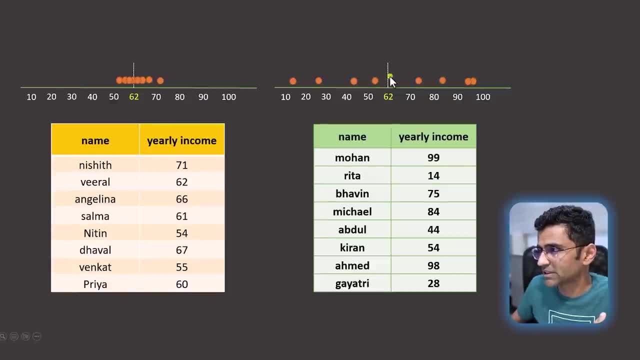 tesla stock. okay, so it is short of like this: see tesla stock. just imagine it's hundred dollar average, but one day it is this much, then. it is this much then. it is this much, this much, this much. so, although average price is same for tesla and tata motors, you want to invest in tata motors? 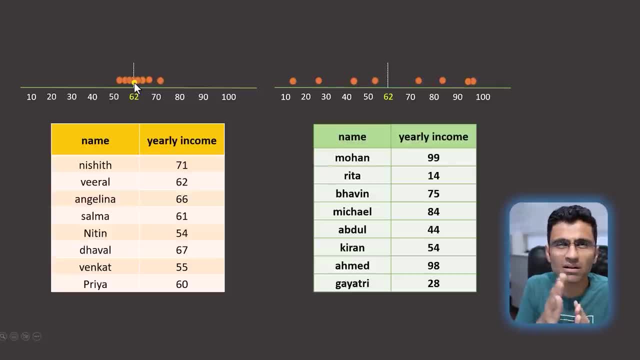 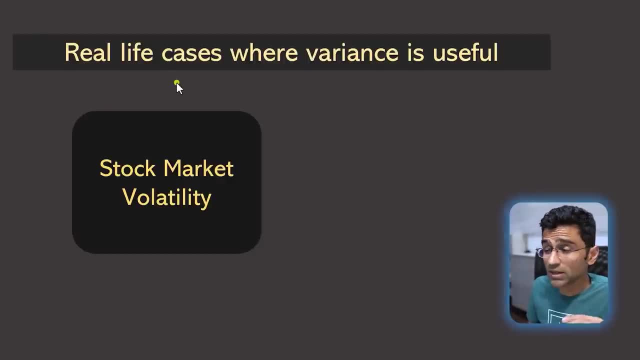 because tata motors might be stable right 100 one day, price is 100, then 100 into 99, 104, etc. so variance is used in stock market. variances also can be used in, let's say, you have a child and you want to admit them to a school. now you have two schools: daily public school and new york. 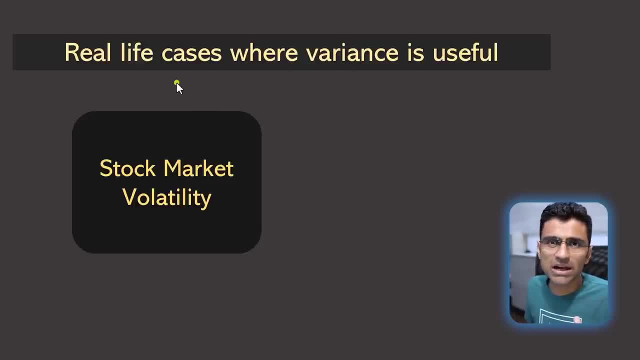 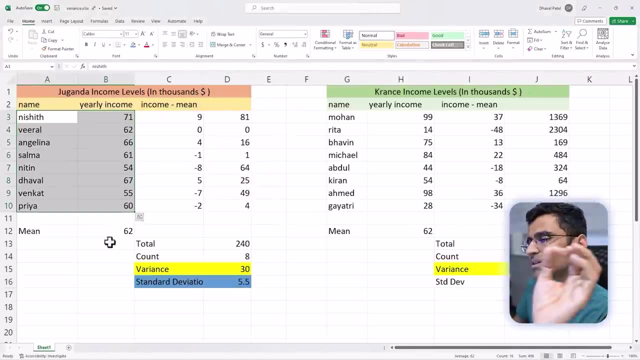 public school, which school i should, um you know, send my child to. well, you can do similar analysis, so just forget. this is income level, right? let's say these are the scores of a student. so let's say you want to admit your student in 10th grade and you look at both the schools. 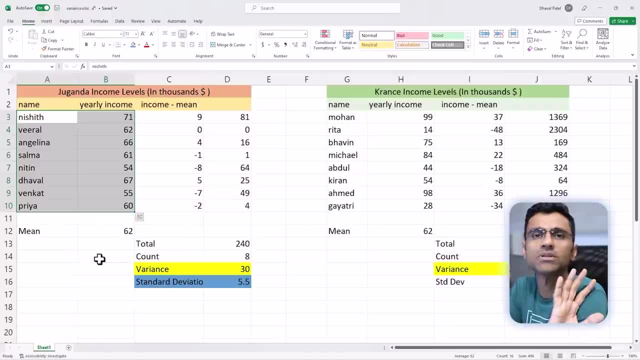 and their current 10th grade student performance, let's say in their current trend grade in a daily public school. let's say: nishit, where are all they are studying? these are their percentage score. their average percentage score is 62 in new york public school. these guys are studying, but 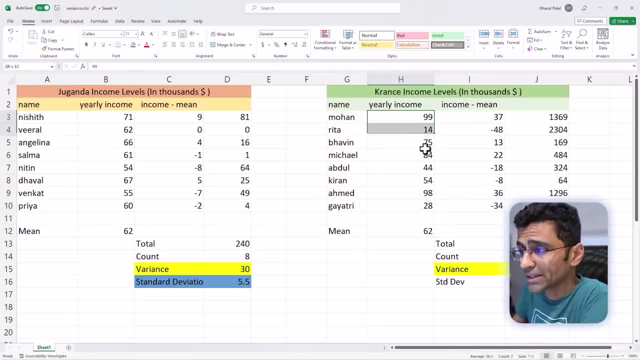 their average score is 62. both are same. but look at their individual scores. it is too volatile, right? let's say mohan and ahmad are getting higher score, maybe because individually they're good. individually they're good, but they're not getting higher score because they're not getting higher. 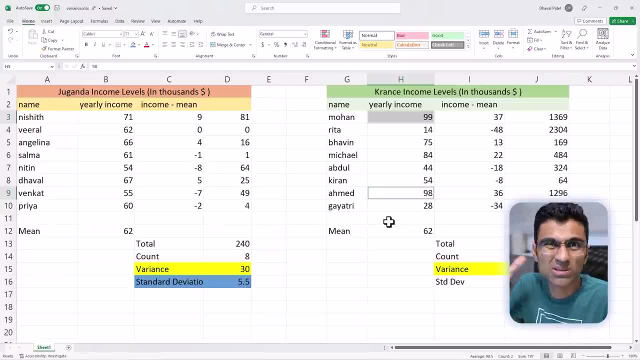 and their parents are taking good care of them. maybe the school is not that great, you know, teachers are not that great, but in this case if everyone is getting good marks, it means students are good. but then there is something that it tells about the teaching quality in that school. so you can make a decision by looking at the variance. so send your kid to a. 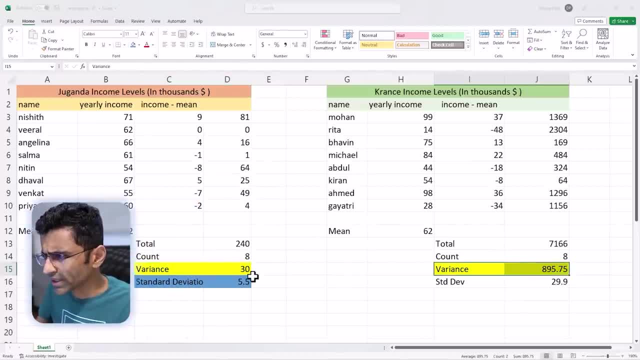 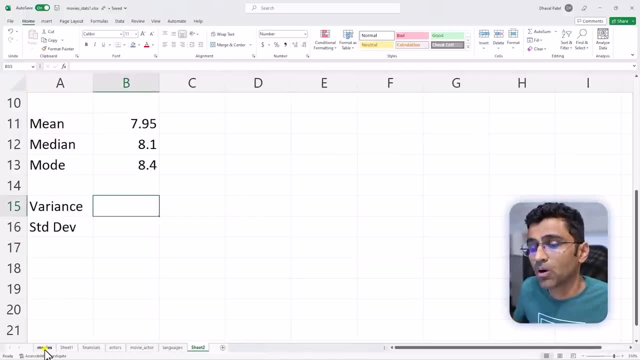 school, which has a low variance. all right. so now in our movies data set we'll quickly calculate variance and standard deviation of imdb rating and we'll use the readymade excel formula. so for variance the formula is var dot p, so there is variance for the entire population, which means 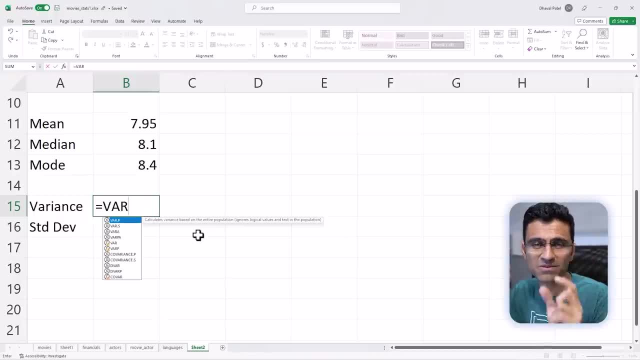 all the data points. there is variance for sample populance, which means only few data points. we are going to use all the data points. so movies imdb rating. so variance is 1.4 and then standard deviation, once again for the entire population, is movies imdb rating. 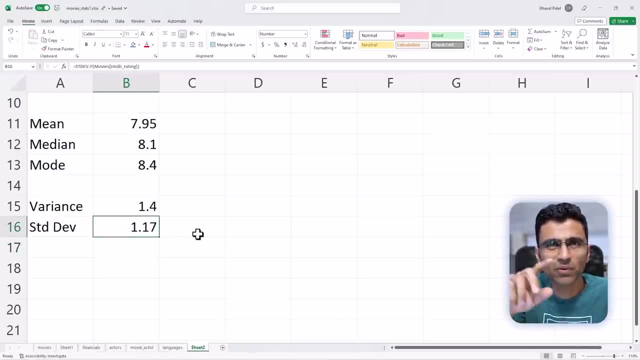 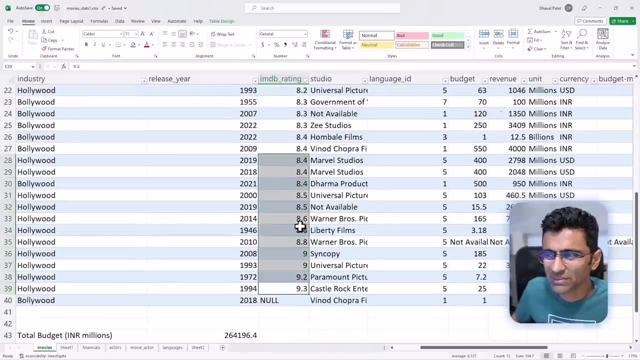 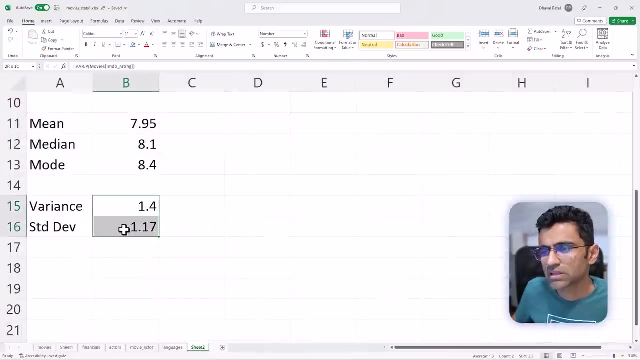 okay, so on average my movie rating is 1.17, plus and minus. you will see from the movies itself you can figure out. see, the ratings are kind of in a similar range between seven to nine. there is just one outlier, but otherwise they are kind of similar. that's why the variance and standard deviation is. 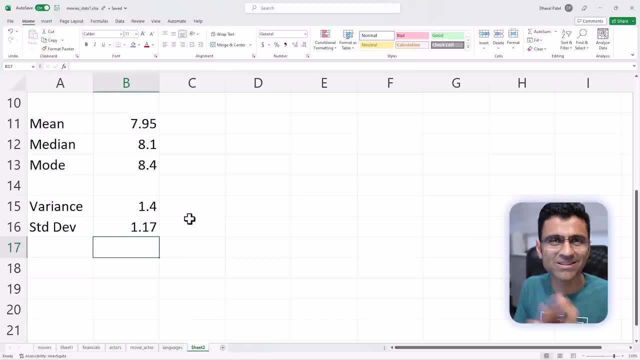 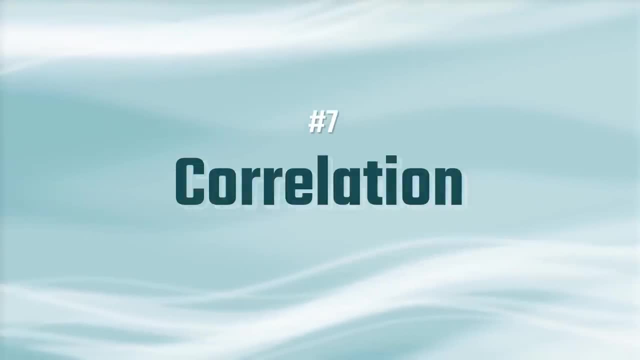 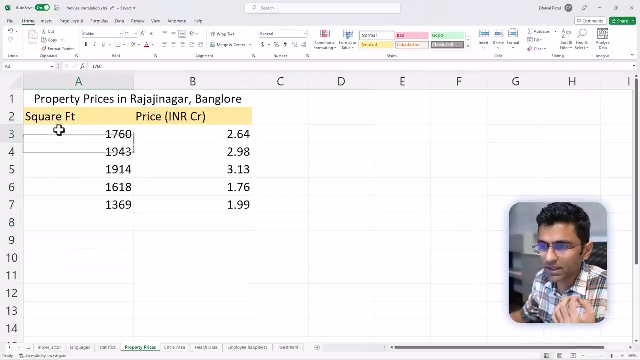 not the same. so all right, that's all we had for this session. i will see you in the next lecture where we will discuss correlation. we will talk about correlation in this video on the screen. i have an excel file where i have shown the square foot of a property and the price. now correlation tells you how related two variables are. 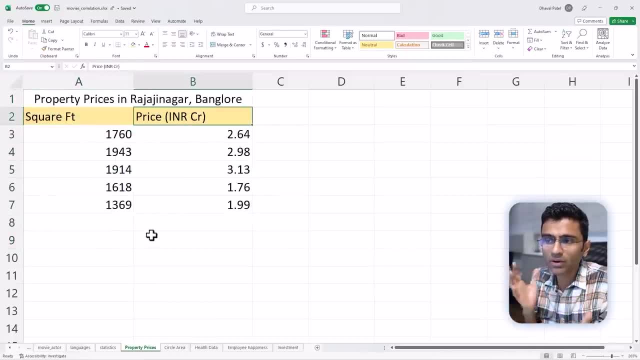 two variables are square fit and price, and you want to know how related they are. now, using common sense, you can say they are closely related because as the square fit increases, the property price will increase. but let's approve this statistically using correlation formula and, by the way, this is: 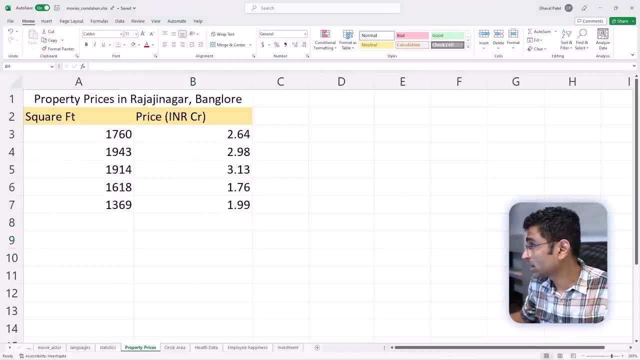 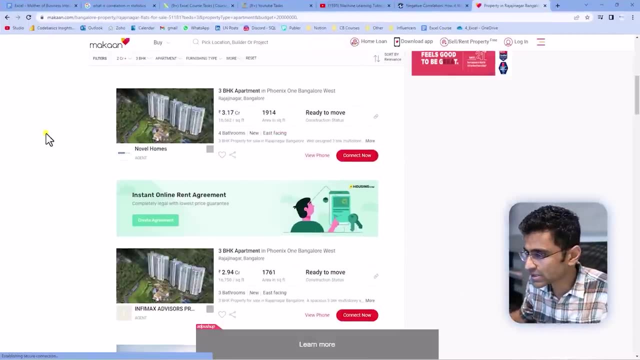 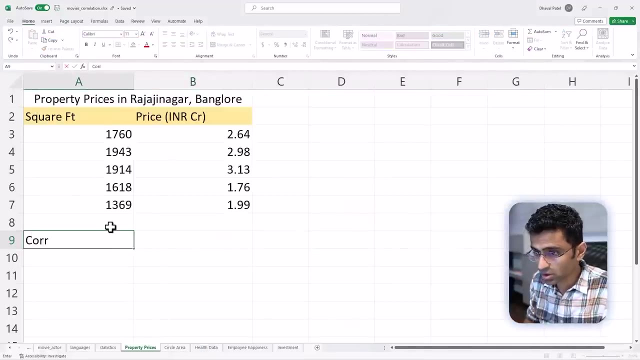 a real data of rajaji nagar area in bangalore that i have received from this makancom website, which is a property website similar to zillow in us, and i got few data points here and that's what i have here and i'm going to now plot a correlation here and the formula you can use. 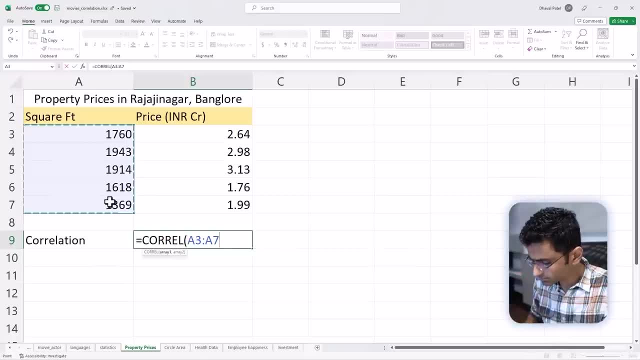 is correl, where you specify both of your data point arrays and it tells you there is a 86% correlation. if the correlation is one, it means they are very closely related. so the correlation is one. it means they are very closely related. so the correlation is one. it means 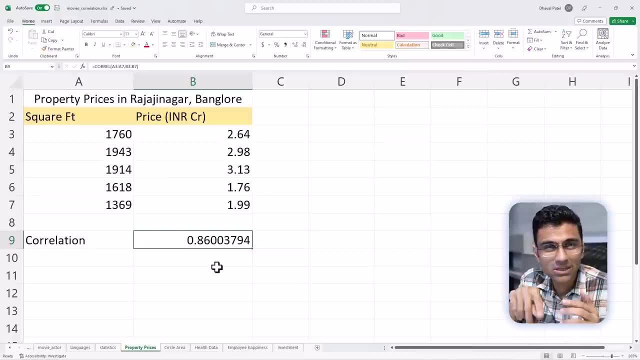 the range is, i think, negative. one to one. zero means they are not related at all and negative one means they are negatively related. we will look at negative correlation in detail, but here it clearly shows 0.86, which is very close to one, which means these two variables square, fit and price, are. 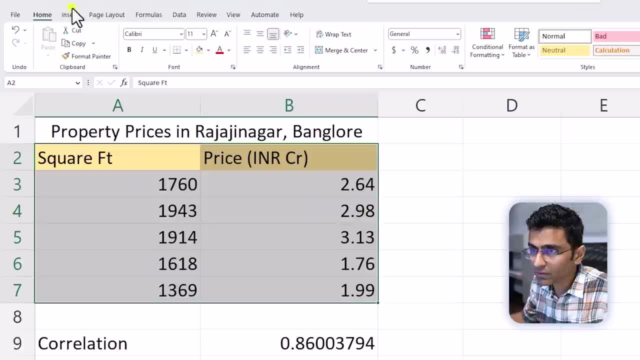 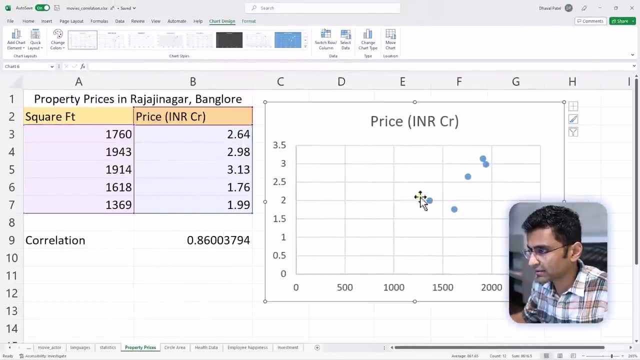 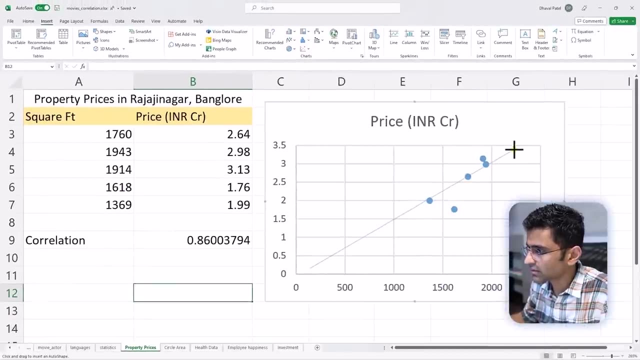 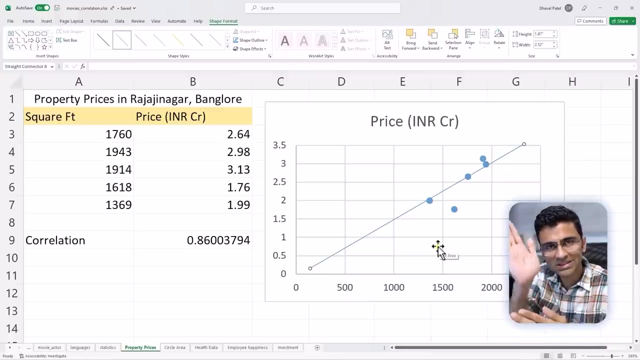 very much related and if you plot a scatter plot by going into insert- click in this, you will find that they are correlated using a linear equation. so if you insert a straight line here, see, it will look something like this where the data points are mostly around that straight line. so if there, 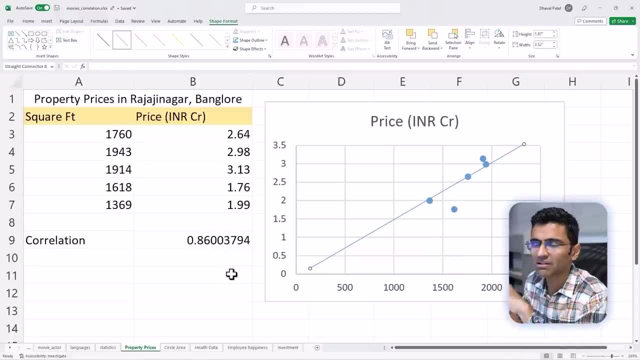 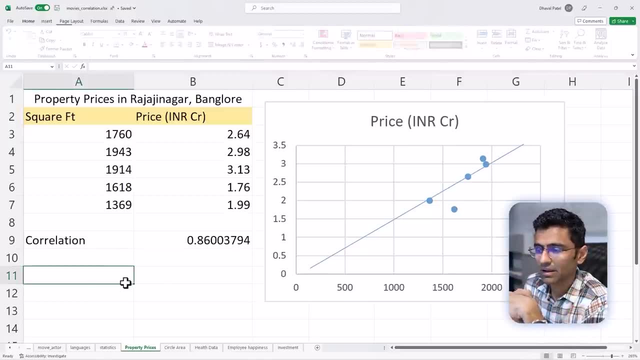 is a line and the data points are around that it means they are related. so on the x-axis we have the square foot, y-axis, we have the price, and this shows positive correlation, where positive correlation means if one variable increases, the other variable increases as well in the same direction, and if one variable decreases, of course the other variable decreases. 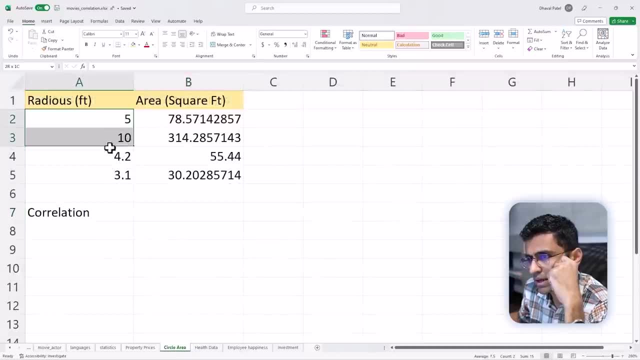 let's talk about circle area, where i have the radius of a circle and you know the formula of the circle's area, which is pi, r square. so pi is 22 by 7 into r square, meaning phi into phi. okay, now tell me what will be the correlation between radius and area if you use common sense. 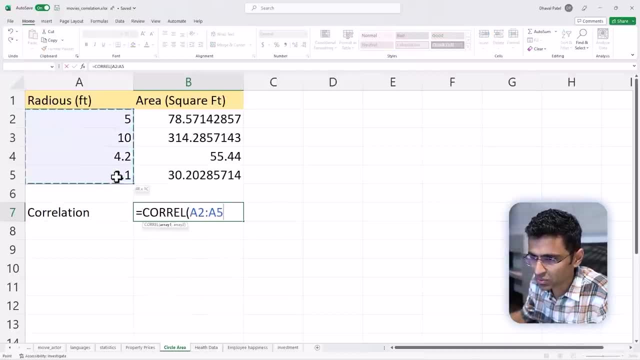 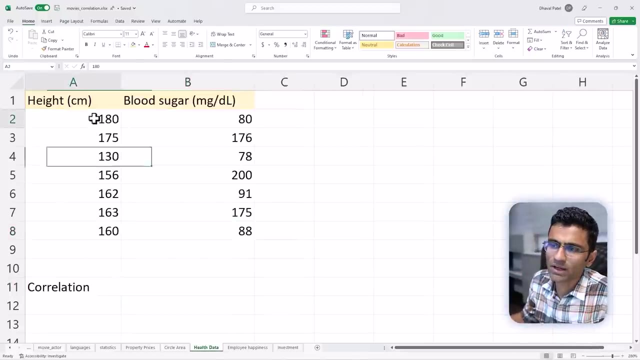 it is pretty straightforward, okay, so let's show this. so correlation between this comma, this close to one, isn't it a common sense? as the circle of the radius increases, the area will increase as well. let's look at health data now, where i have people's height in centimeter and 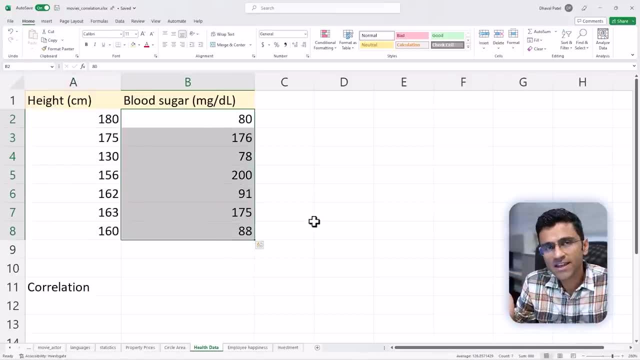 their fasting blood sugar level. now tell me, is there any correlation between people's height and their sugar level, whether they will have diabetes or not? is it dependent on height? no, correct height and the diabetes health level has no relation, almost no relation. there could be some relation. i don't know, i'm not a doctor. 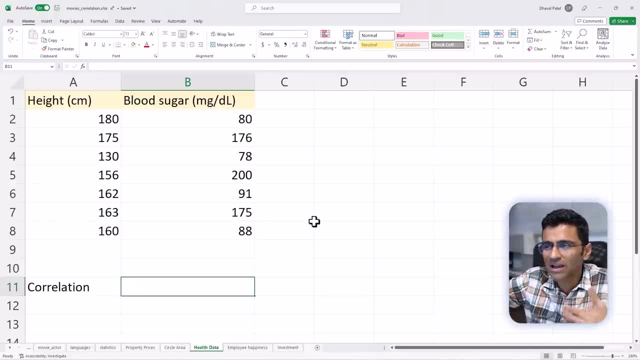 but the common sense says no. i mean, if you're getting diabetes or not, it is dependent on your genetics, your eating habits, your exercise, etc. so let's see, so i'm gonna use correlation here between this comma, this and you find, is this point two? there'll. 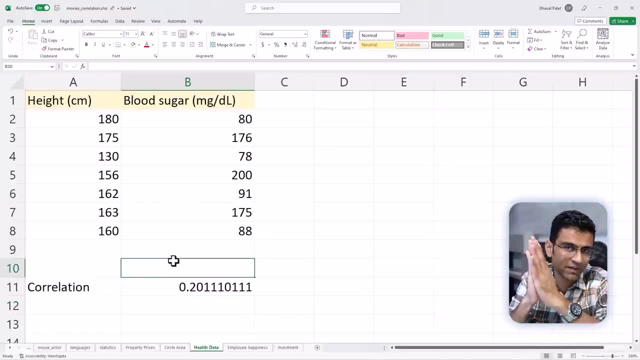 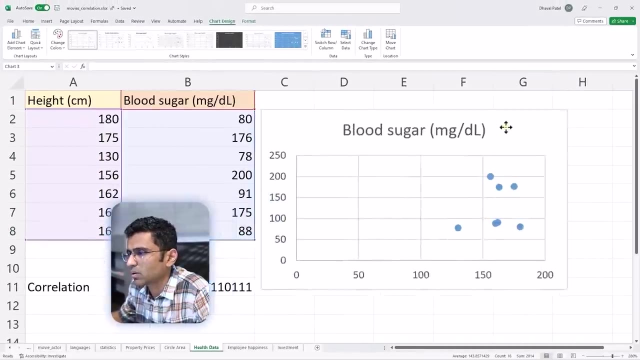 be some correlation, obviously, but see, it's very like, like far away from one, and it is close to, closer to zero, which means these two variables are not related. and if you plot a scatter plot of the same thing here, you will find that data points are all over the place. see, there is no like linear. 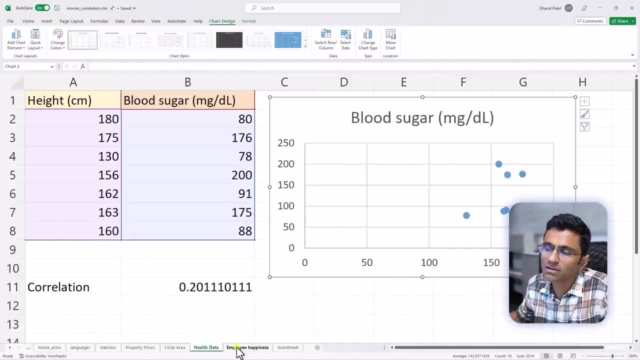 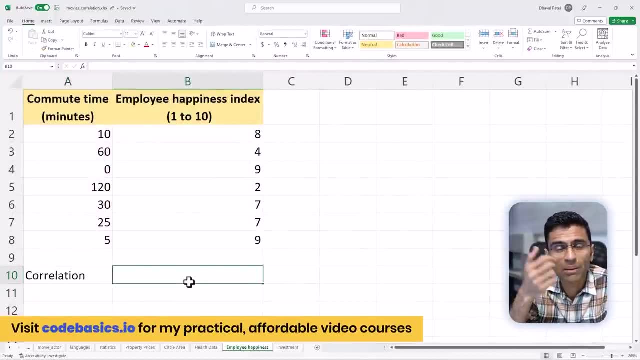 correlation that you can draw from here. the other example i want to use is employee happiness. now tell me what is the correlation between commute time and the employee happiness? the common sense says that if the person is commuting longer hours, let's say this person is commuting two hour one. 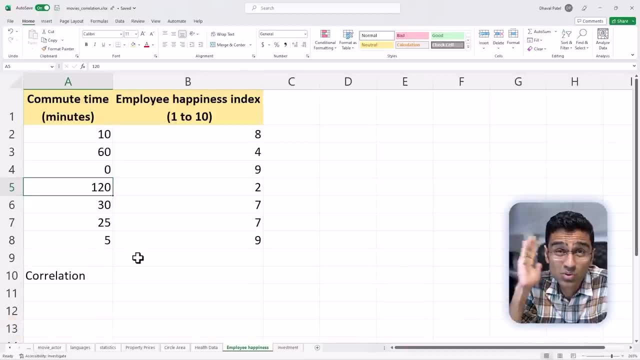 way 120 minutes is two hour. one way he goes two hours, then he works and then he comes back two hours again. he or she, their happiness index is low. so if the person is commuting longer hours this is out of ten. so two out of ten means employee is not happy. the happiness as such. 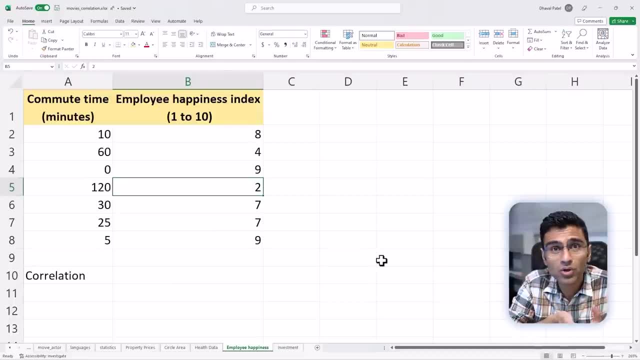 depends on other factors as well, such as salary, what kind of work you are doing, you know, your relationship with your manager and your colleagues, etc. but just to keep things simple, let's say your happiness depends only on commute. it's very clear, see, this person is having zero commute, which means 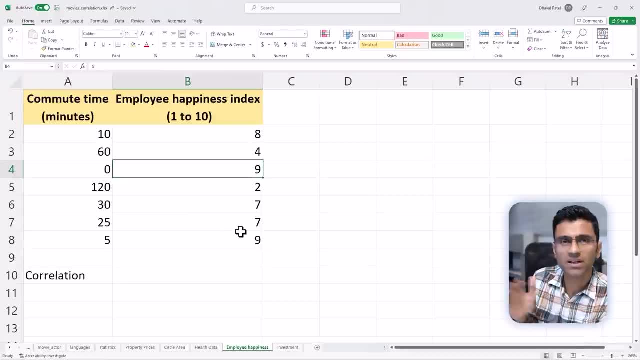 he's working from home and their happiness index is very high. nine out of ten. this person is working 10 minutes. her happiness index is eight out of ten. sixty four out of ten. let's plot a correlation here between the two. do you have any guess? what will be the output? pause the video and make a guess: negative, close to negative one, okay. 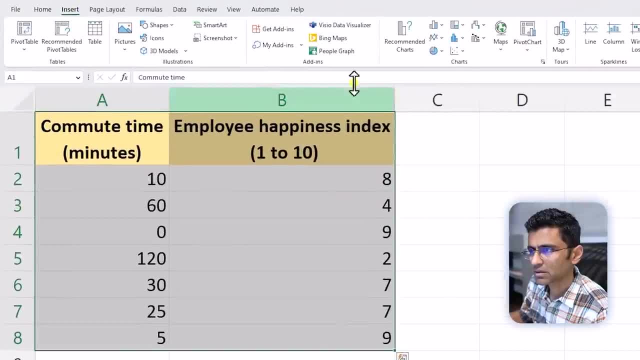 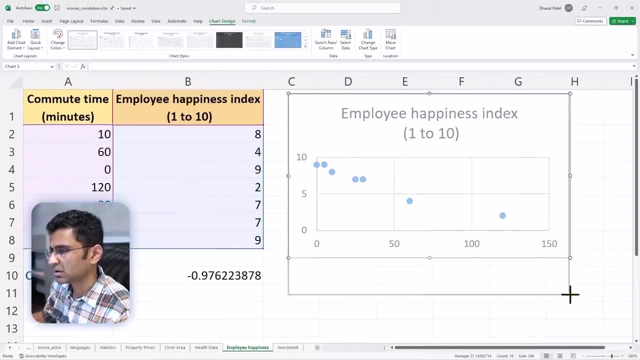 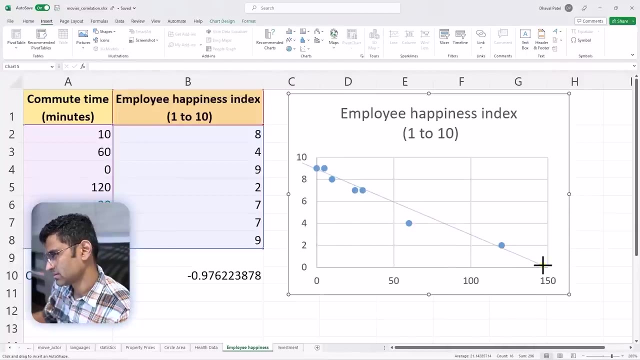 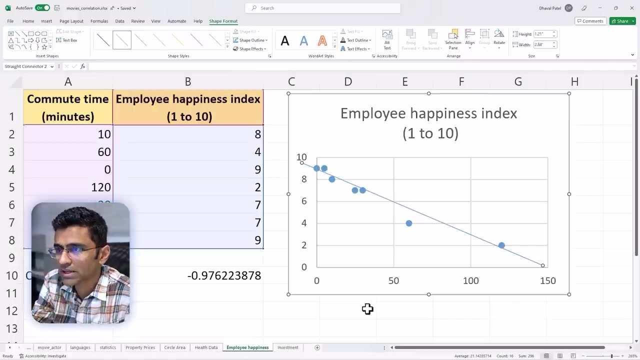 so if you plot this here- yeah, once again i'm gonna plot a scatter plot- see, here you can almost draw a line- straight line, i would say- and that data points are around that line only. so that means, uh, there is a correlation, but it's a negative correlation. and then there are types of correlations such as: